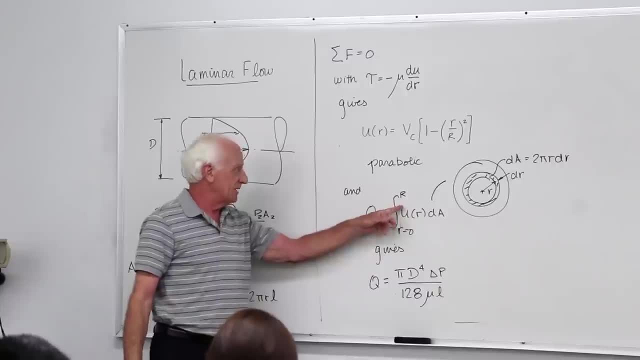 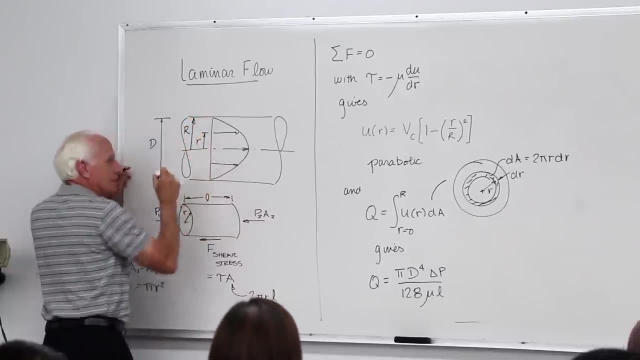 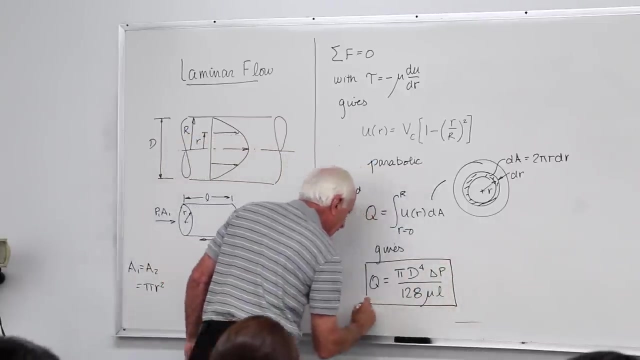 that from the center line, R equals 0, out to the outside radius. Here's the picture. The outside radius goes to here, capital R. Okay, When you do that, you end up with this equation. Okay, This is this equation. 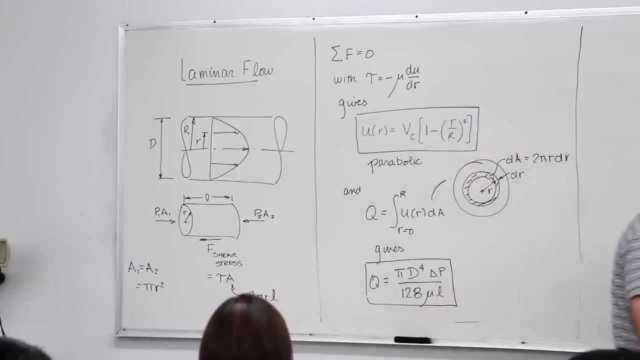 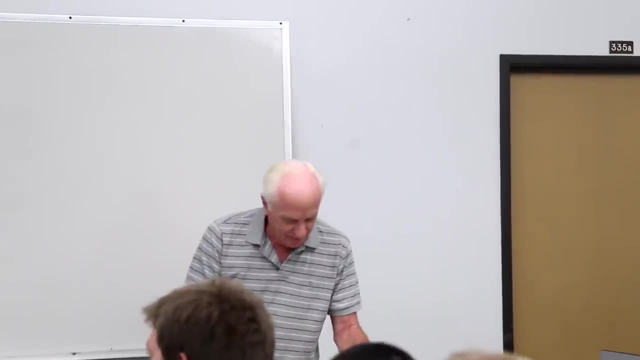 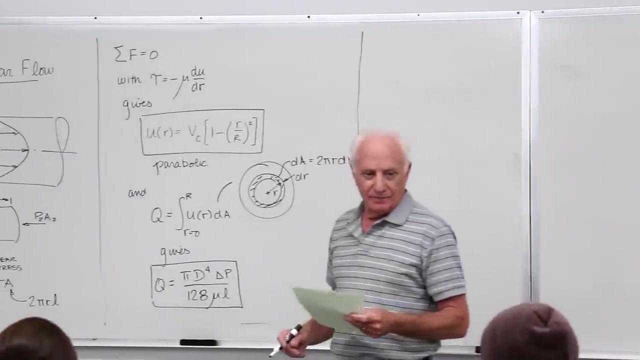 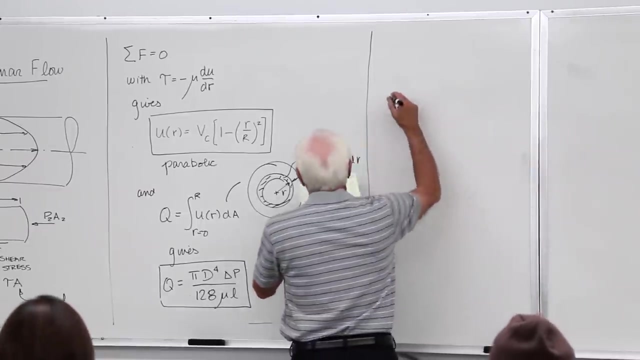 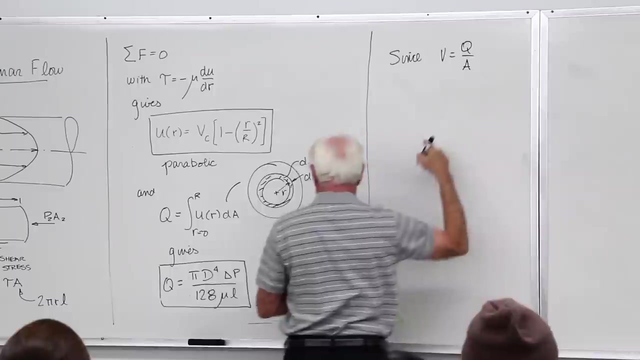 Okay, I think that's about where we left off last time. Now the next step: Yeah, I think we did this two less times. Did we get VC equal to V two less times? Yeah, okay. So what we said last time was: since V equal Q over A, we put that Q up there, divide it. 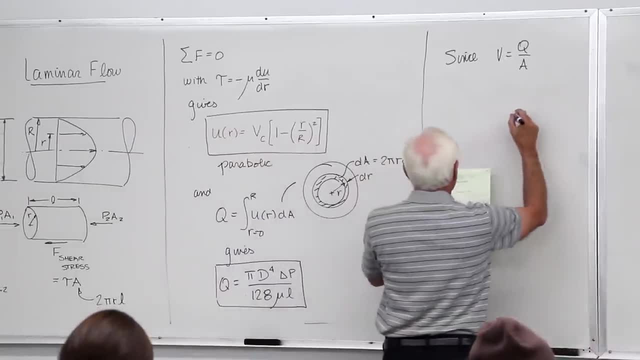 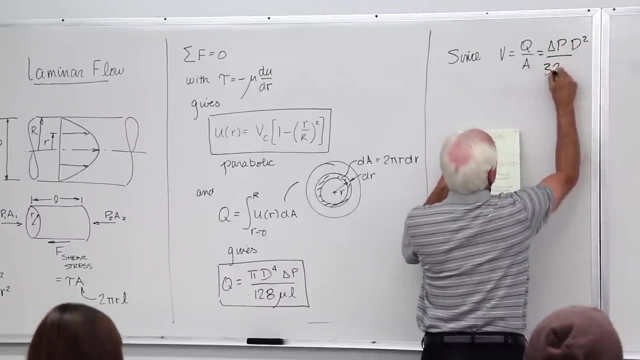 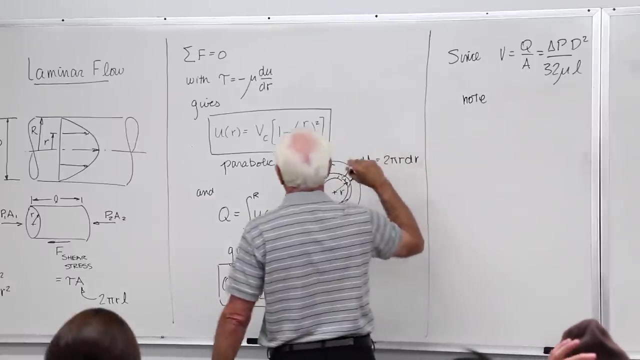 by the area pi big R squared, and we get the average velocity, delta PD, squared over 32 mu L. And then we note, when we did this last time too, we compared that to VC- that the average velocity is delta PD squared over 32 mu L. And then we note, when we did this: last time too, we compared that to VC- that the average velocity is delta PD squared over 32 mu L. And then we note- when we did this last time too, we compared that to VC- that the average velocity was just VC over 2.. 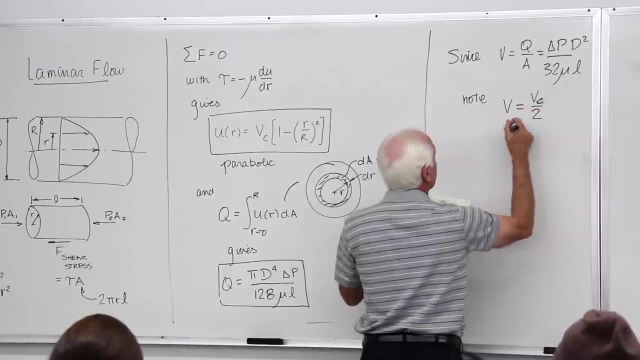 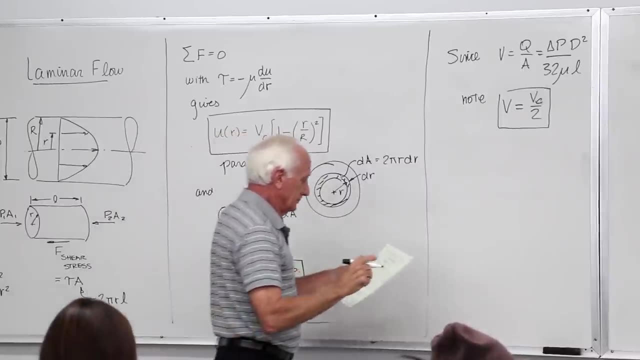 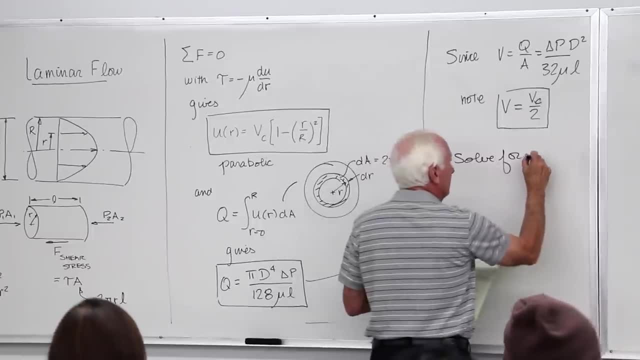 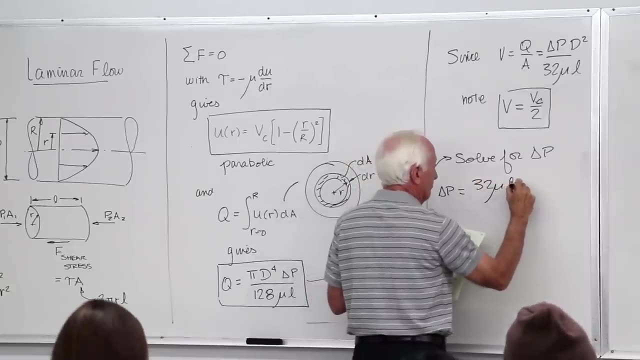 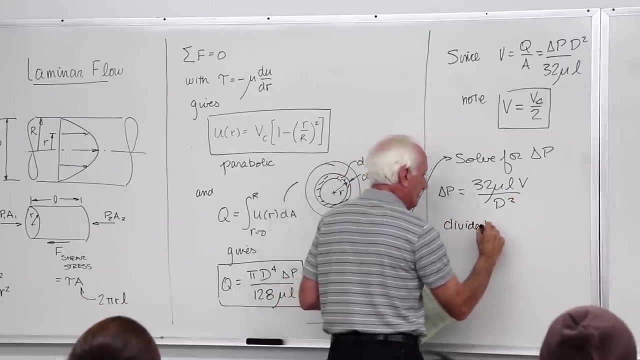 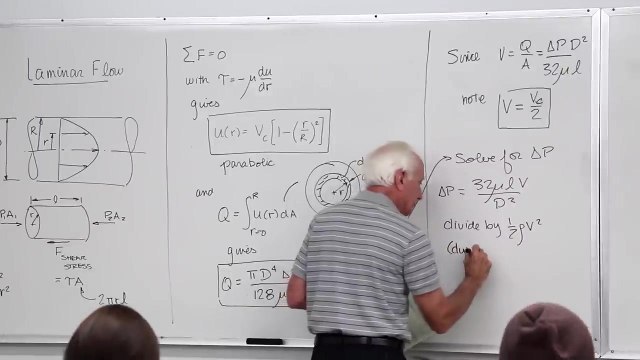 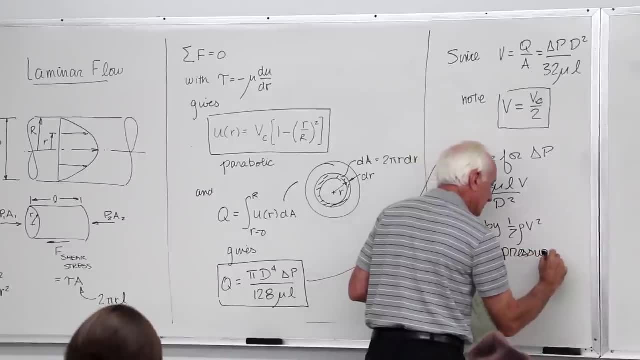 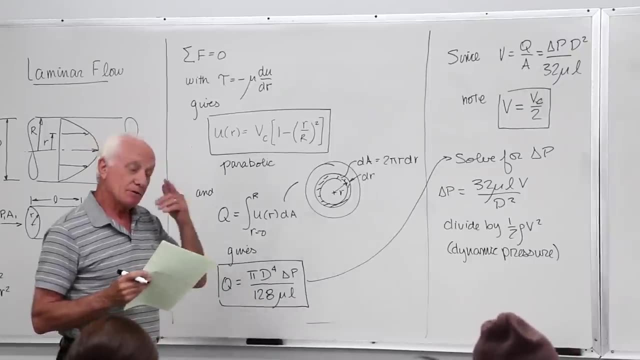 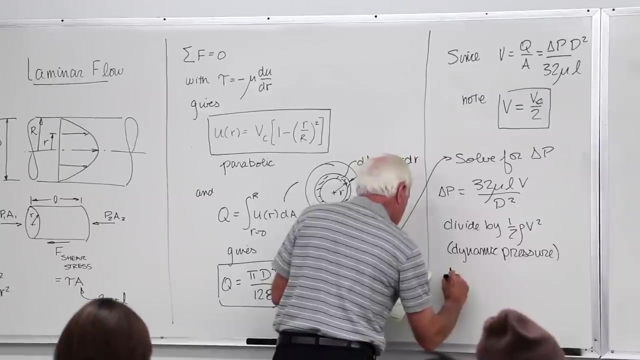 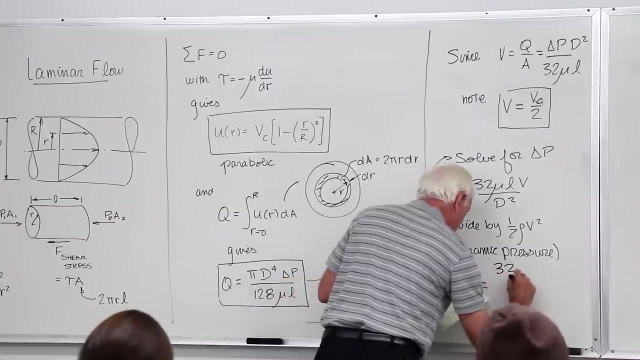 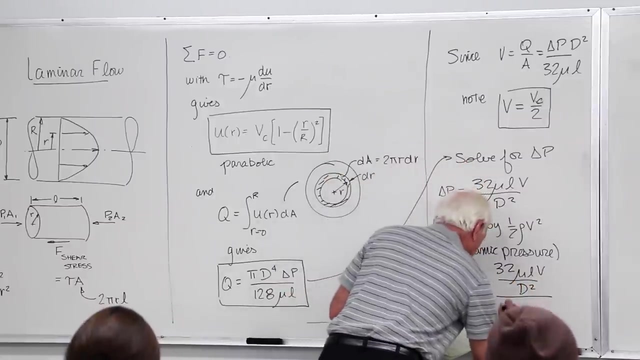 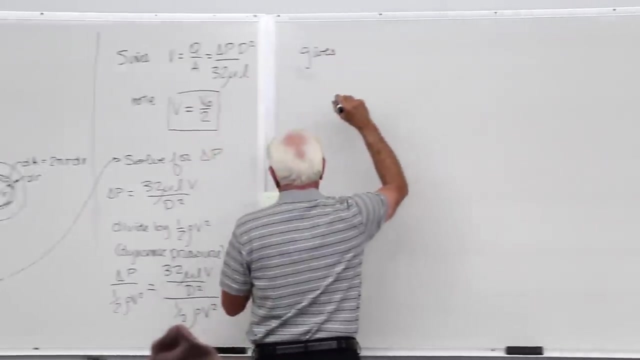 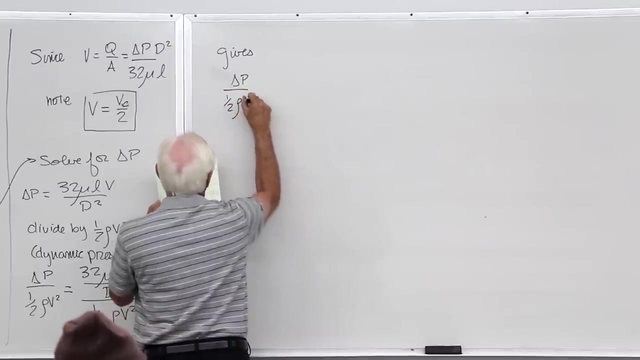 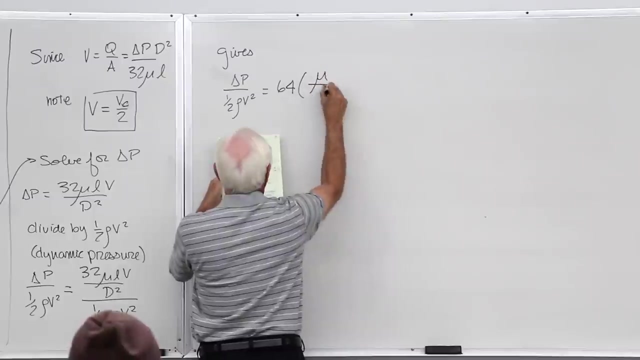 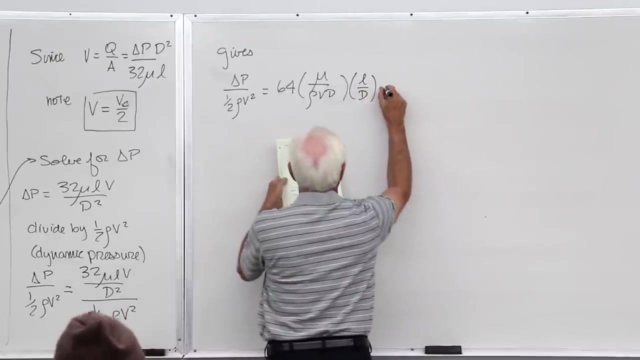 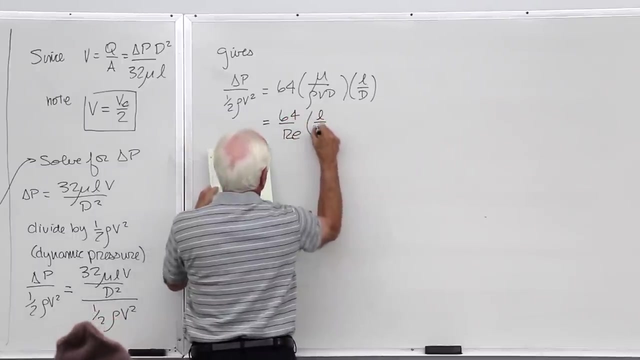 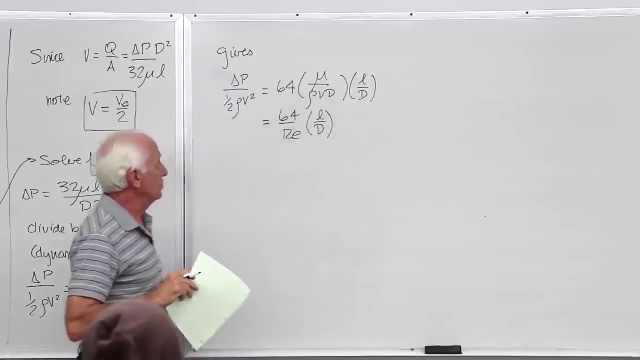 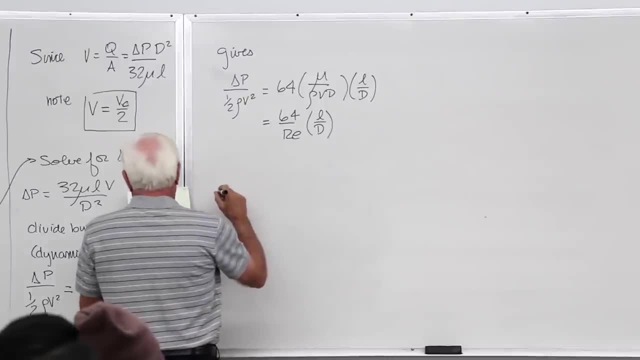 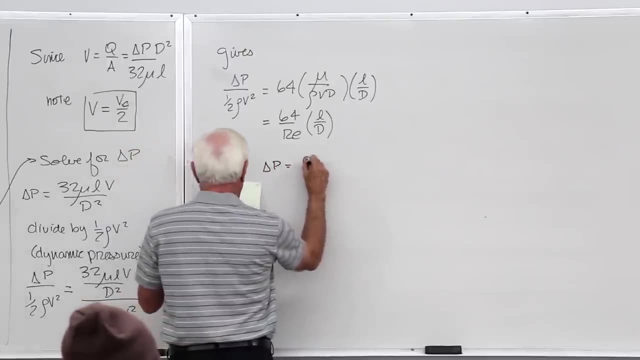 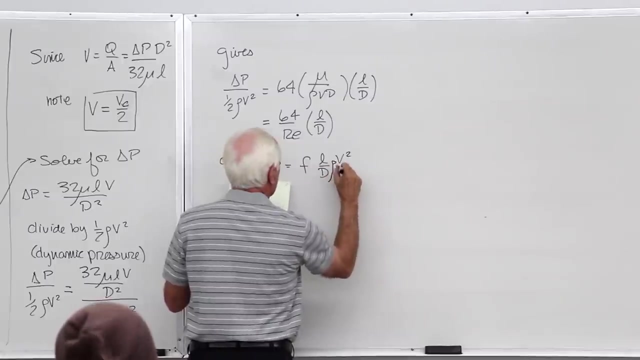 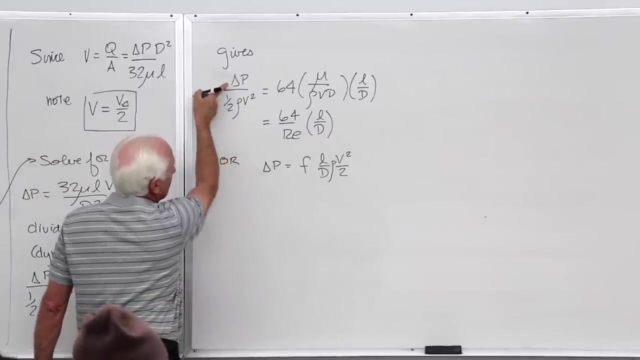 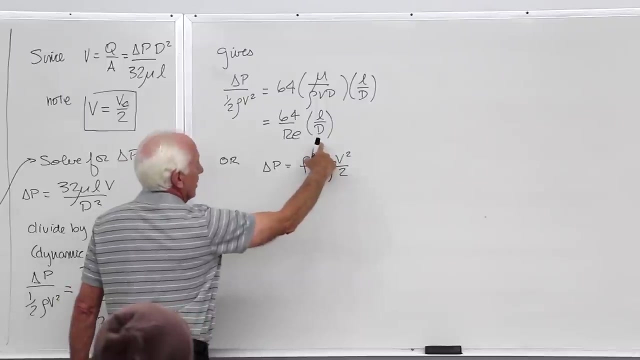 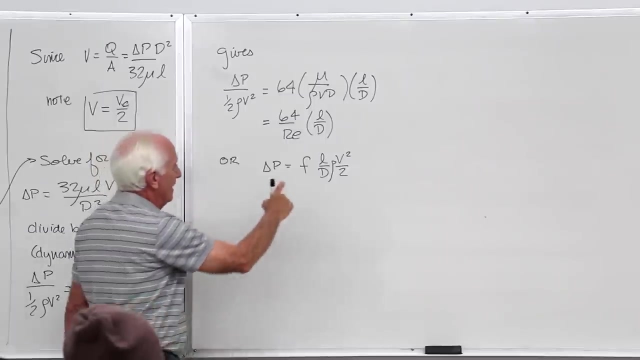 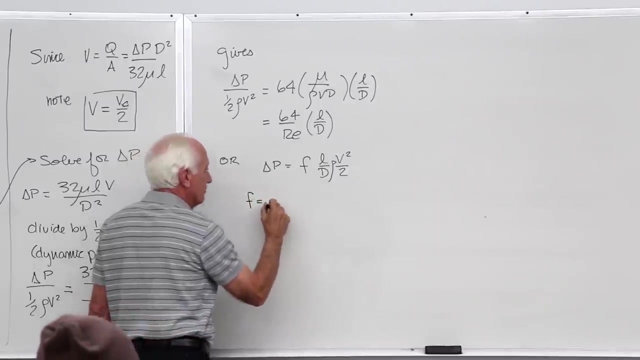 Now here's delta P multiplied through by 1, half rho B squared over 2.. That's that one. There's L over D, This thing, this is a definition. This is a definition. We define F by this equation. This F is called the friction factor. 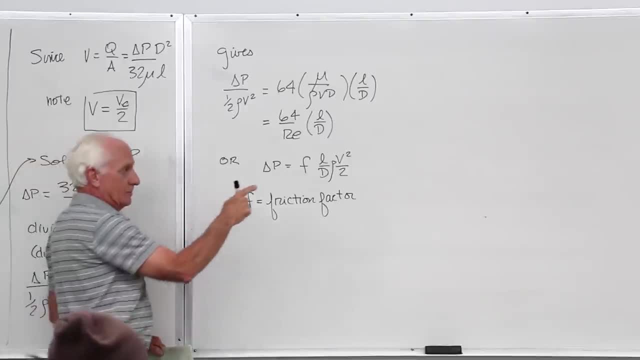 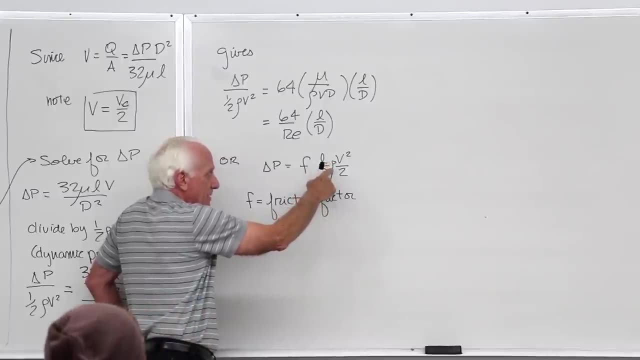 So if we want to find the pressure drop in a pipe, we can take the length, divide it by the pressure, divide it by the pipe diameter, multiply it by the density of the fluid flowing, multiply it by the average velocity squared, divide it by 2,. 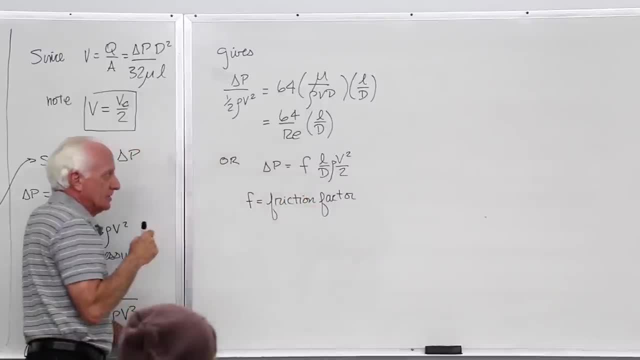 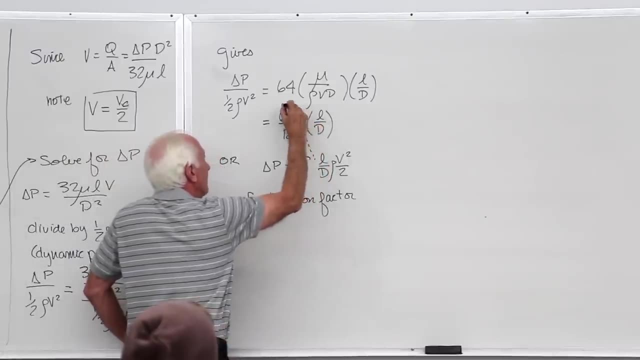 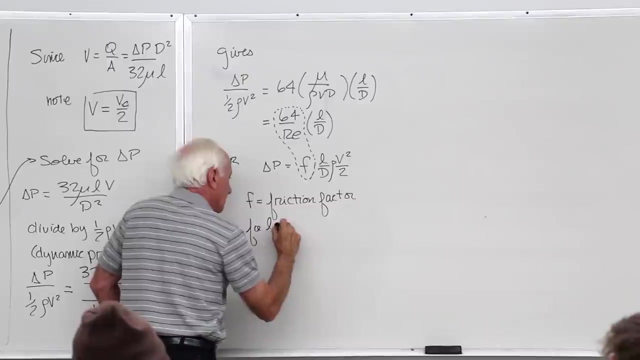 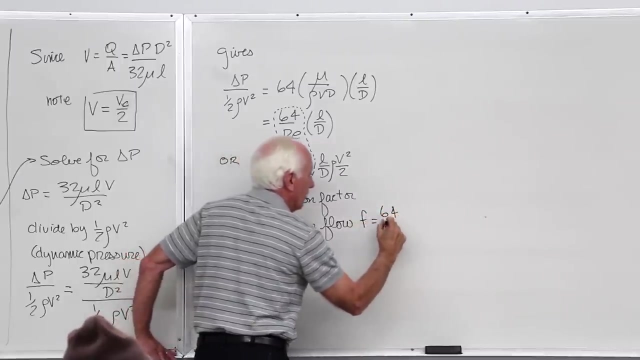 and times a factor which we call the friction factor. Now, if it's laminar flow, you can see in laminar flow what F is. There's F so far laminar flow. F equals 64 over the Reynolds number. Now, friction factor is dimensions. 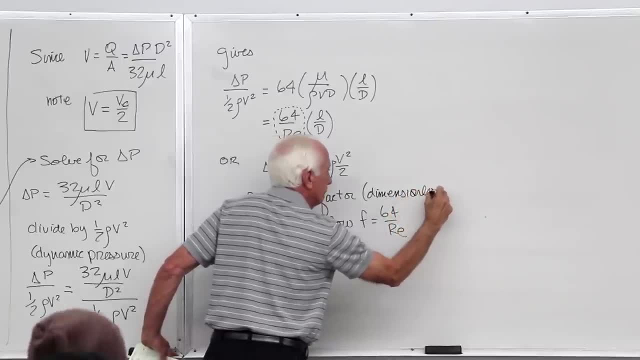 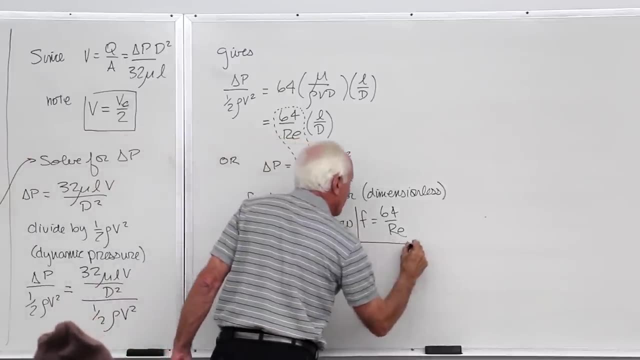 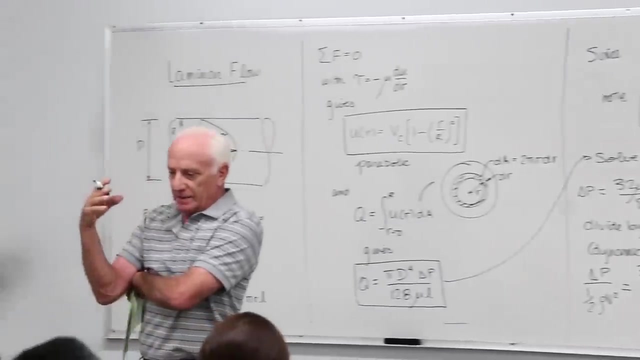 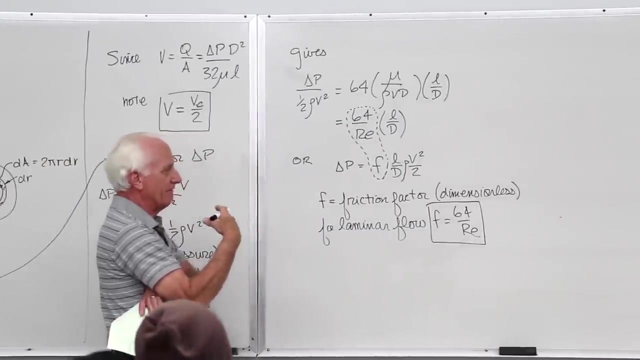 Dimensions. So that's important to know. And again, the friction factor is something we've invented. We define it. Why do we invent it? Because it makes it easy to calculate. It's easy to calculate the pressure drop in a pipe with this concept of a friction factor. 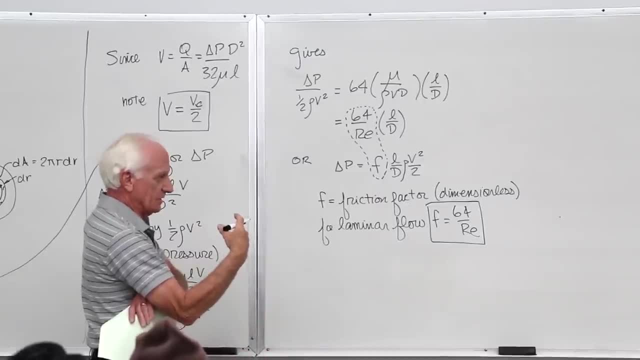 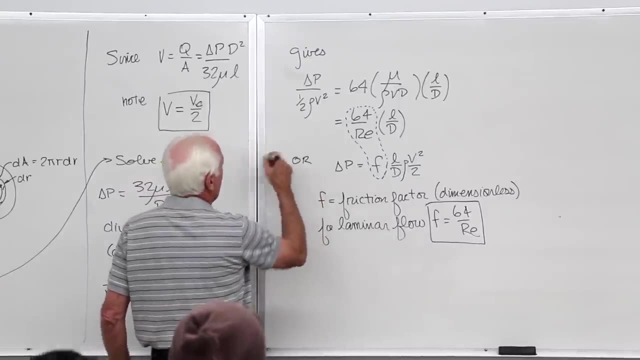 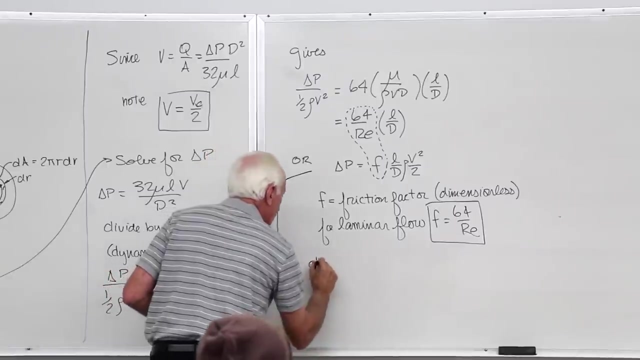 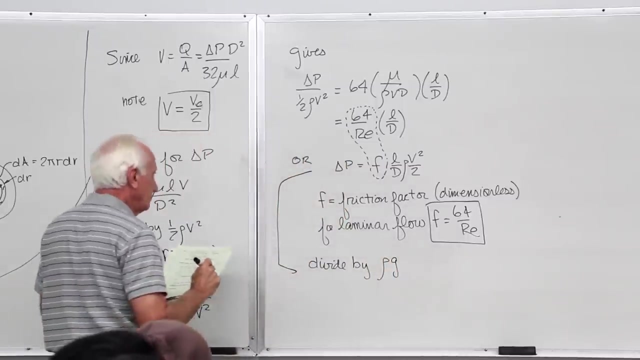 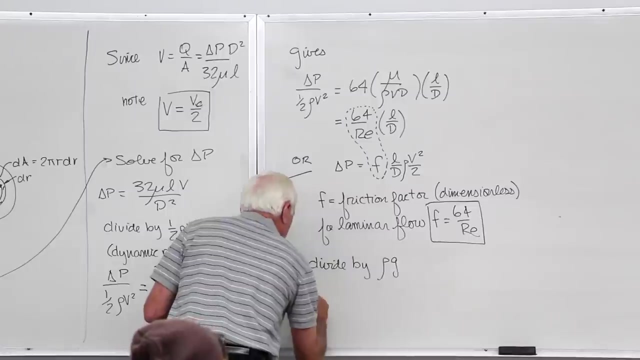 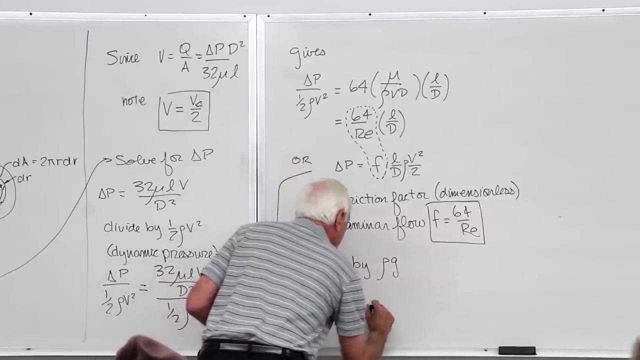 And laminar flow is very simple: 64 divided by the Reynolds number. Now we can also divide this by rho Rho of G. So divide this guy by rho G, So our rho of G is gamma. So we have delta. P over gamma is equal to F L over D. 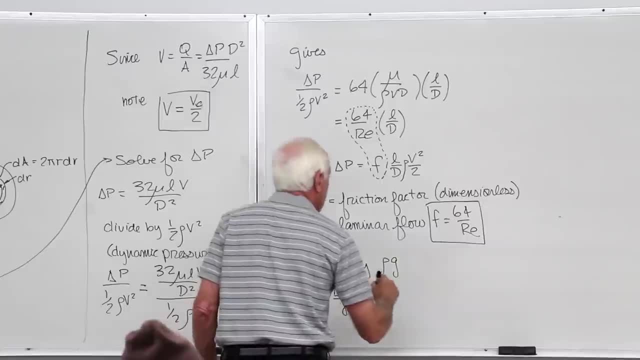 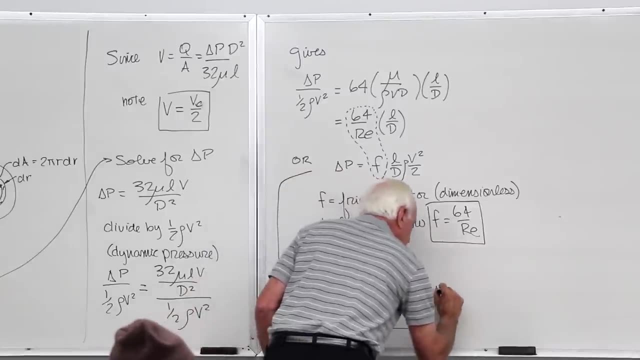 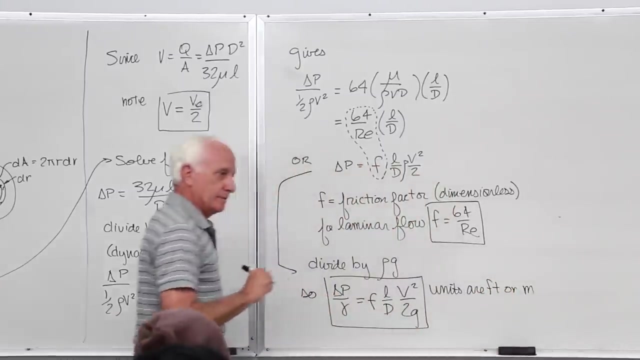 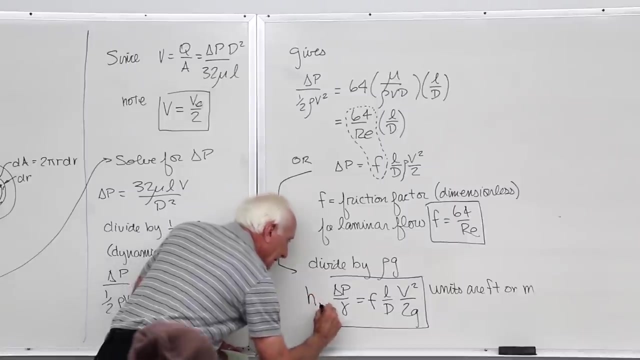 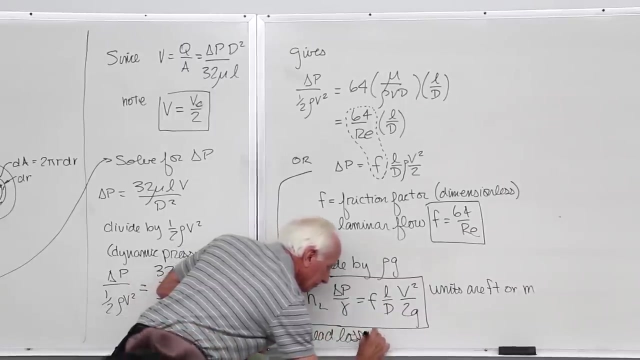 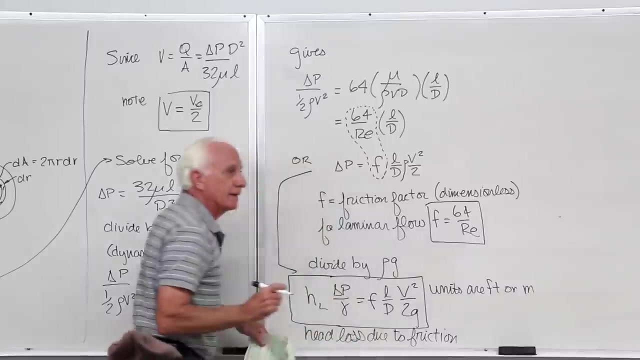 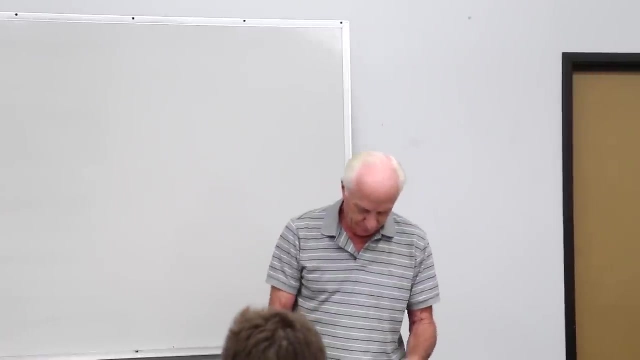 The rho's. cancel out The G's downstairs. V squared over 2G Units are feet, are meters, And we now call that the head loss due to friction. The head loss due to friction. The head loss due to friction. Now for the head loss. 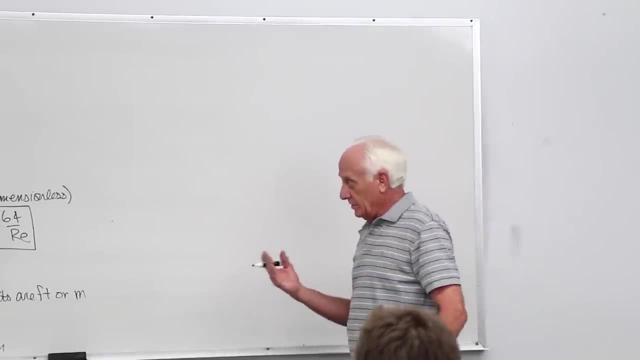 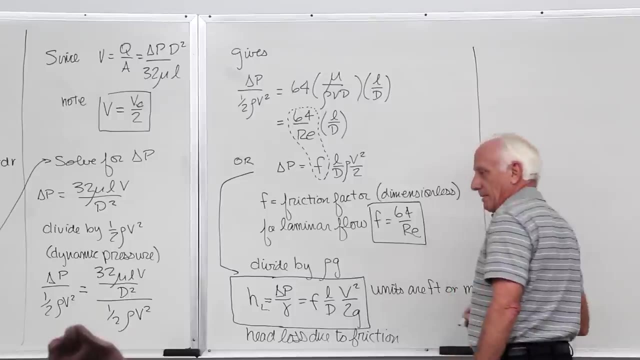 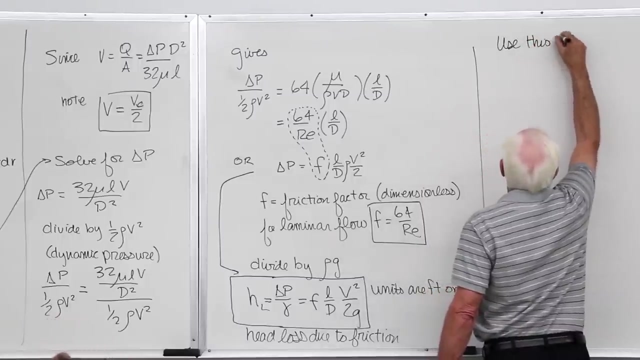 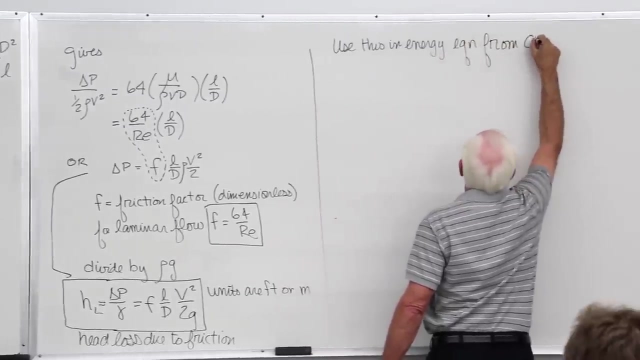 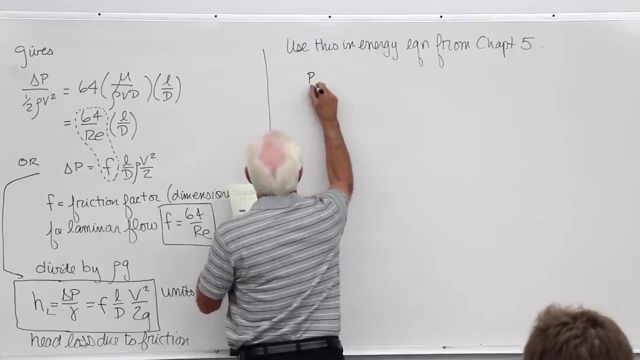 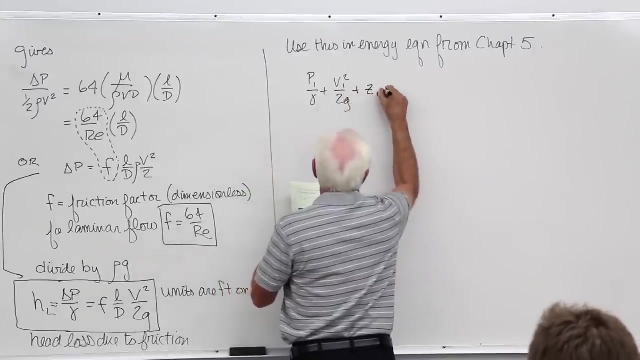 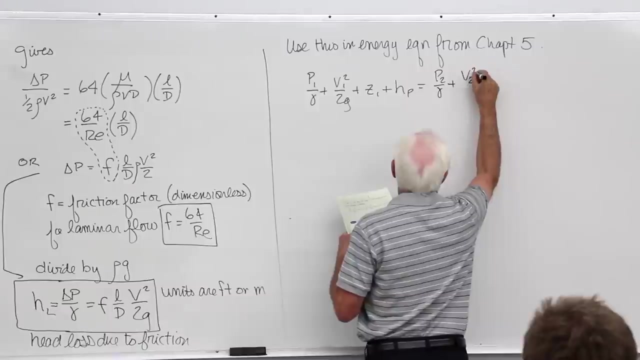 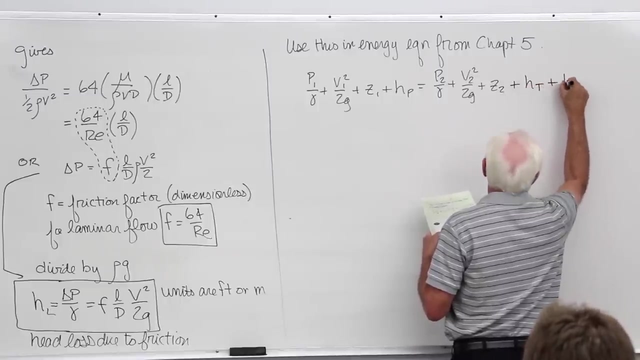 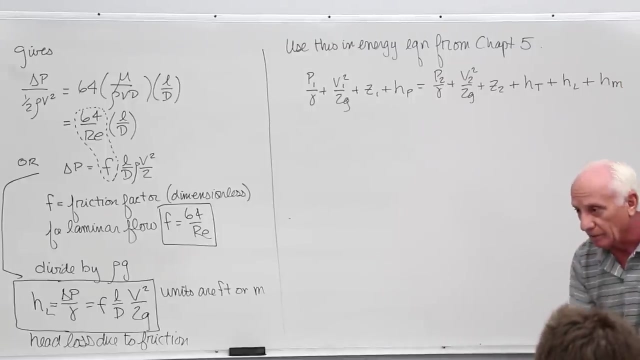 The head loss due to friction 🎵. That's regular people, as I know. ä, of course, in the energy equation from chapter 5.. Okay, the energy equation, chapter 5.. There it is Now. let's just review that equation again. 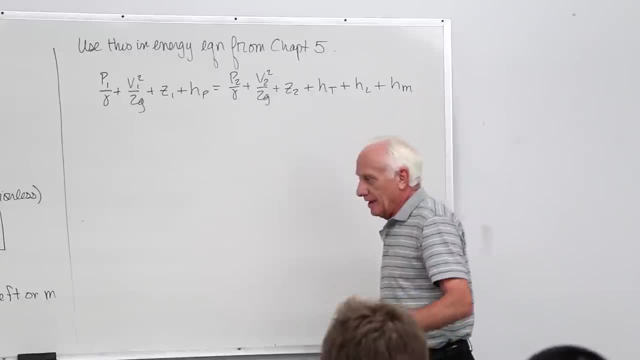 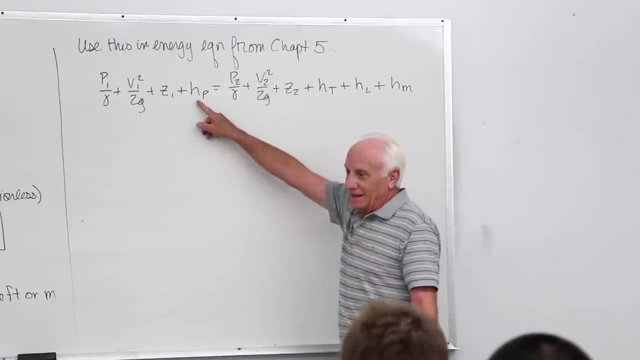 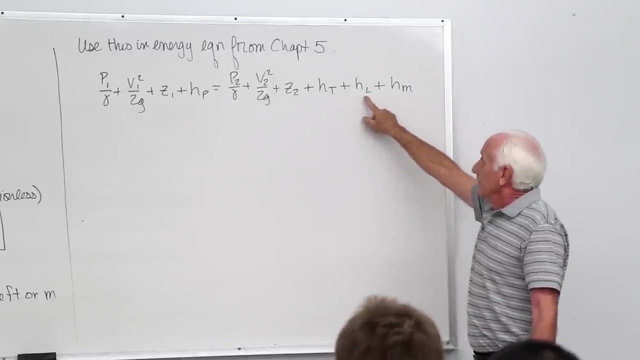 Except now, we allow- compared to Bernoulli's, we allow- many other things to happen. For instance, that's the head developed by the pump. This is the head developed by the turbine. This L stands for the length of a piece of pipe. 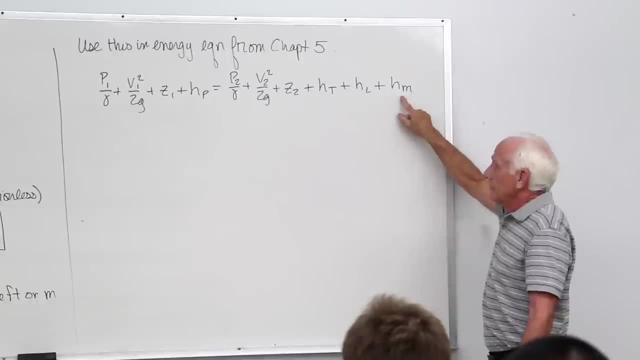 This is the head loss due to pipe friction. This is called the minor losses due to elbows and fittings and valves. This is the head form of the energy equation, because every term has units of feet or meters. This HL now. we used to say this was called the losses. 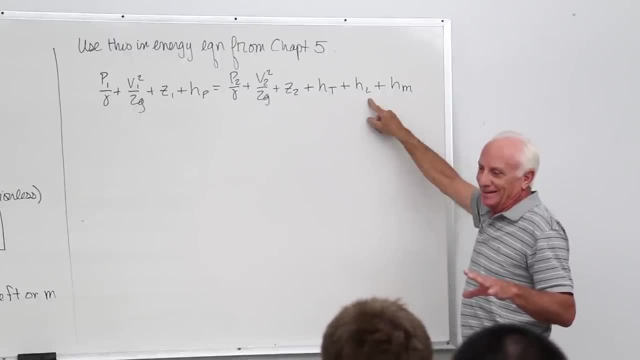 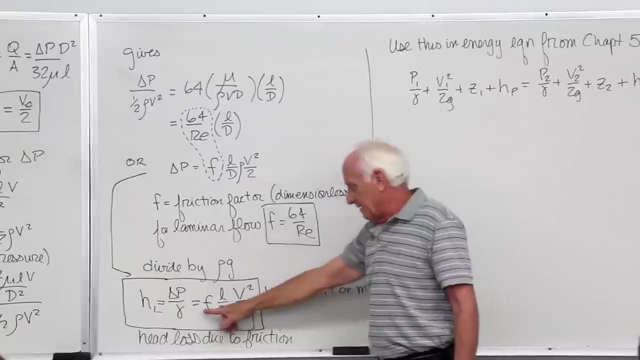 Just call the losses L-O-S-S-E-S. We called it that. Now we've got a way to find the losses. There it is. I've got to find, though, the friction factor. That's the key. I know how long the pipe is. 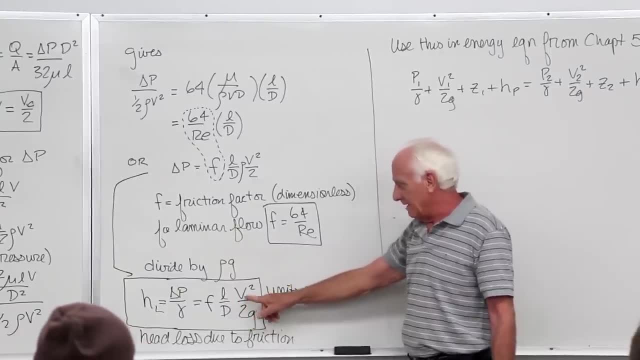 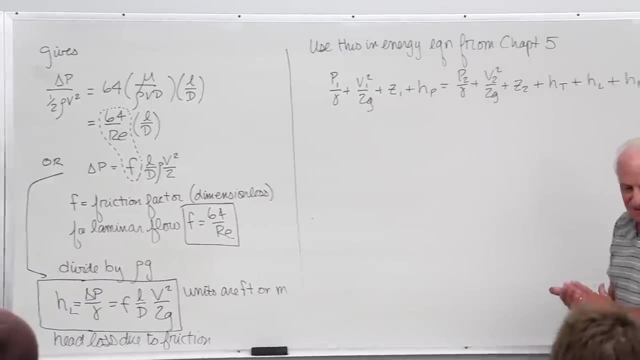 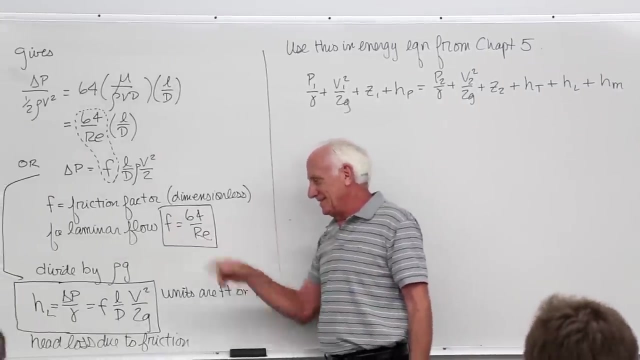 I know its diameter. If somebody gives me the flow rate, I can find the velocity, But it comes down to finding F. So that's what it amounts to: We have to find F, And if we have laminar flow it's very easy. 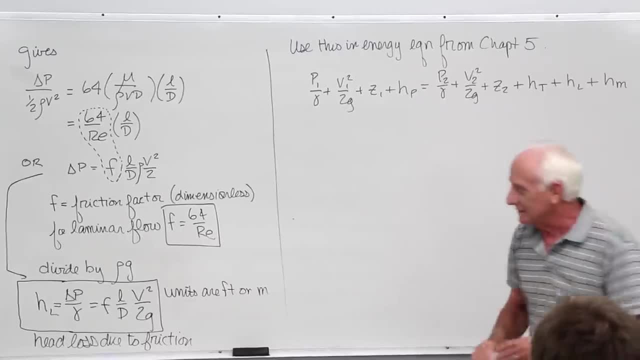 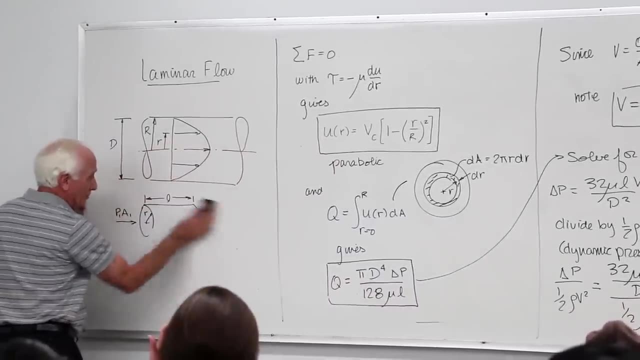 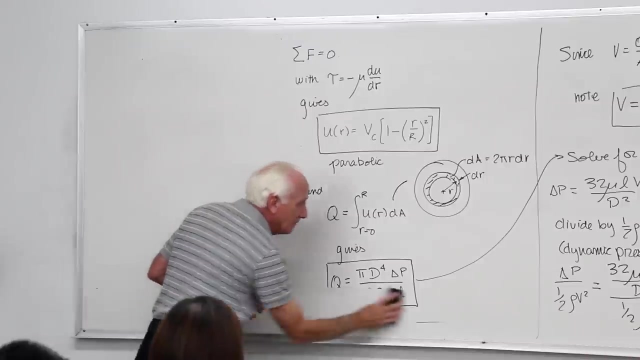 There's the equation for F. Okay, let's work an example. problem in using that? By the way, the reason why we write the energy equation like that on the right-hand side of the board is because everything on the left-hand side is energy that's coming into the fluid. 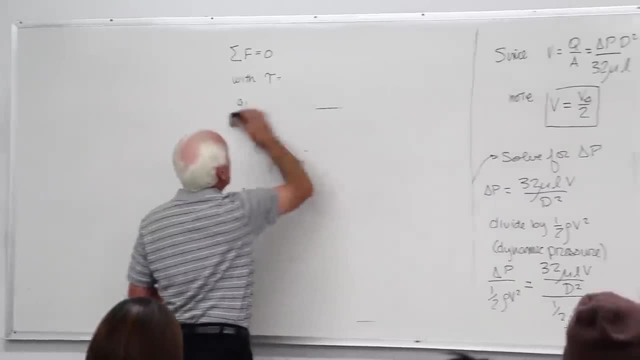 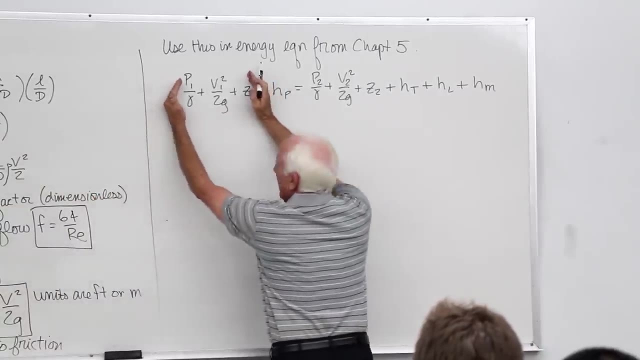 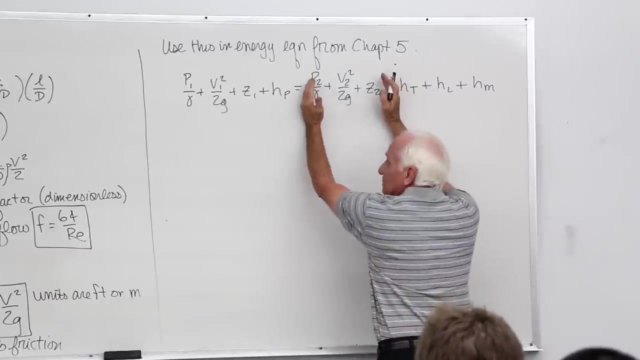 The subscript one means entering A pump does what Adds energy. So the fluid brings in energy, The pump adds more energy. Now where does that energy go? Some of it goes up with the fluid, leaving There it is. A turbine can take energy out. 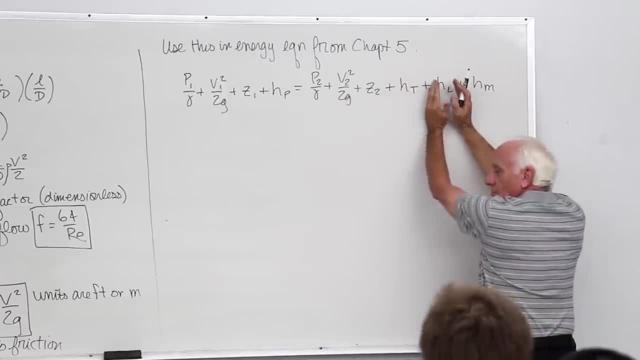 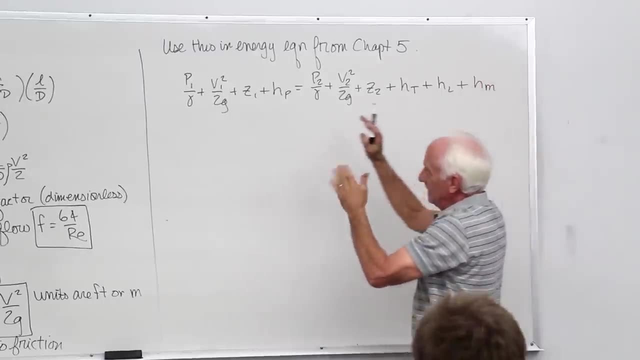 That's what a turbine does. Losses of course reduce the energy available. Minor losses of course reduce the energy available. So that's why it's nice to write that equation in that form, Because you can then talk about it in words. 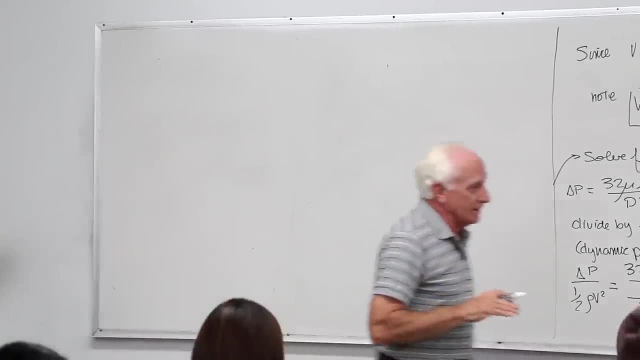 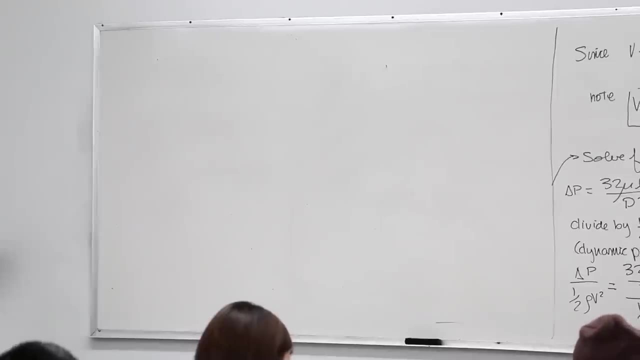 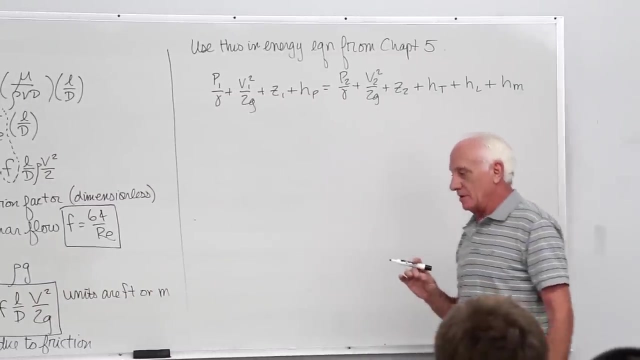 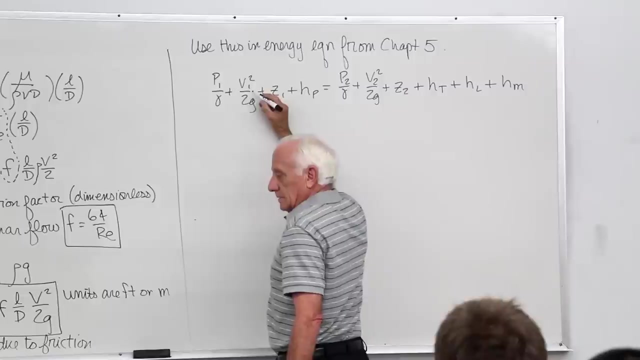 and not just in symbols like that. Okay, so our example then: horizontal pipe. What if we had a horizontal pipe, A horizontal pipe of constant diameter, A horizontal pipe of constant diameter, incompressible, flow Continuity incompressible. 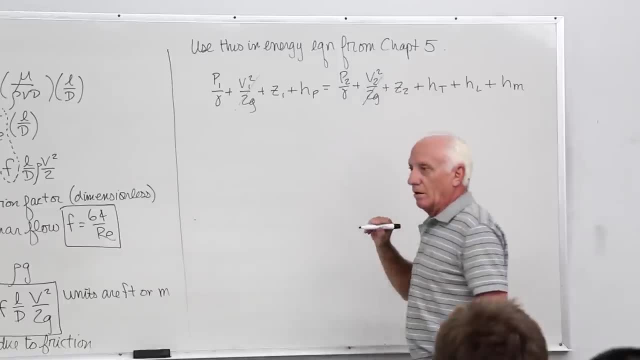 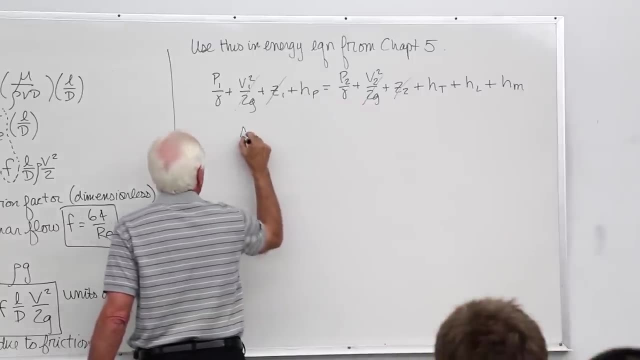 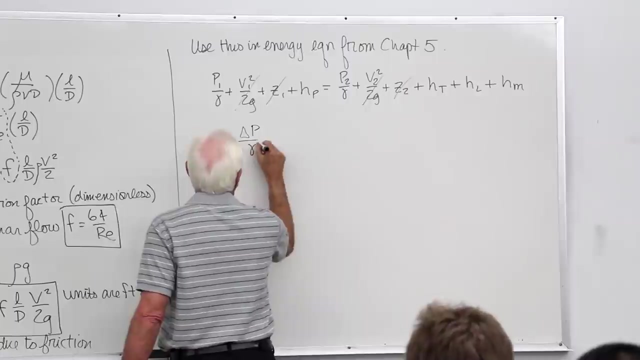 V1, V2, same Horizontal pipe, Z1, Z2.. Okay, We're left with what. P1 is greater than P2.. Yeah, pressure Coming in Delta, P divided by gamma equal If there's no pump, goodbye. 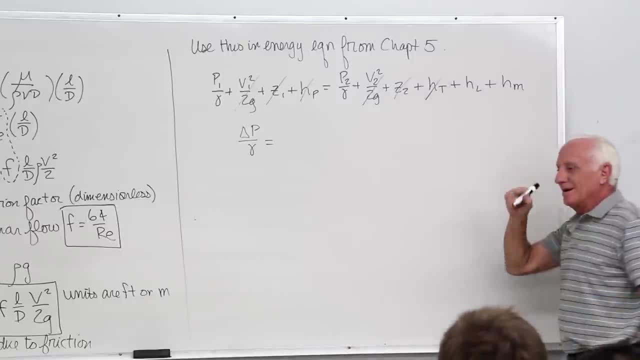 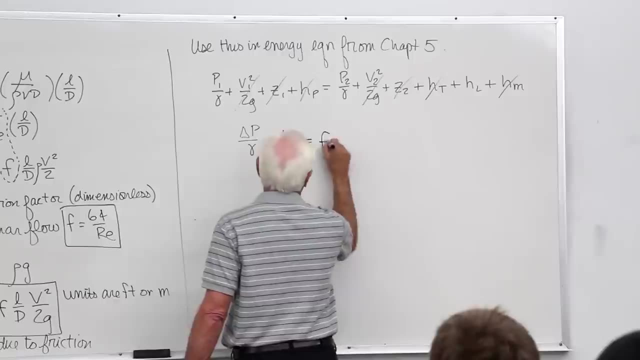 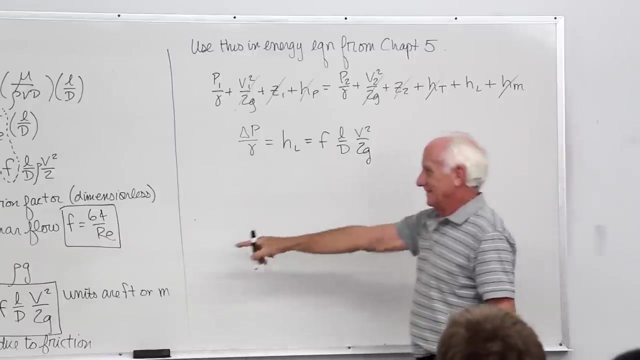 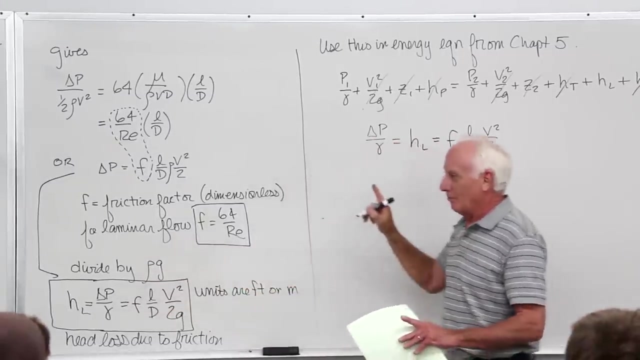 If there's no turbine, goodbye. If we neglect, minor losses gone. Then, and only then do we get that guy. Okay, That's where it comes from, Donner. just so you know where it came from. That equation there is valid for what again? 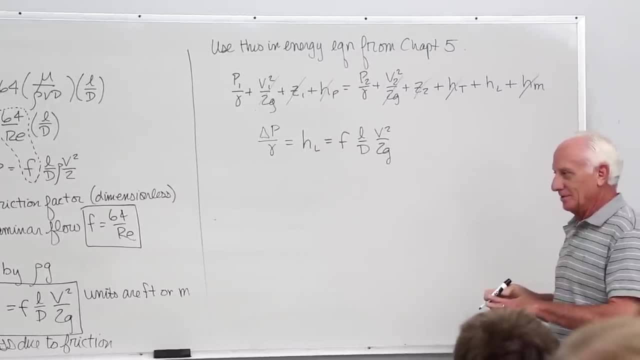 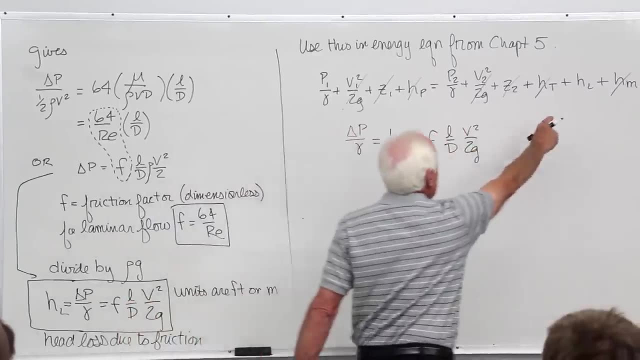 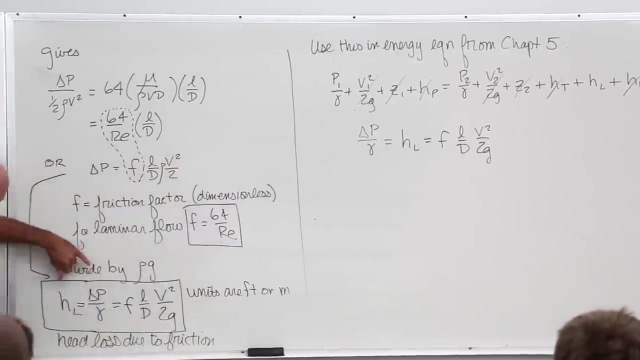 Incompressible horizontal pipe, no pumps, no turbines, neglect, minor losses. If that's not true, go back up there. That H sub L is still the same thing, But you don't have this equation. See this equation right here. 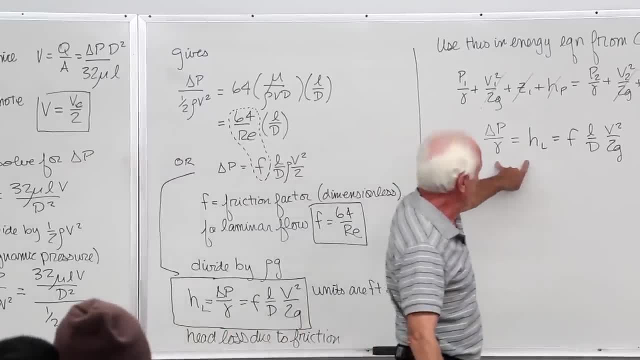 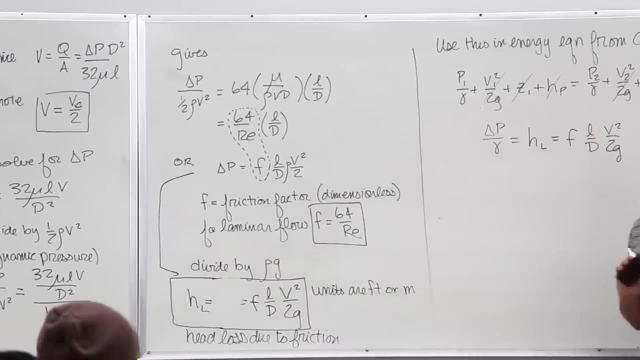 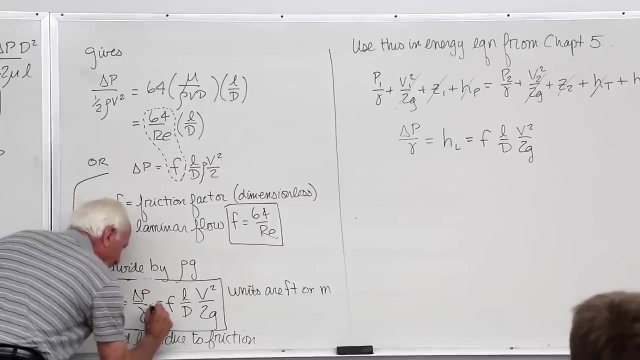 H sub L, equal delta gamma. That's where it comes from. So just be careful when you use that guy. That thing's always true. That thing is always true. This thing is sometimes true. When's the sometime? Here we go again. 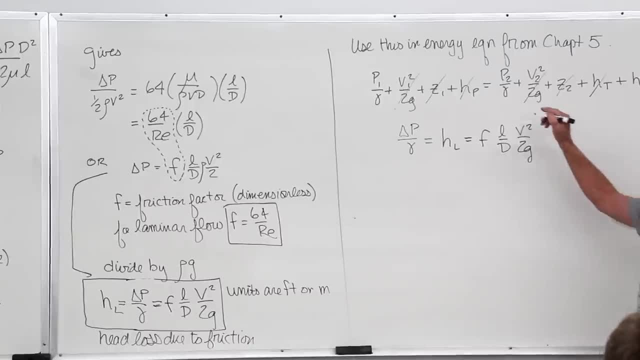 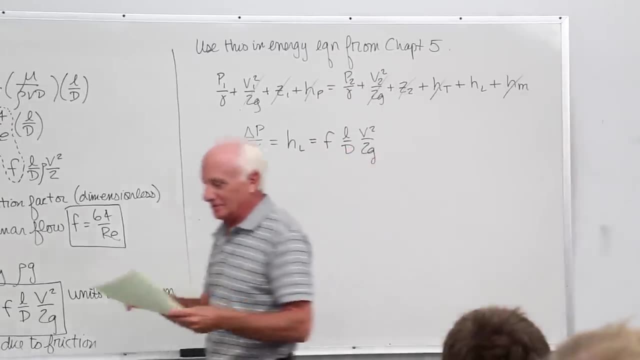 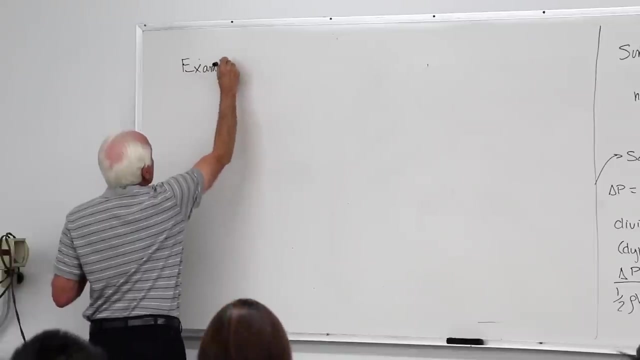 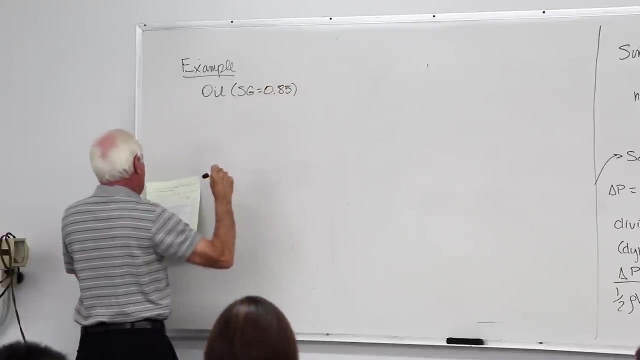 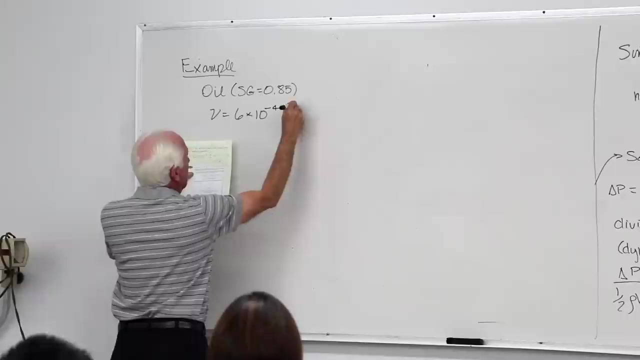 No pumps, no turbines, neglect, minor losses and incompressible horizontal pipe. Okay, So this example is incompressible horizontal pipe. Oil specific gravity 0.85.. Okay, Viscosity, kinematic viscosity- 15 centimeter diameter pipe. 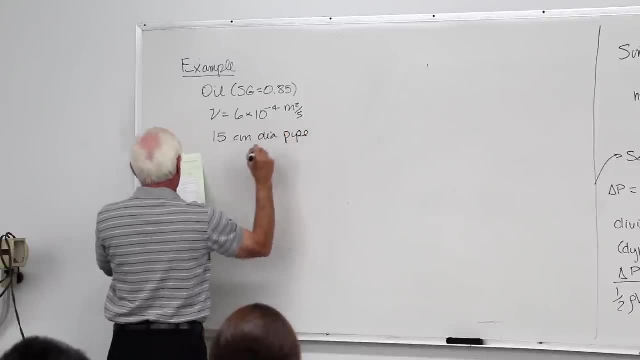 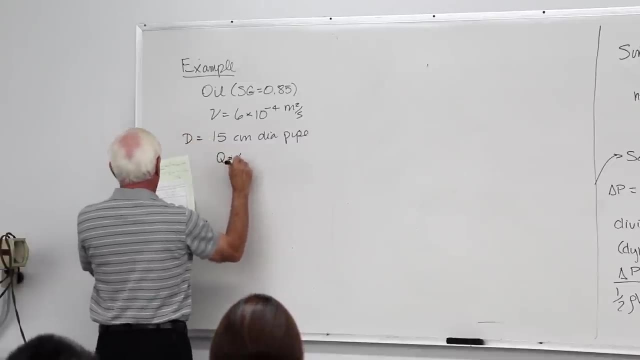 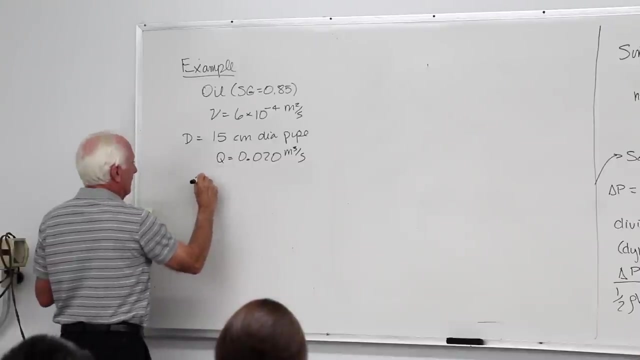 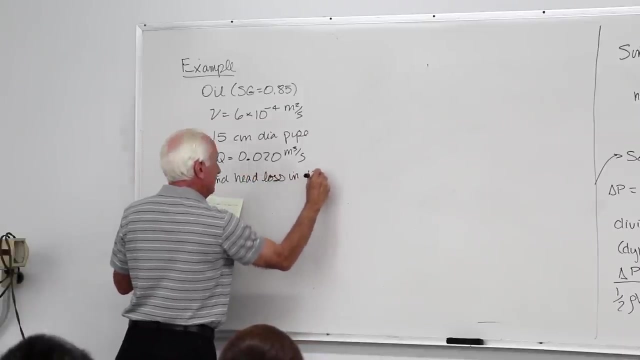 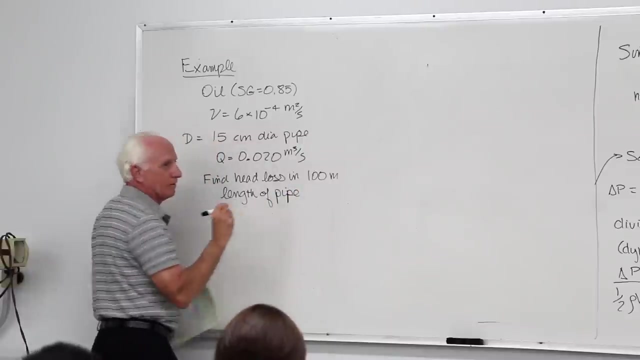 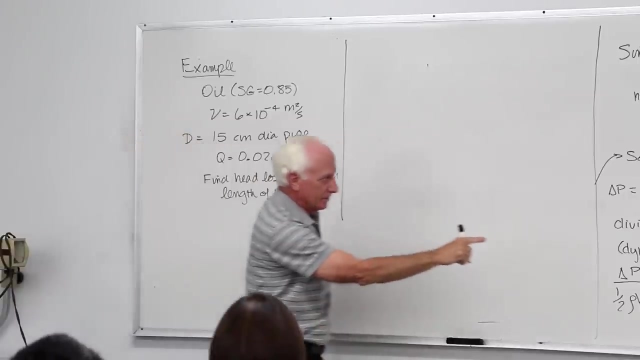 And a flow rate Q 020 cubic meters per second. I want to find head loss in 100 meter length of pipe. Okay, There it is, Head loss. Head loss H sub L is horizontal, Incompressible Constant diameter. 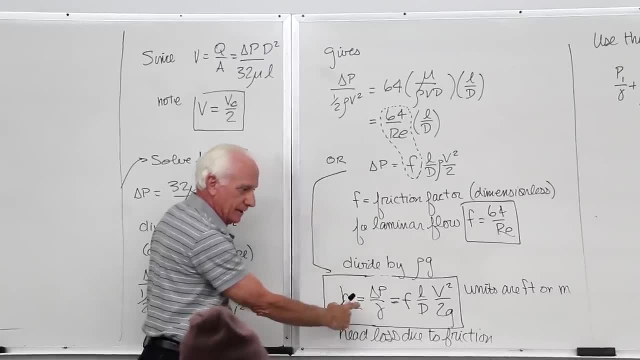 There it is: H, No pumps, no turbines, no minor losses. H sub L, Delta P over gamma, Which is F: L over D. V squared over 2 G, V squared over 2 G. Delta P, Delta P. 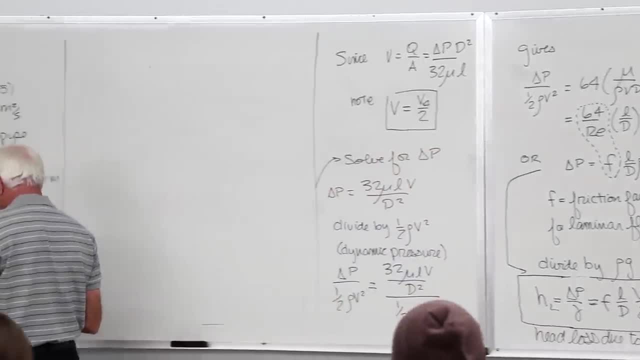 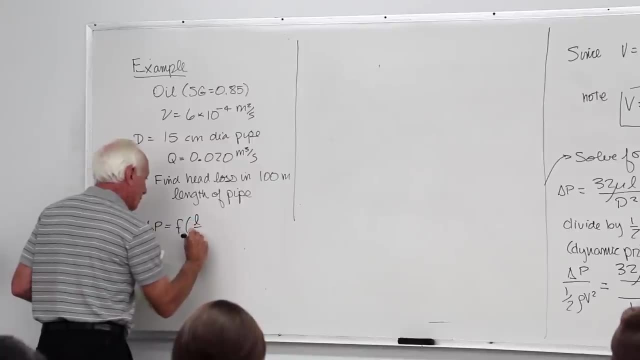 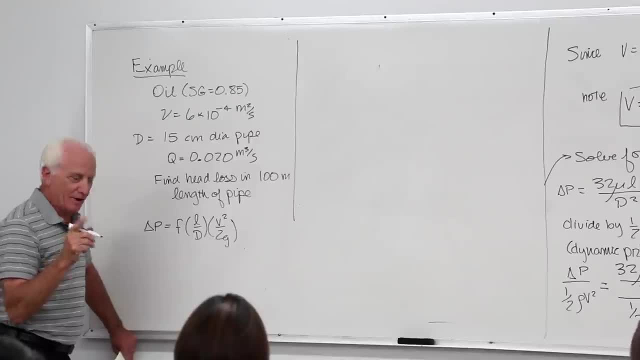 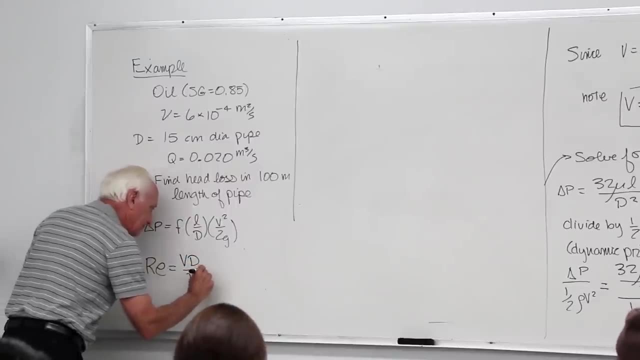 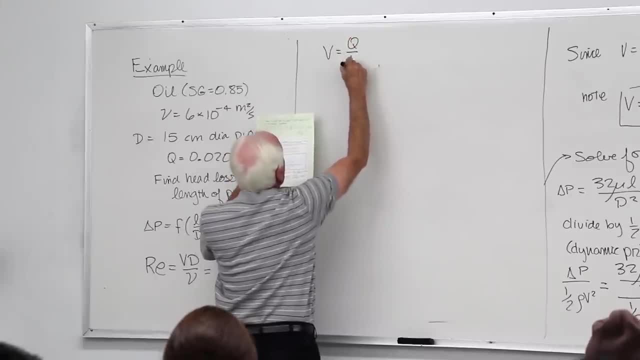 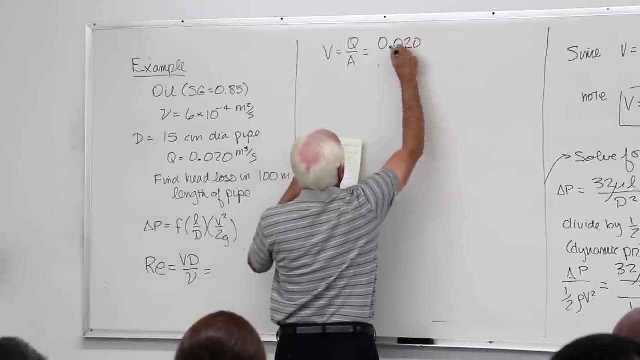 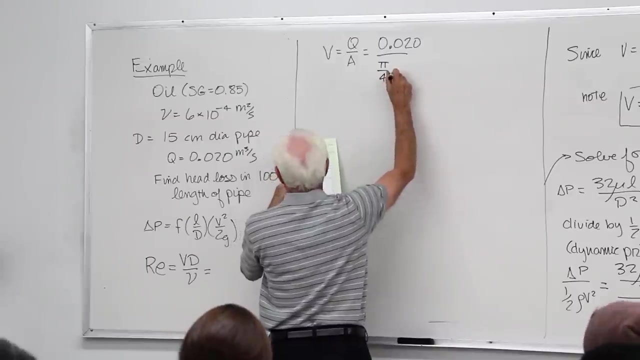 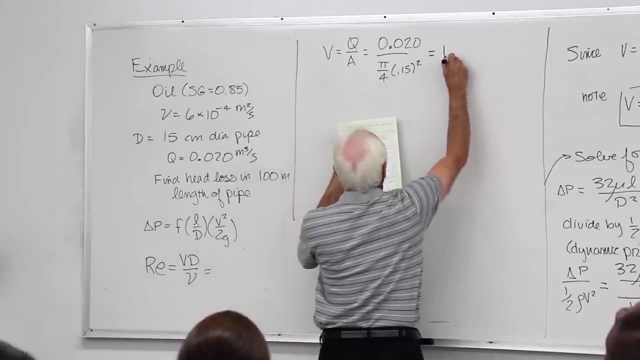 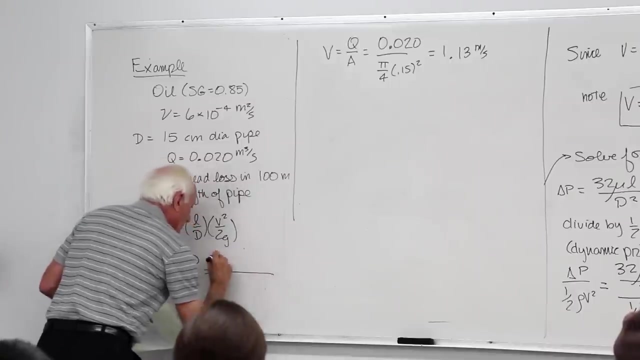 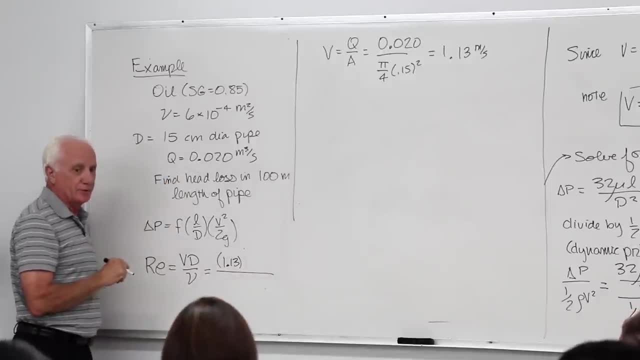 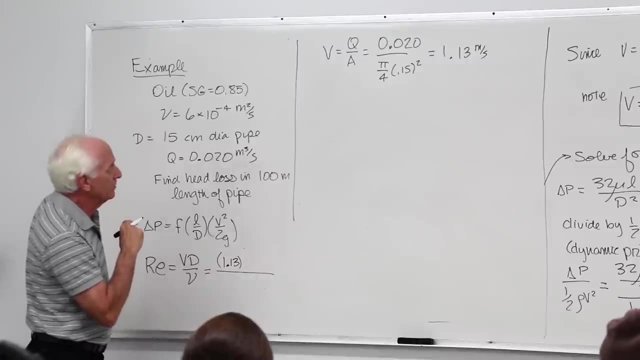 equation which was in terms of Q for the Reynolds number. You could do that too. That's a shortcut way to do it really, But I found the velocity first. I'll need it. I think maybe later on We'll see Times. the diameter. Diameter is 15 centimeters. 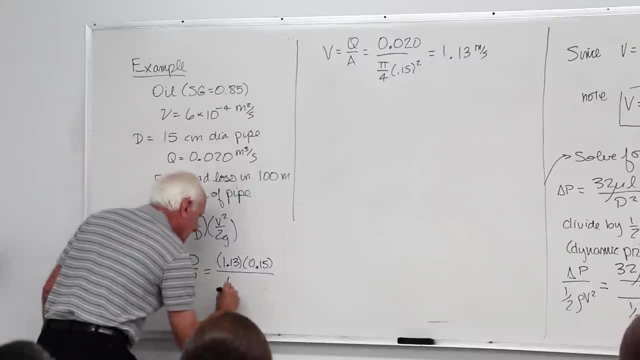 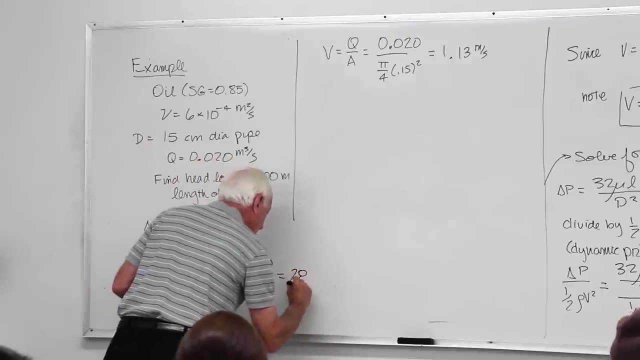 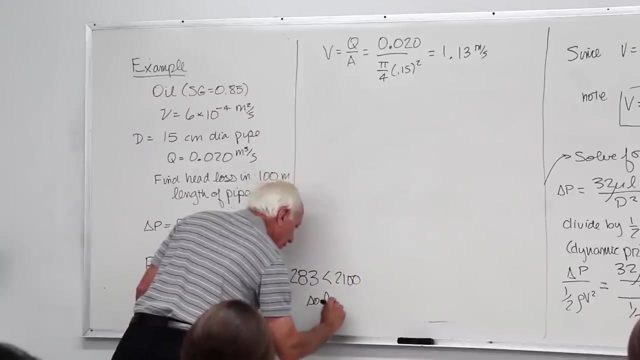 Divided by kinematic viscosity, given 6 times 10 to minus 4.. So the Reynolds number 283.. Less than 2100, so it's laminar, Okay. so now we know, yup, okay, laminar flow. 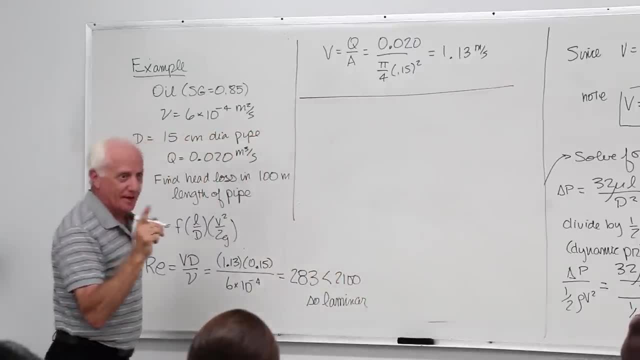 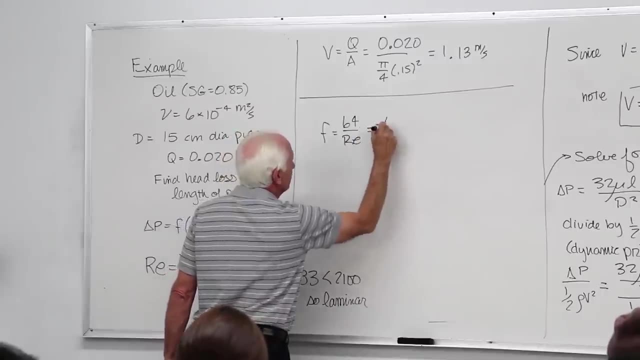 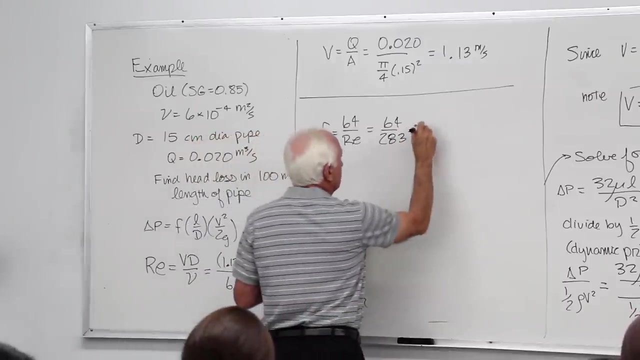 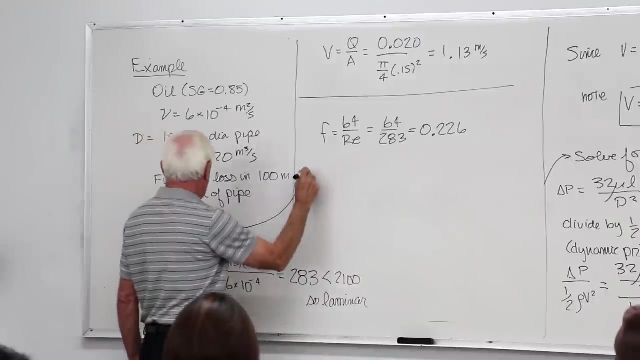 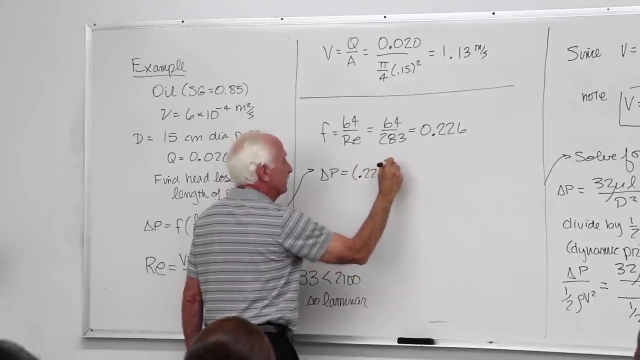 Once I know that now I can get the friction factor, Friction factor 64 over the Reynolds number, Friction factor .226.. .226. .226.. Now I plug it into the delta P equation: F226.. The length of the pipe: 100 meters. 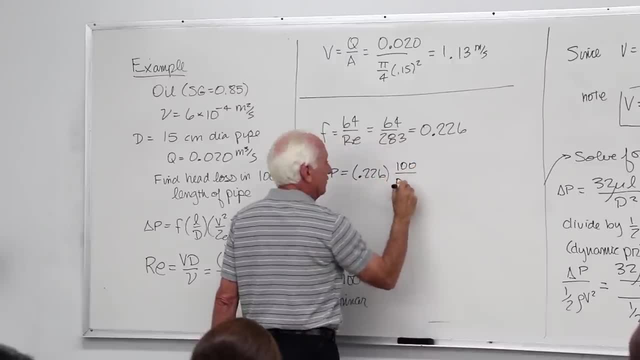 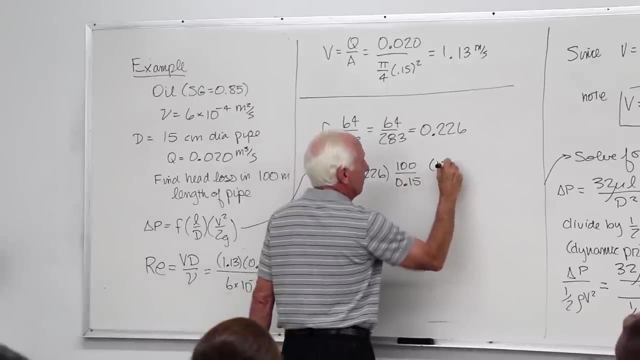 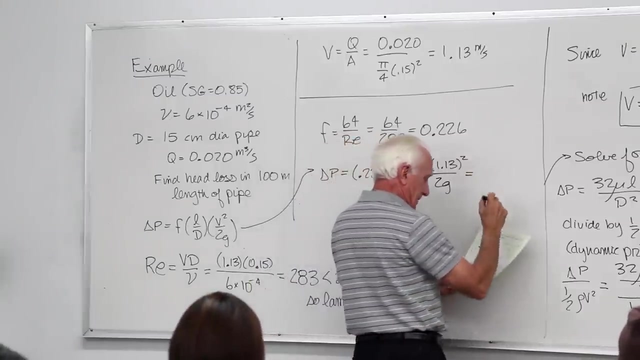 The diameter of the pipe: .15 meters. Yeah, I need V squared. V 1.13 squared, Divided by 2g .15 meters. Divided by 2g 9.83 meters. That's you what happened to the the gamma. 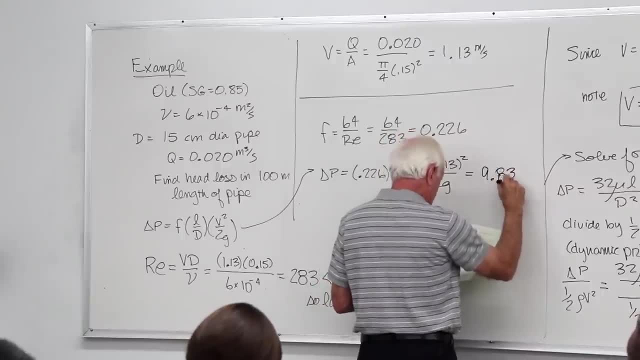 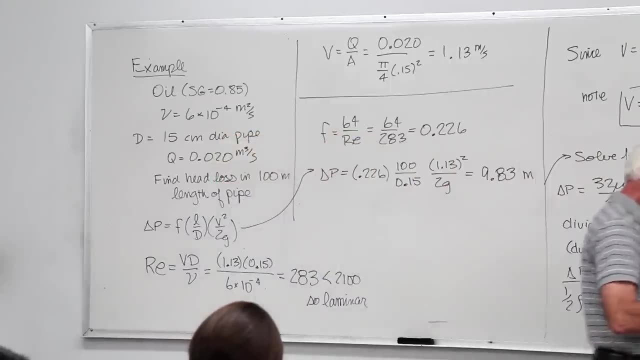 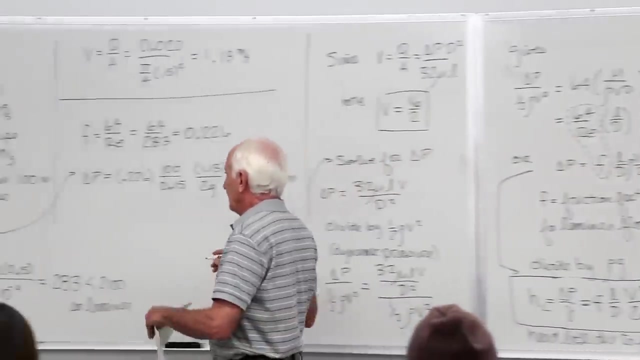 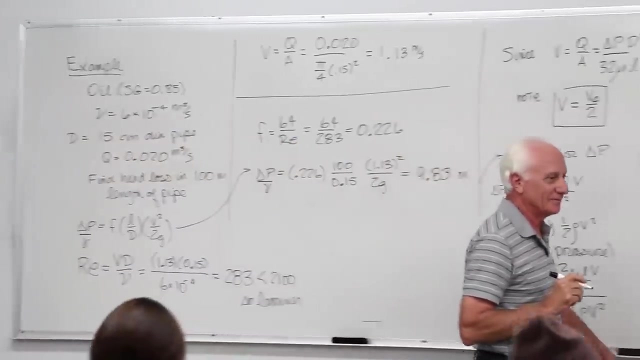 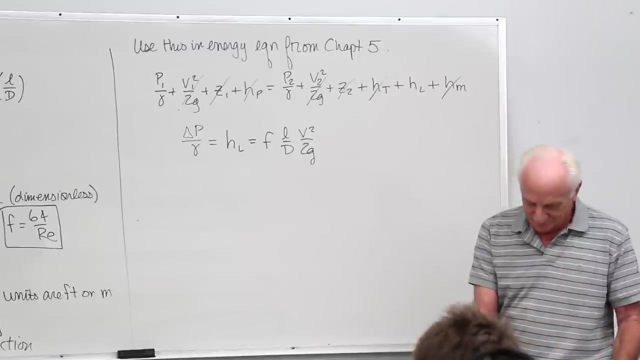 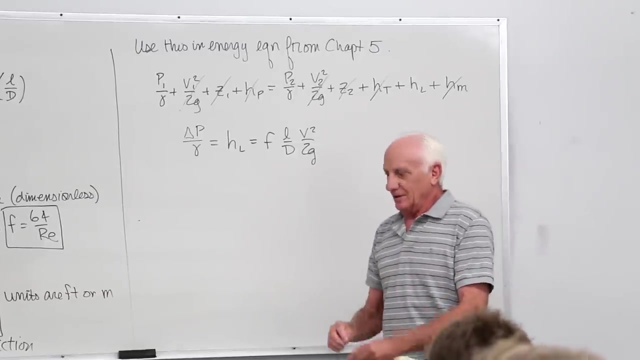 It just popped up again. thank you, 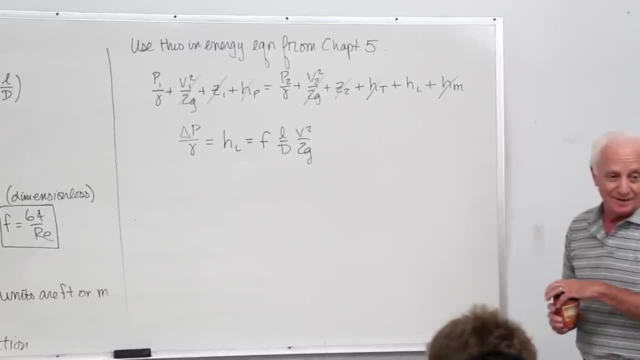 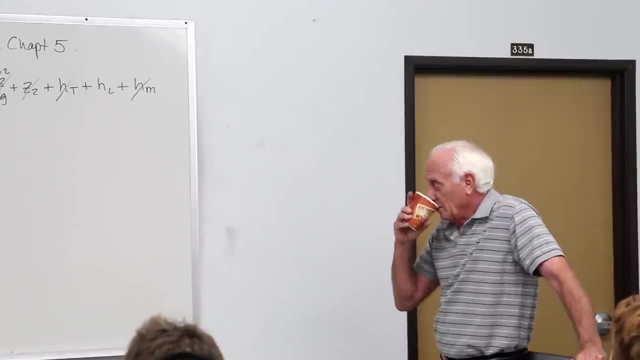 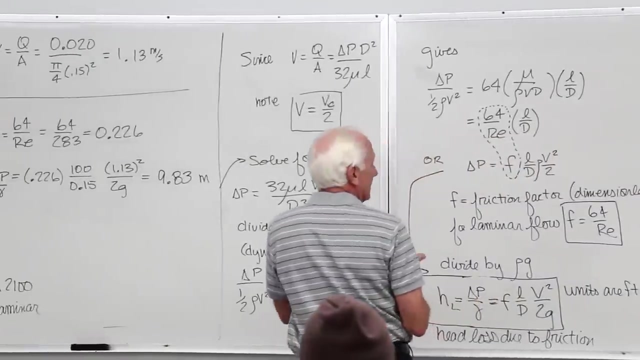 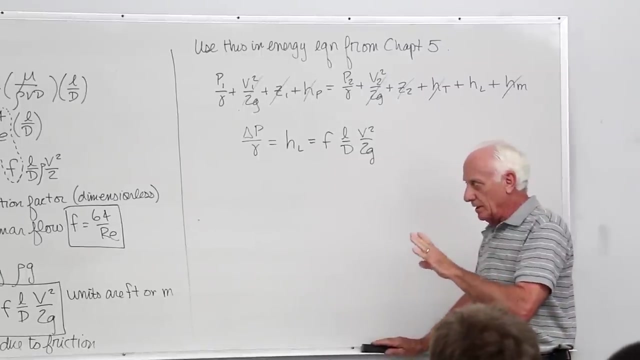 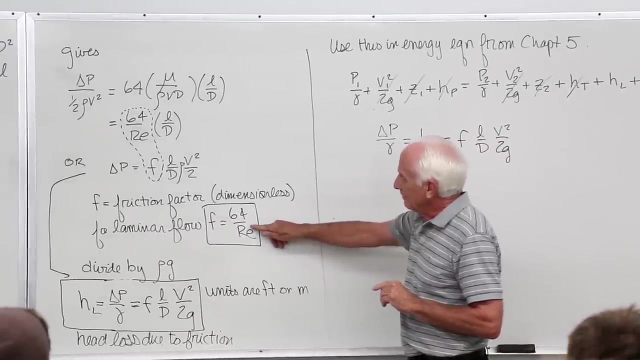 Okay, Let's, I think I'll put it over here. By the way, this equation is still going to hold, whether the flow is laminar or turbulent. The only thing we can't do is this guy right here, Because he came from here, and he came from here, and 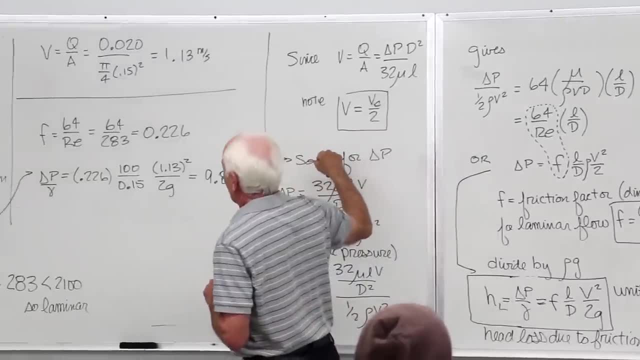 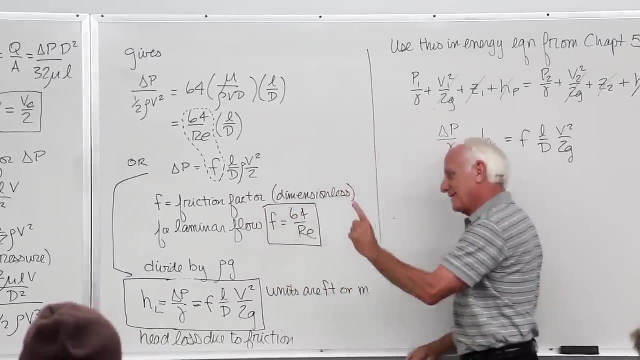 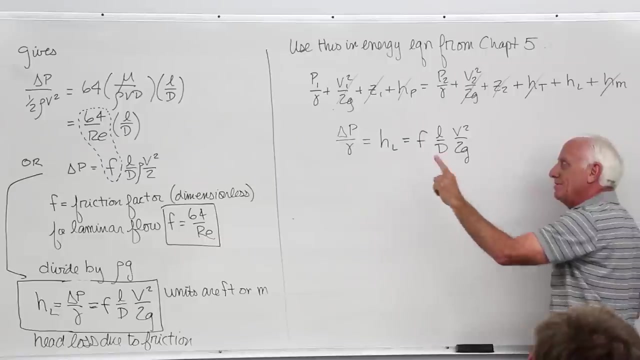 he came from here And it came from Newton's law of viscosity. So this is the one we cannot use for turbulent flow, But this equation is still true. This equation is still true, Except now we need F for turbulent flow. Let's just 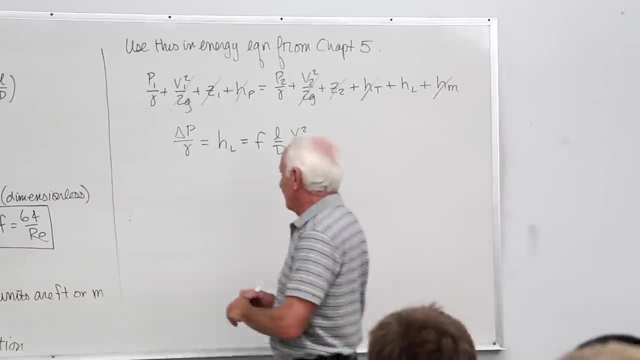 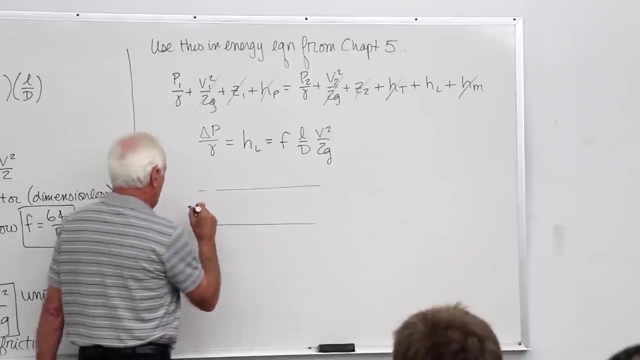 review real quick. laminar and turbulent flow. Laminar flow: pretty much if you follow a fluid particle, it's going to be a fluid particle. If you follow a fluid particle as it moves down in a laminar flow field, it pretty much is. 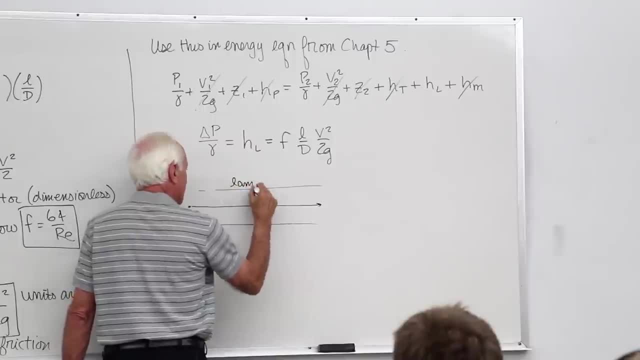 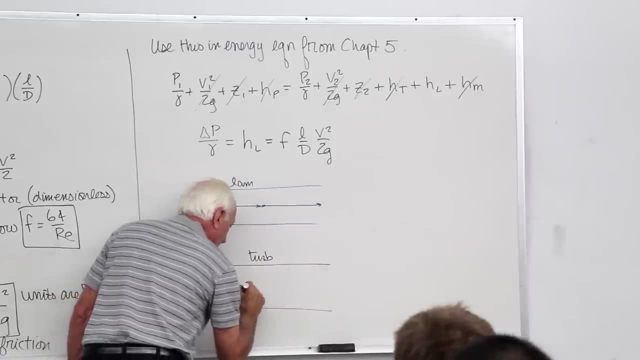 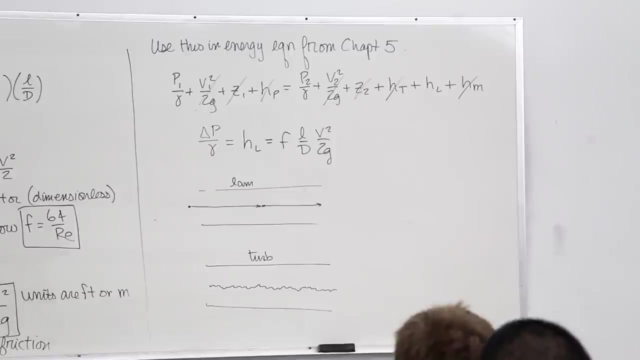 straight Now, if you go to a turbulent flow field particle might, if you greatly exaggerate it, just to show you on the board that's what it does See. the word laminar comes from lamina. What does lamina mean? Lamina means flat. 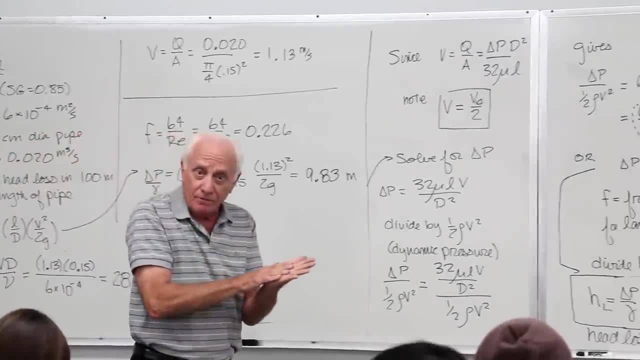 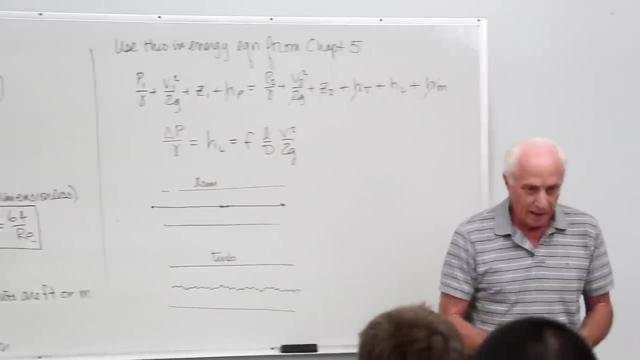 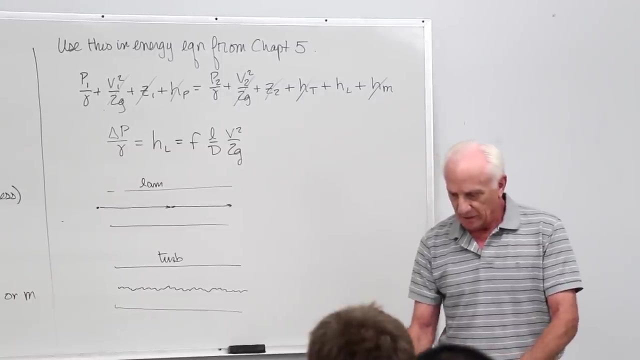 surfaces, A laminate flooring for your kitchen or whatever It's a flat surface, A textbook. these pages are like lamina, They can slide over each other very smoothly. They slide over each other, That's lamina, So the fluid molecules pretty much go in a 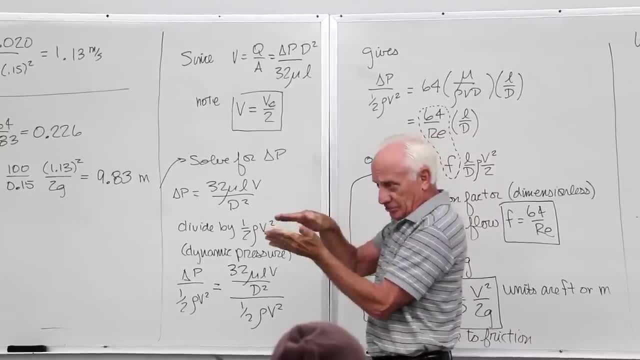 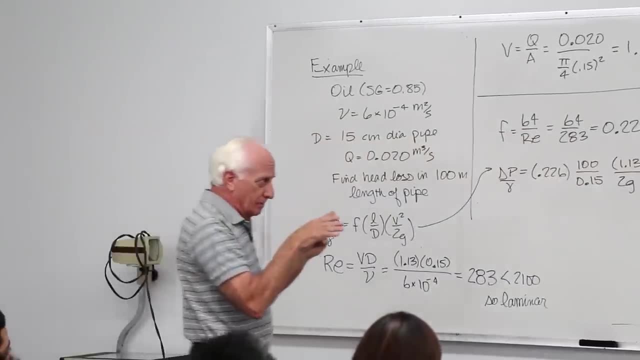 U direction, X direction the U velocity, And they don't hit each other too much, They go straight like this. They don't hit each other too much. Okay, Now, when you get to turbulent flow, you get a little V component of velocity. 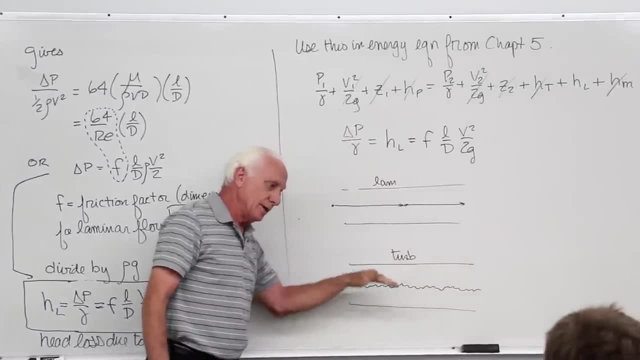 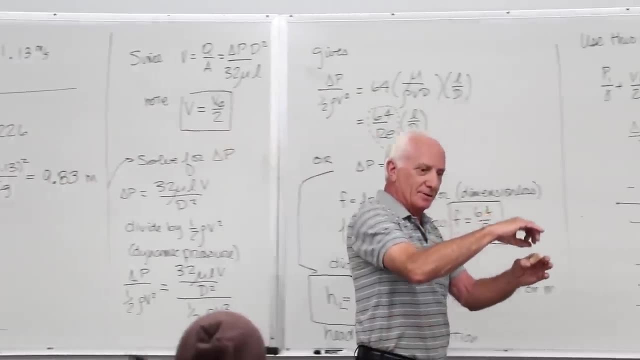 Don't forget: U goes this way, V goes normal to it. You get a little V component, So this molecule starts to bounce around like this. as they go down, They're bouncing like this And, of course, two cars in a freeway, one guy going, like this one going. 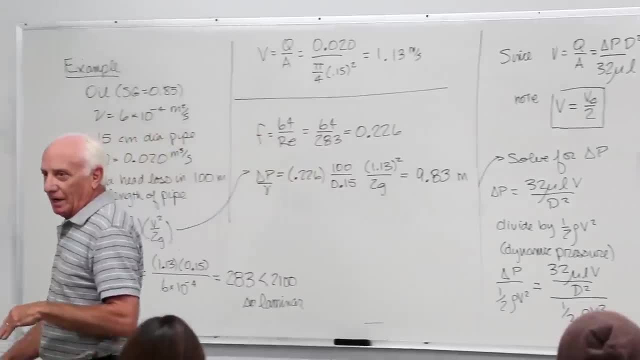 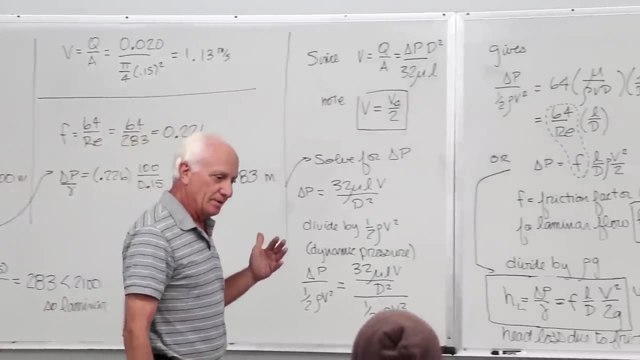 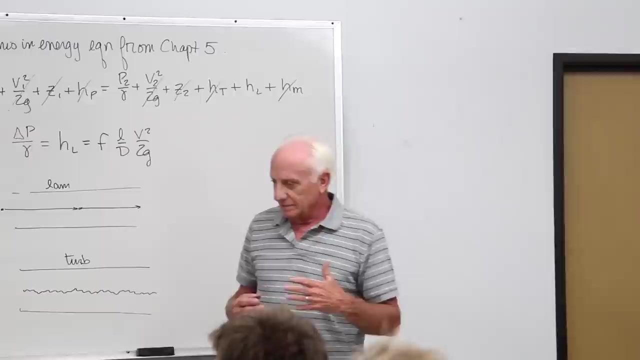 like this. Guess what happens? Metal on metal friction slows the car down. Guess what happens to the molecules in the water. They bump into each other, They exchange momentum And friction develops And they start to slow down. This is rougher, It's more reaction. So that's what's happening. 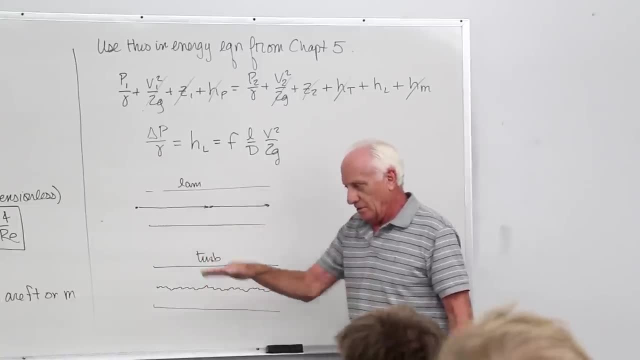 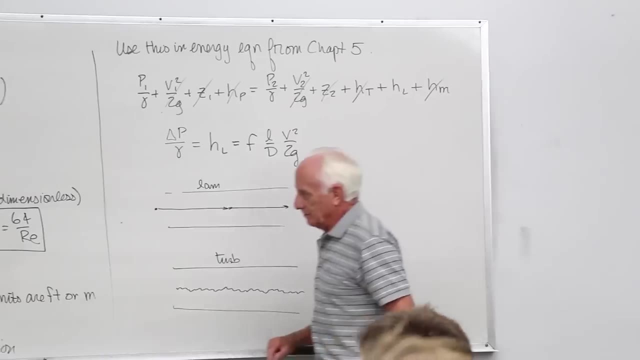 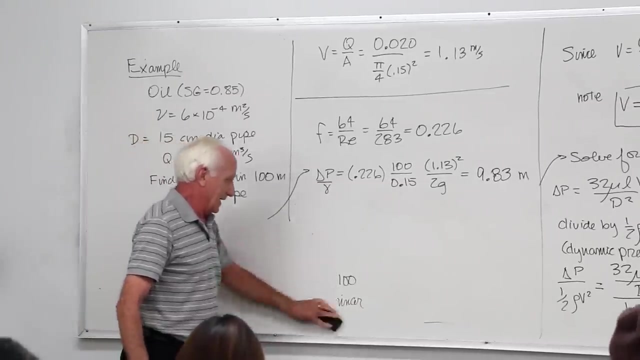 here There is a V component of velocity in turbulent flow as opposed to a nice smooth flow in lamina flow. Okay, Let's get down to turbulent flow a bit. Turbulent flow: Okay, to get the F values. they didn't go to any theoretical derivation like we did. 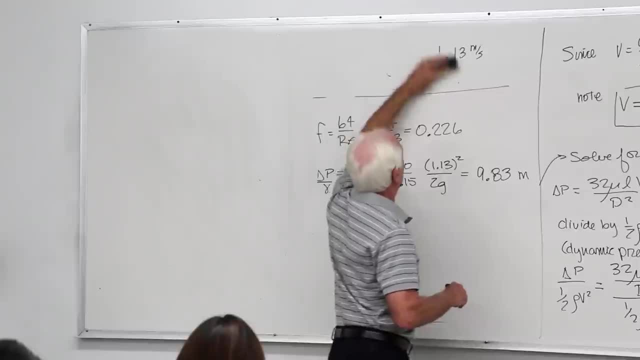 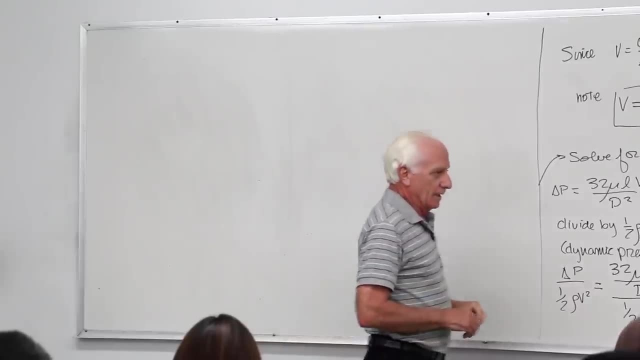 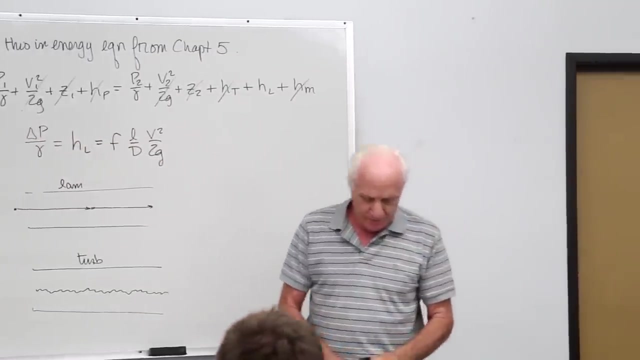 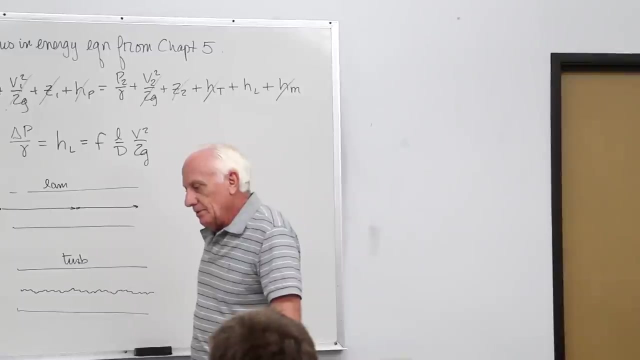 for lambda flow. No, it's very, very difficult, nearly impossible. So what they did is they took pipes, and it's described in here. They took pipes, and they different diameters, and they glued sand on the inside surface of the pipe. Now 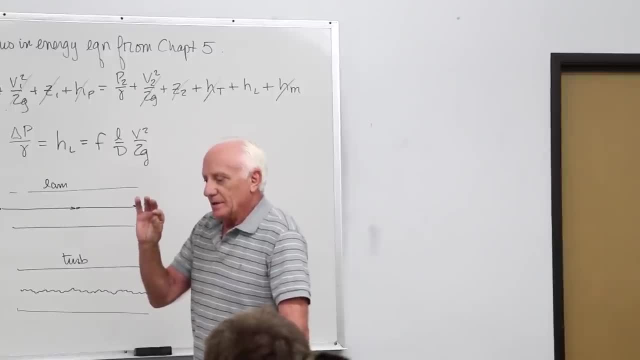 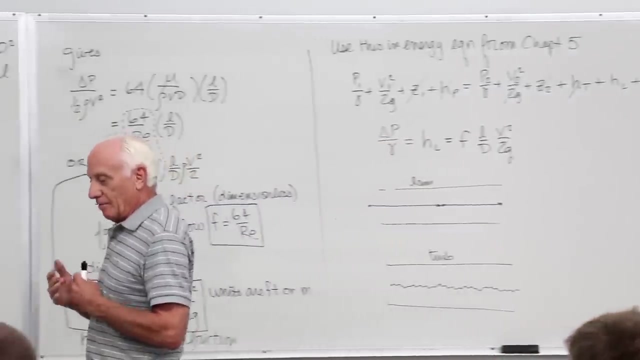 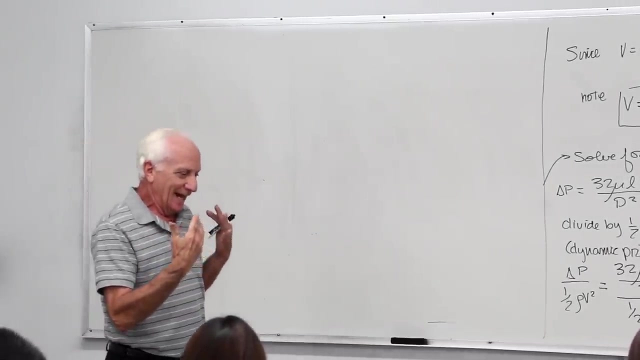 they glued very precise diameter sand particles- not random sand particles, very precise diameter sand particles onto the inside of a pipe to go to a rougher and rougher pipe, And then they made the flow turbulent And then they looked at the results of this pipe roughness. So they artificially 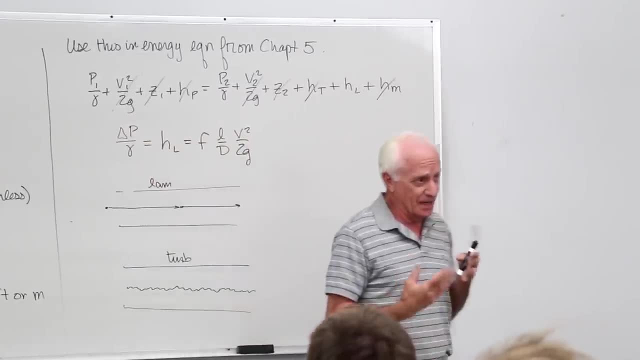 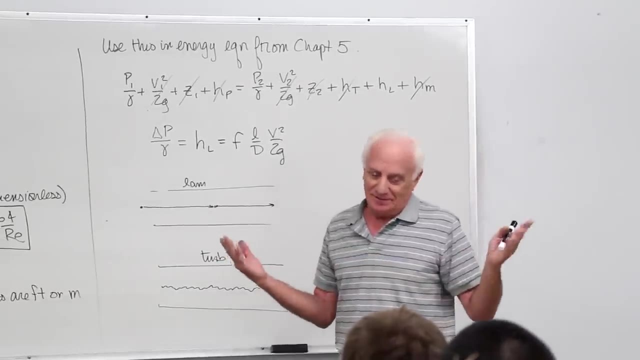 roughened the inside surface of the pipe with sand particles and glue. Imagine that. What a job that was for some of the graduate students. He got his- you know, tuition paid for. I'm sure So, but anyway, yeah, that's what. 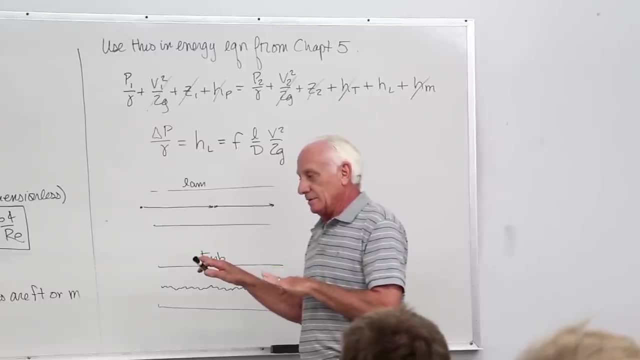 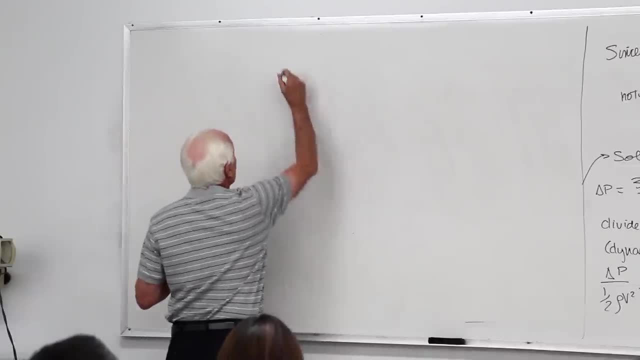 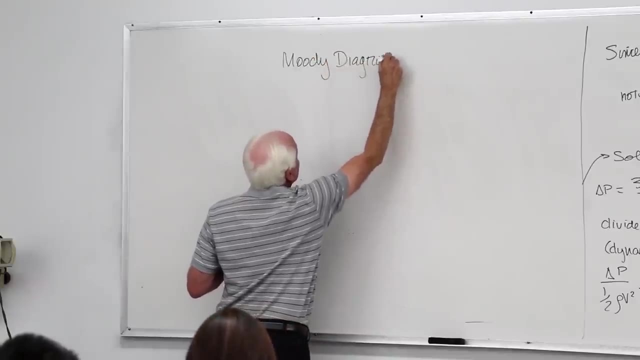 and different people massaged it. So what they did is they took all that data and different people massaged it. So what they did is they took all that data. they ended up with something called the moody diagram. now here's what the moody 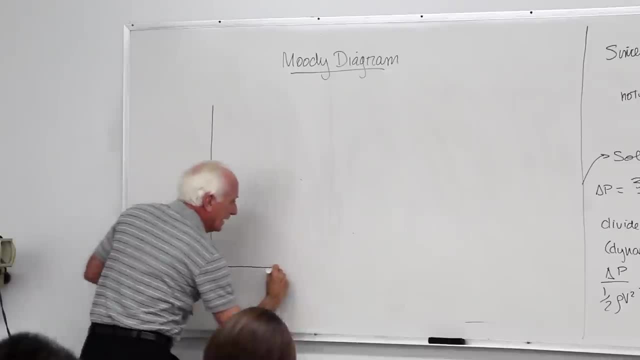 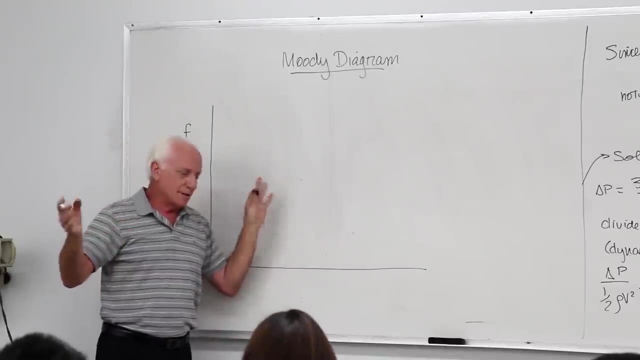 diagram is plotting on the y-axis. they're plotting the friction factor F. I'm going to give you one minute, I'll just throw the board now. so if you want to copy and have to, I don't copy anyway. that's the friction factor and this is 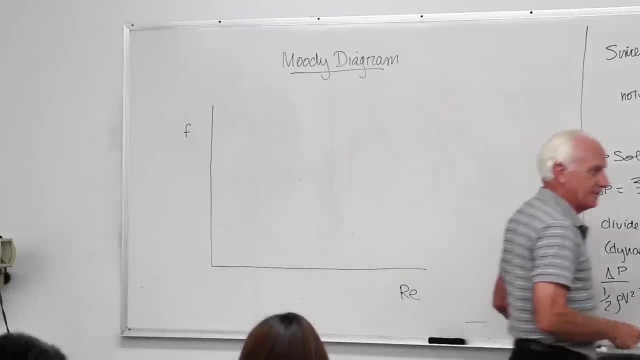 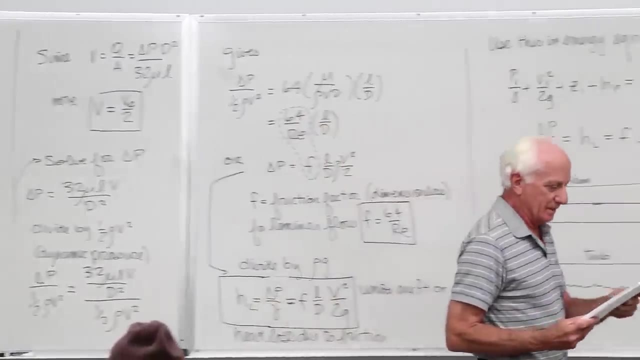 the Reynolds number. so maybe what I'll do is give it to you now so you can look at it. okay, I got one. all right, again, bring this back with you on Wednesday. so there's a moody. I'm going to just sketch on the board again, mention some things. 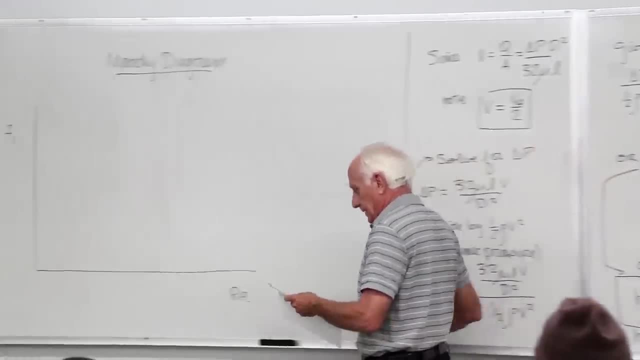 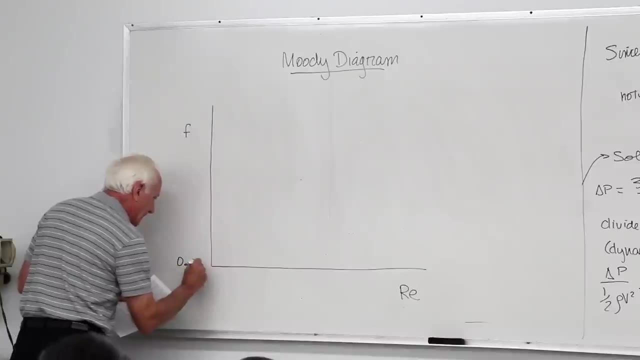 about it. we're plotting F on the x-axis. it starts down there at 0.008 and it goes up to 0.008. one zero. this is 0.01. yeah, okay, 2, 3, 4, 5, 6, 7, 8, 9, that's 0.0. Reynolds number 10 squared. 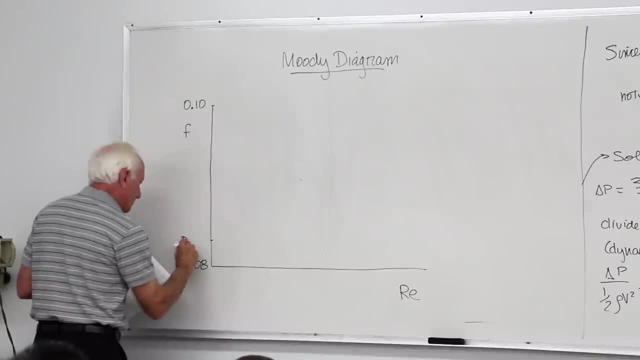 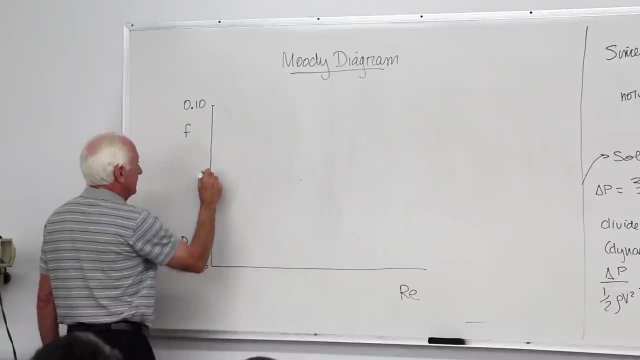 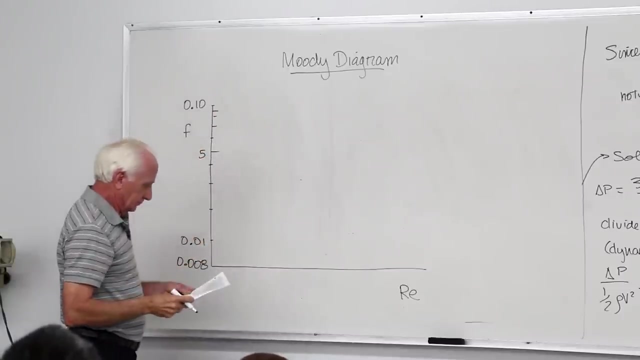 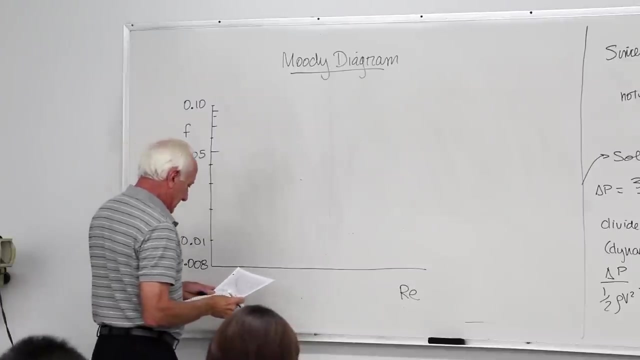 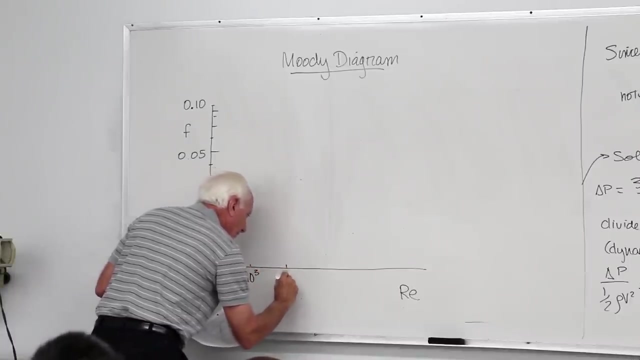 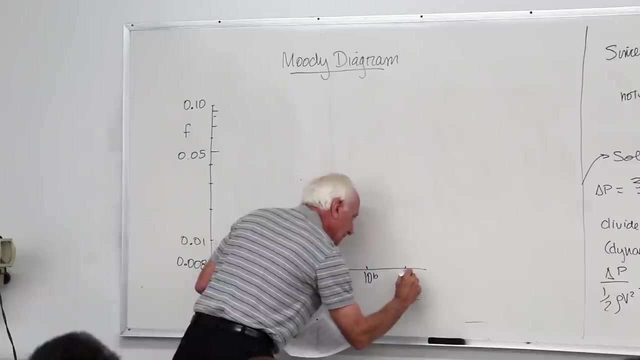 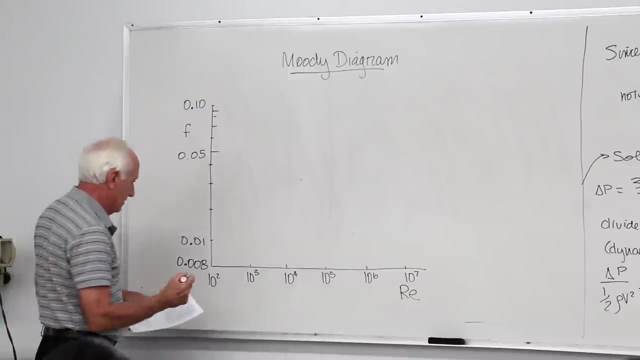 that's 0.01. yeah okay, 2, 3, 4, 5, 6, 7, 8, 9, that's 0.0. Reynolds number: 10 squared. I'll just start at 10. squared. third, fourth, fifth, 6. lavender flow out there roughly, doesn't 2100. here's a hundred. now this is a log. 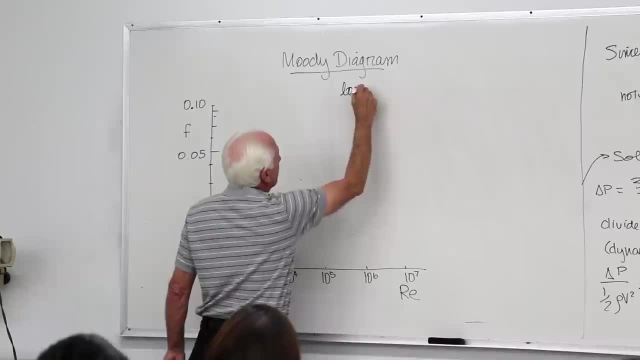 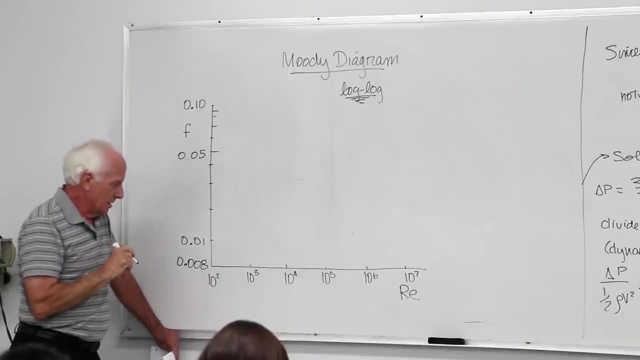 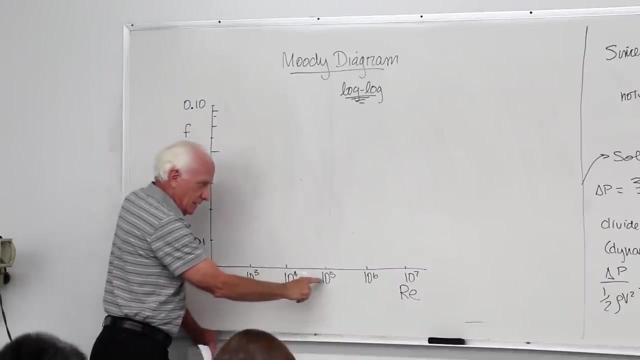 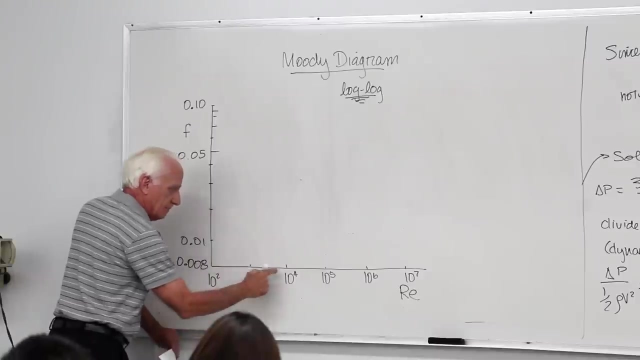 log axis. first log log axis. both axes are log log. so here's a hundred, a thousand, ten thousand, hundred thousand, million. okay, so lambda flow: 2100. two thousand, okay, ten thousand, two thousand, three thousand, four, five, six, seven, eight, nine, ten, about there, 2100. 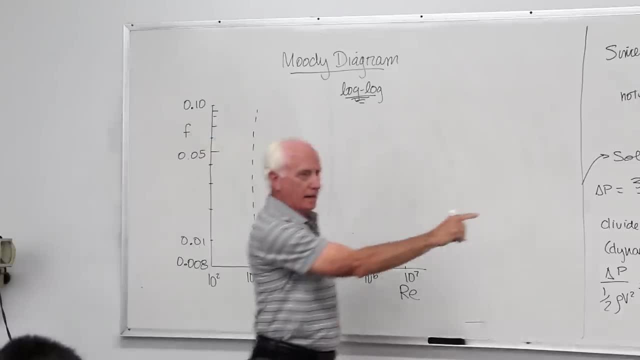 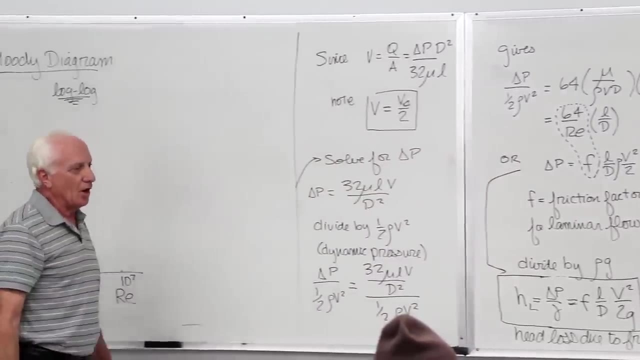 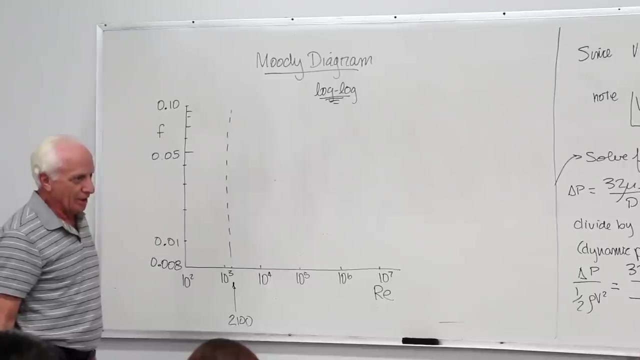 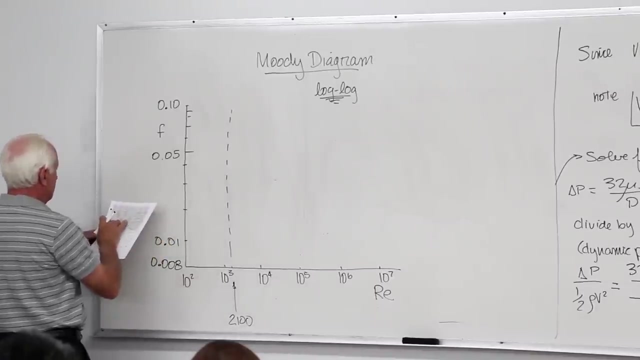 in that region and laminar flow, the friction factor is 64 over Reynolds number. when you plot that on log log axes, that's a power law. plot it on log log axes, guess what? you get? a straight line. okay, there it is here down to about point zero three. 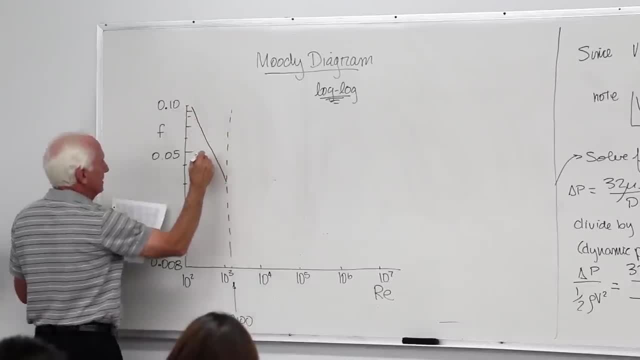 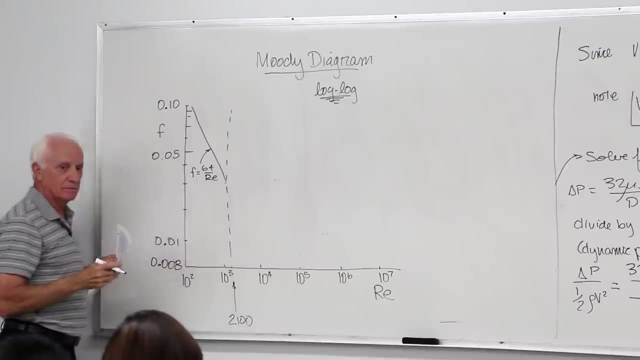 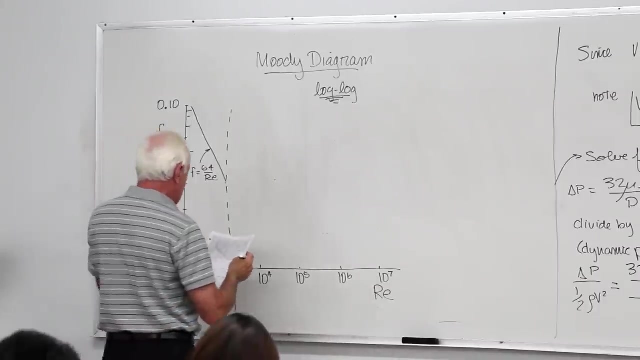 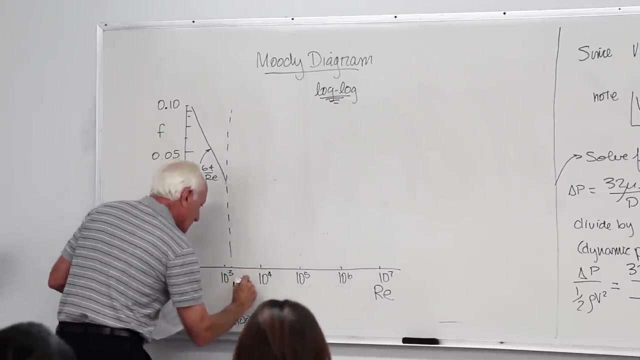 you. so there's a line F equals 64 over the Reynolds number, lambda flow. but now you see another family of lines and they start out up here at about 0.03, and this this is for roughly 4000. so this is 4000. 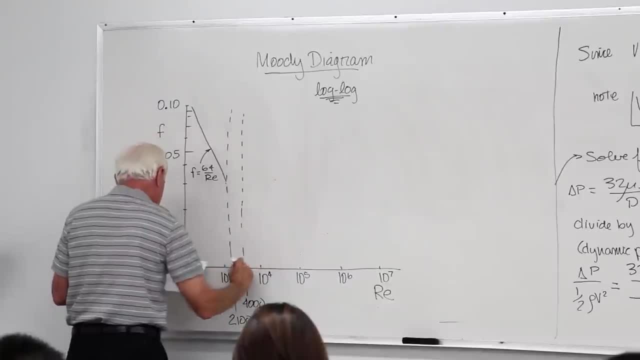 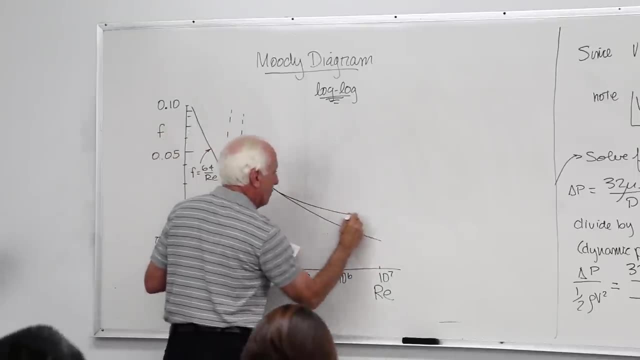 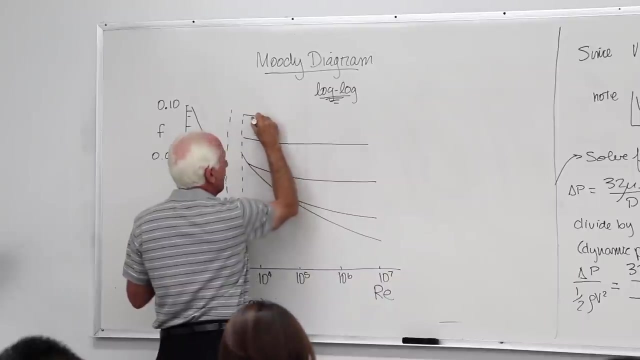 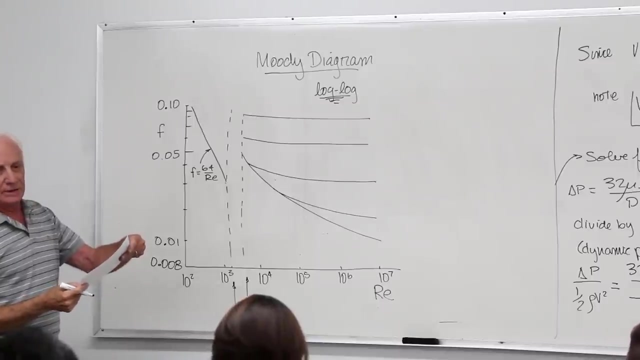 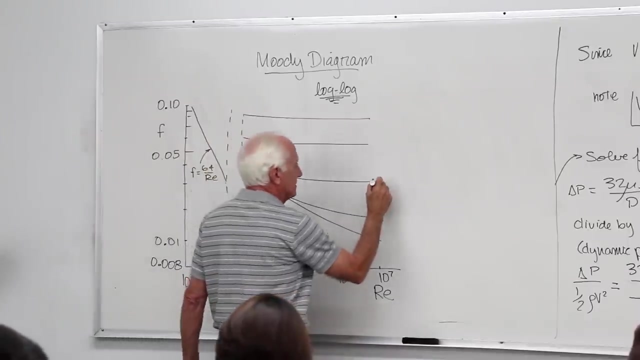 you, you lines go something like this. I'm just going to sketch them like this, And these lines are labeled on the right-hand axis. You can either say little e or epsilon. take your choice. I'll use little e. E over d. the relative roughness: e over d. 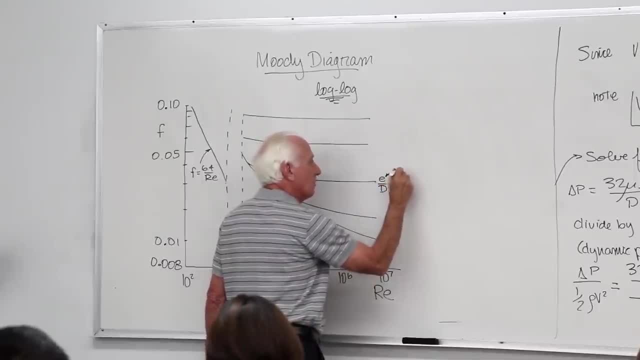 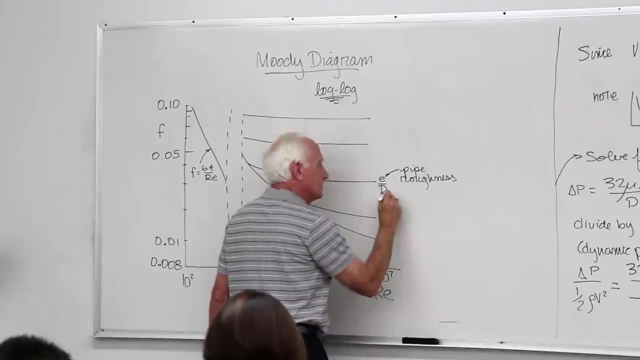 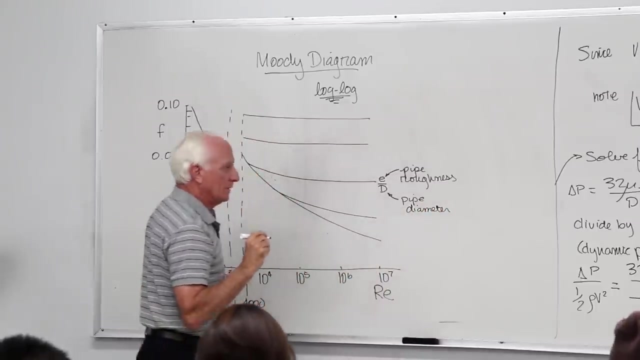 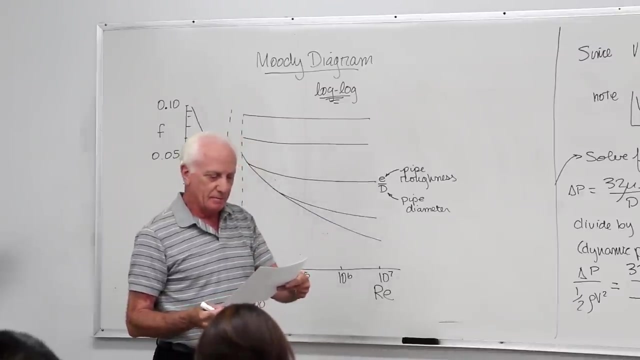 These lines are e over d. This guy is called the pipe roughness. This one, of course, is the pipe diameter. Where do you get the pipe roughness? In the little legend. In the little legend it says if the pipe is cast iron or galvanized iron. 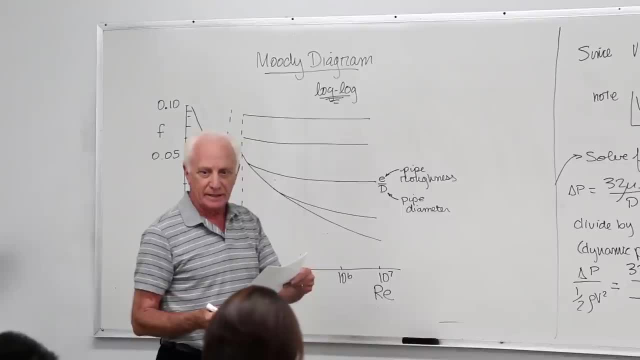 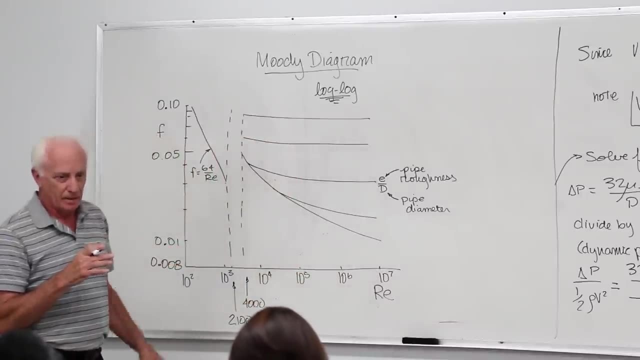 or drawn tubing or concrete. They give you the value of little e. So they give you the value of little e for different pipe materials. Notice concrete Really really rough compared to a rod-arm pipe. Of course concrete's rough. Take your hand and wipe your hand on. 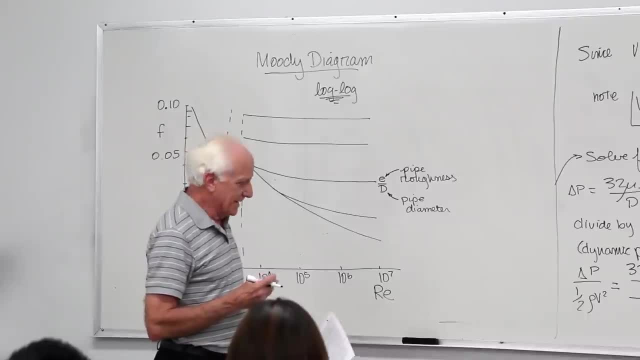 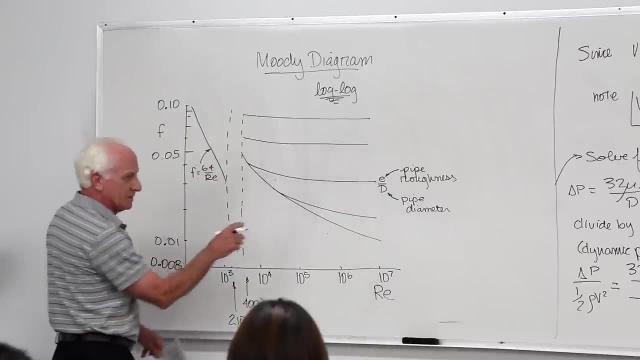 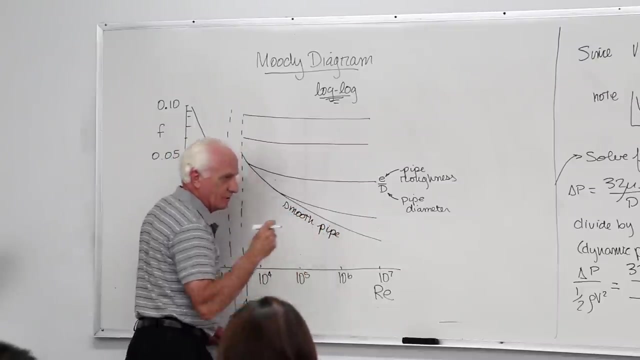 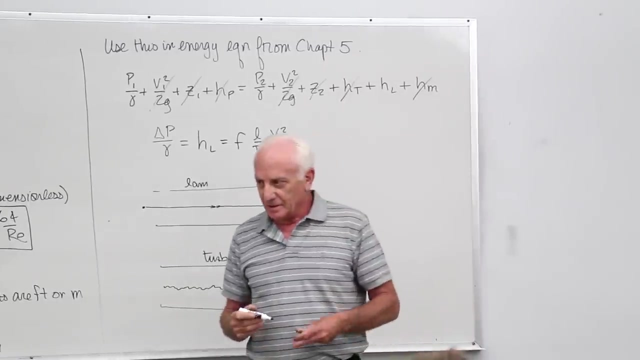 it. It's not good, It feels rough. Now take your hand on a PVC pipe. Rub it along the PVC pipe. Wow, is it smooth. Copper, Wow is it smooth. This line here is called the smooth pipeline. PVC can be approximated most of the time as smooth. 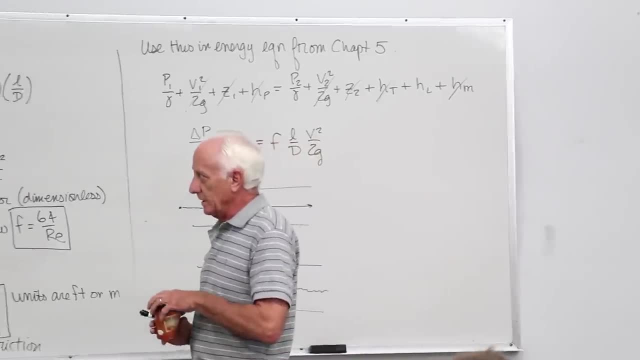 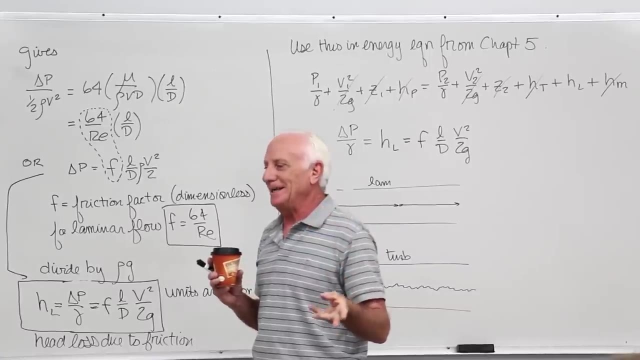 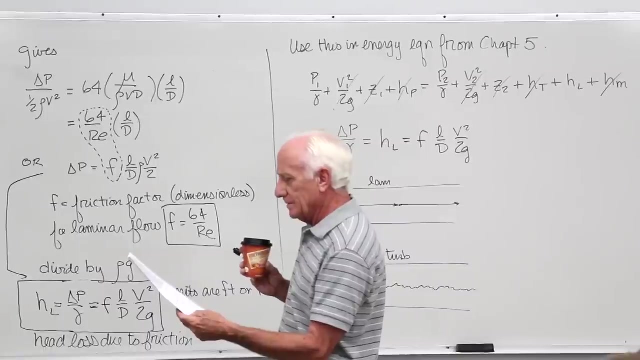 Drawing copper tubing can be approximated most of the time as smooth. There's a little bit beyond that. they call hydraulically smooth, But normally in this class if you hear something like PVC or copper, look at drawn tubing. Oh my gosh, what are they? six zeros. 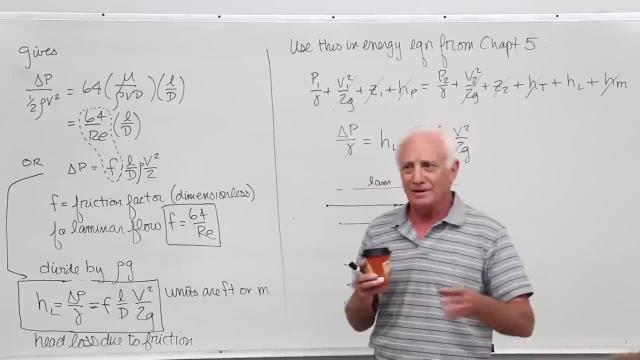 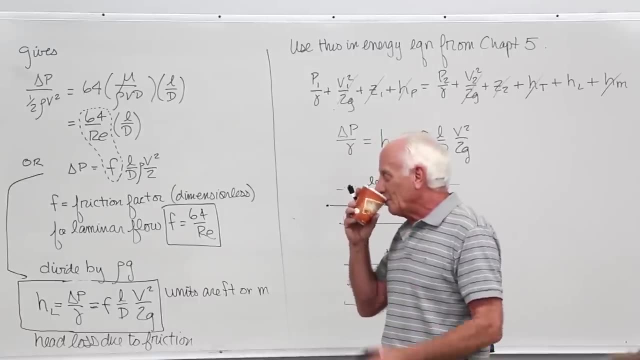 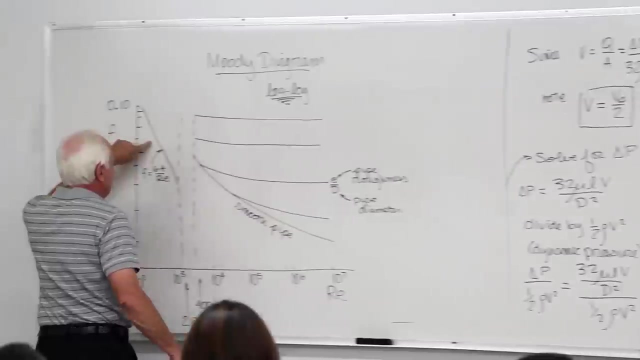 and a five feet. Yeah, it's really pretty smooth. So, yeah, we're going to assume a pipe like that is smooth, yeah. So how'd they get those lines like that? Now don't forget, they got this one over here, They got this one from theory, These guys, they didn't get. 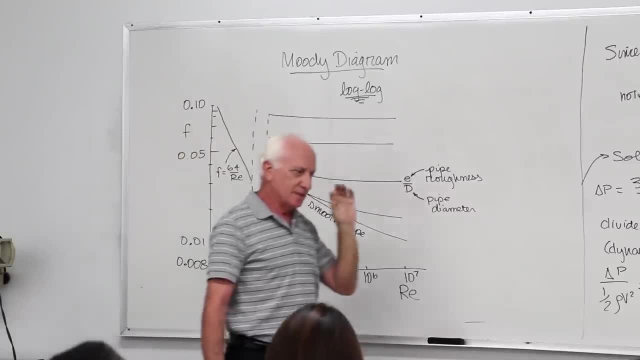 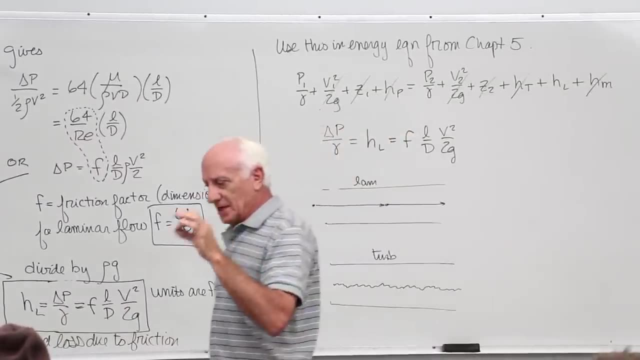 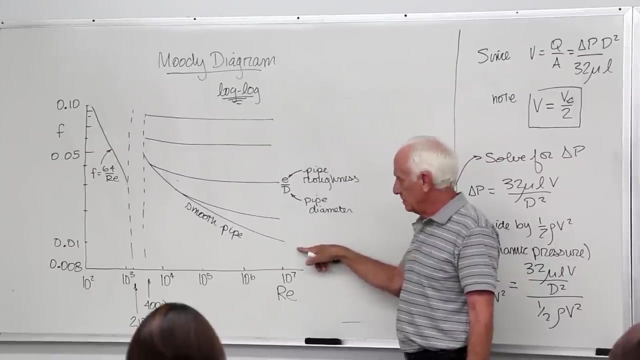 from theory. They got from doing what They got from doing what They got from doing what Gluing sand particles very carefully on the inside of a tube, And the bigger the sand particles were, the rougher the tube was. This is high roughness. This is no roughness. 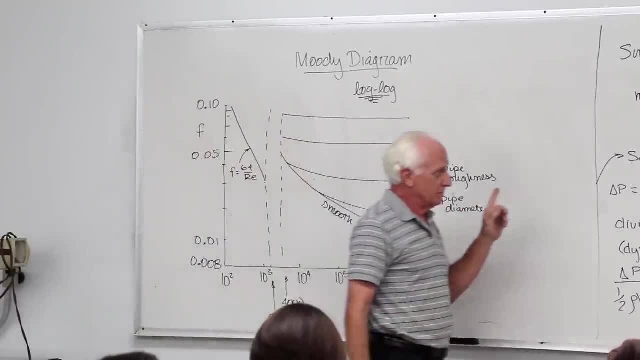 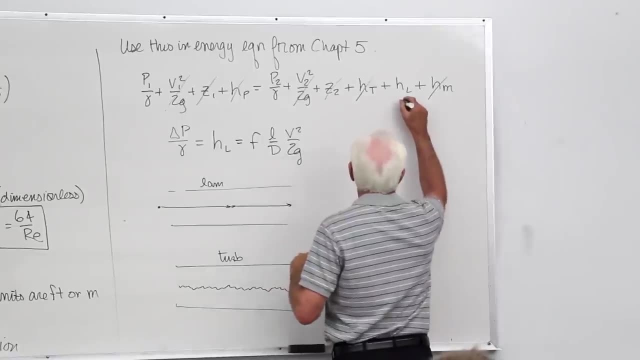 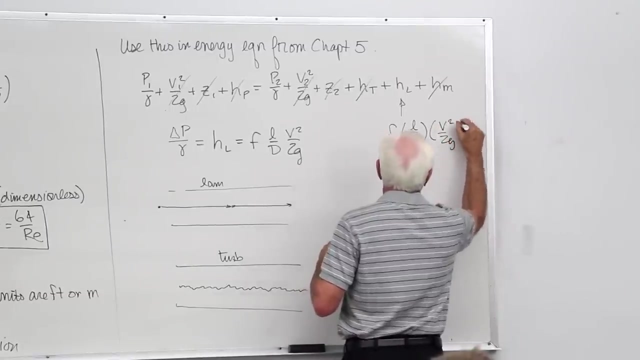 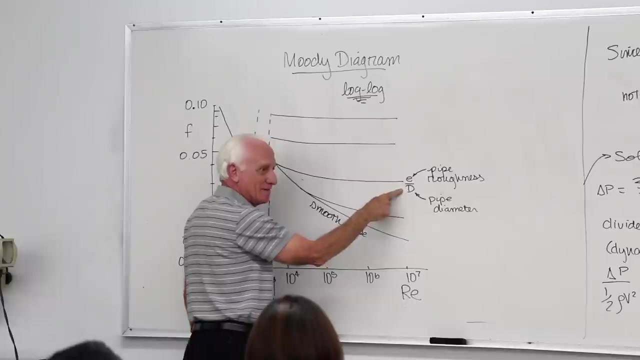 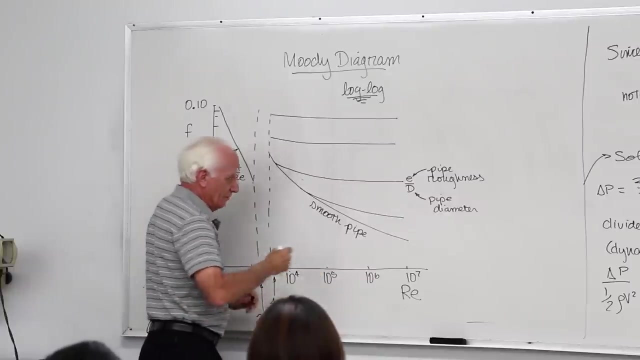 So if we want to get F in turbulent flow- to put this equation right here or up here- then we have to get the relative roughness, divide it by the diameter, find what line we're on, get the Reynolds number, go up here with the Reynolds number until you find out. 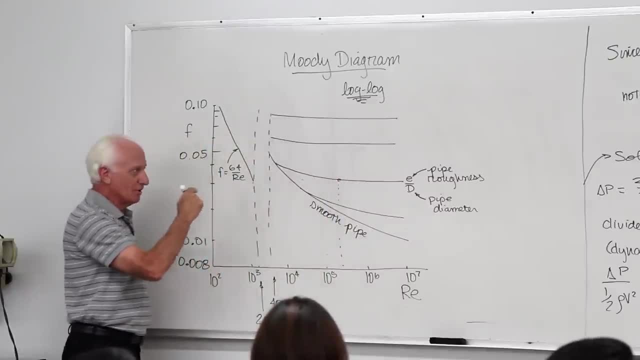 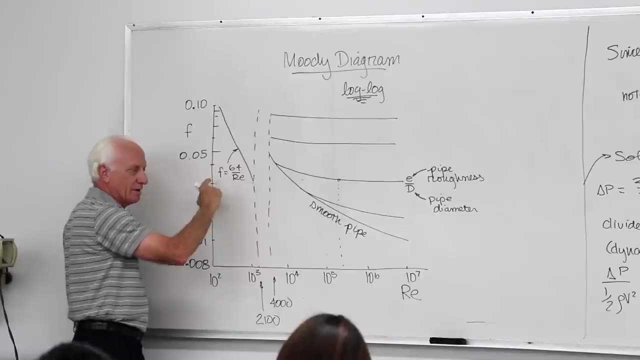 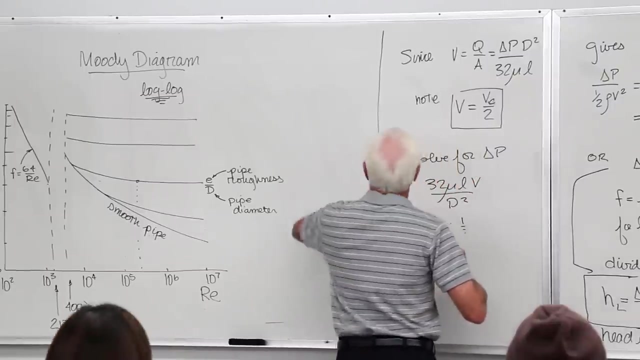 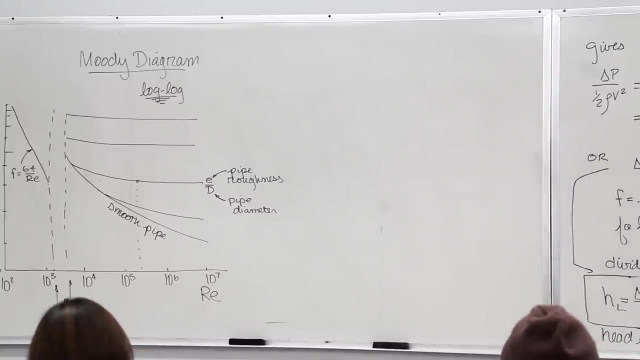 what line you're on, Then go across horizontally until you get the relative roughness. So that's the value of the friction factor. So we get to the F axis, and that's the value of the friction factor. Okay, Now let's see. Just for your own information, I gave you three examples. 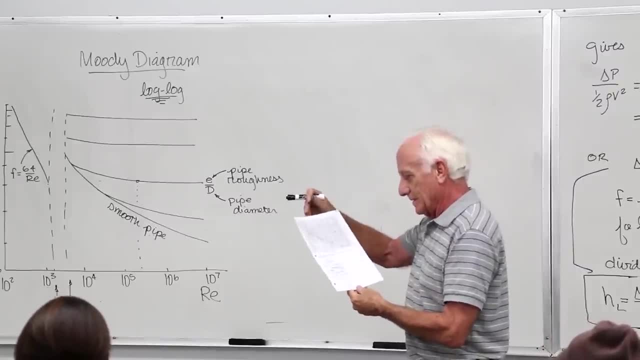 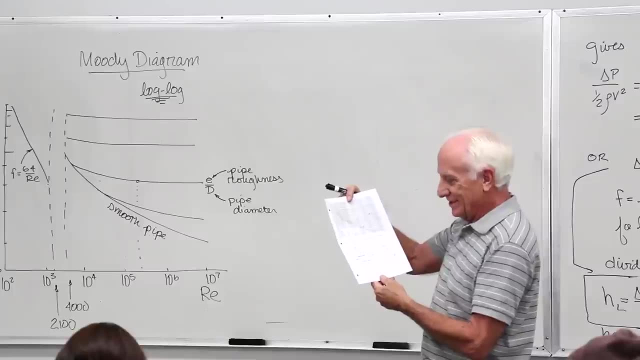 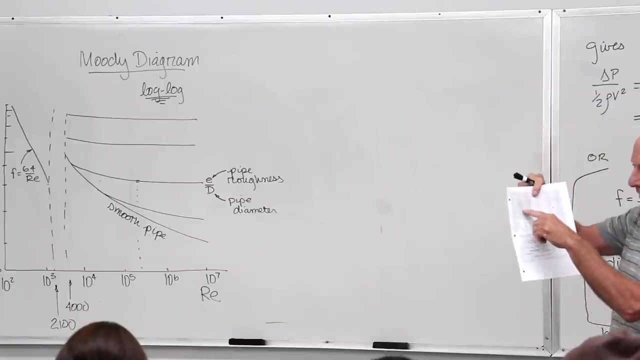 on the bottom of that page with a woody shark on it, to make sure you're reading the woody shark correctly: One is for a galvanized iron pipe, One's for a riveted steel pipe, The other one's for a drawn tubing pipe And I got the points labeled there to show you. on the woody shark. 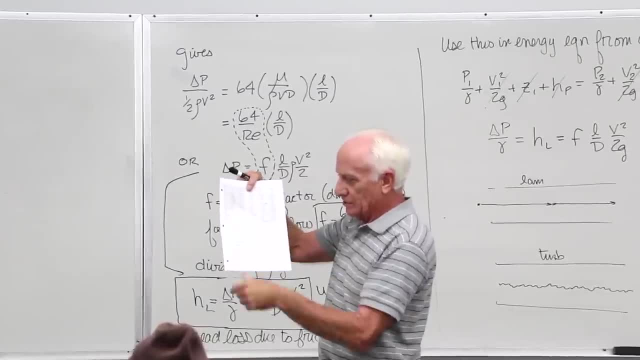 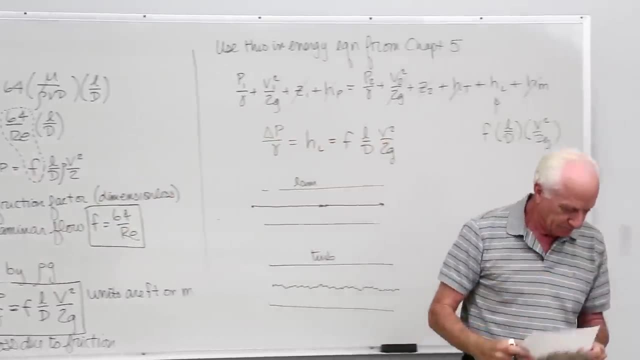 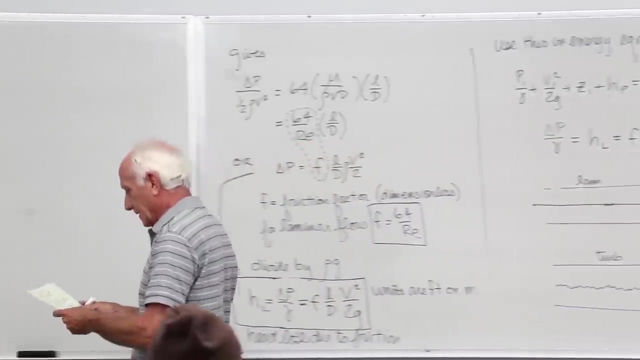 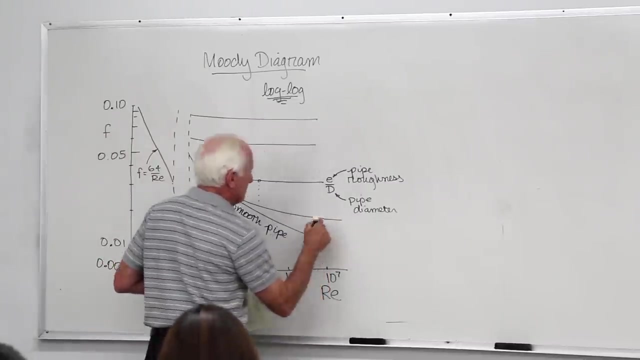 where those points are, to give you the friction factor in the left-hand side of the page there. So that's examples of how you get the friction factor. Okay, This is called. now You can see where it starts to be flat. It starts to be flat out here. 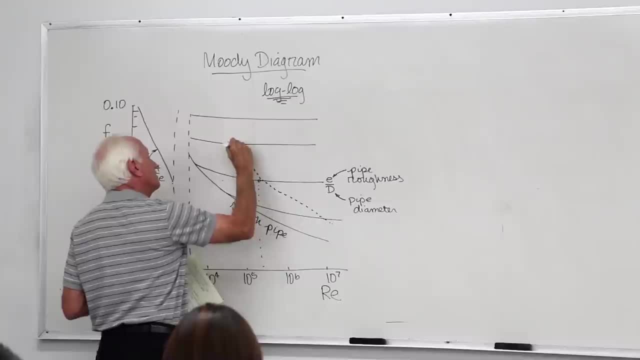 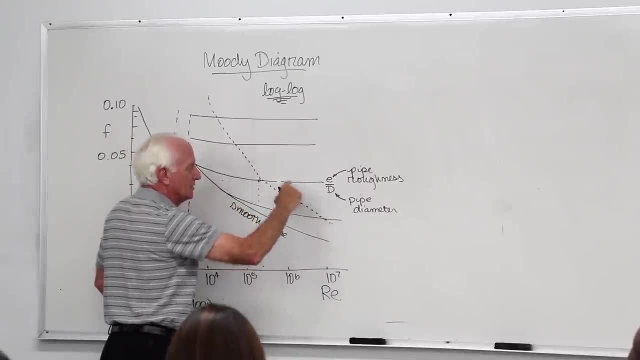 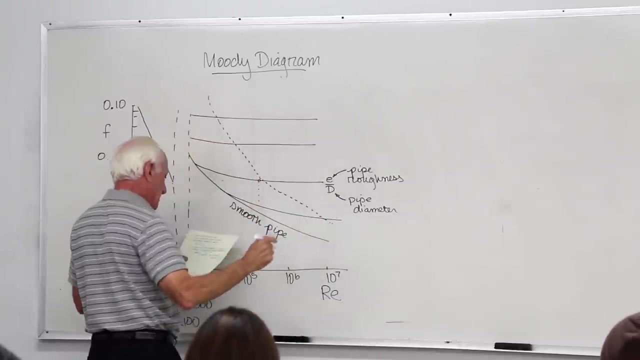 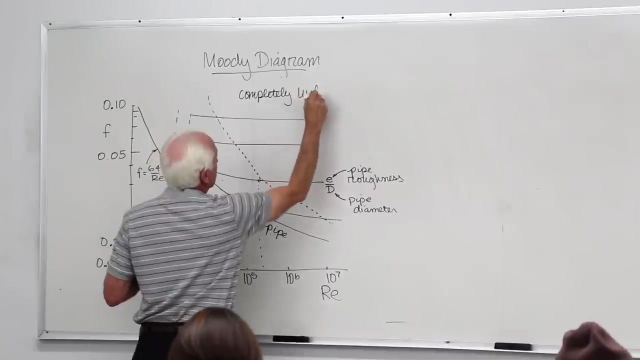 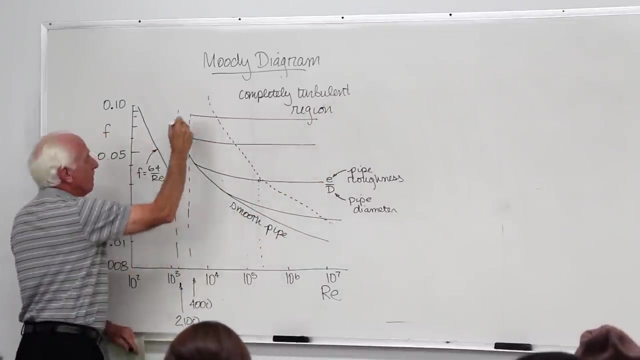 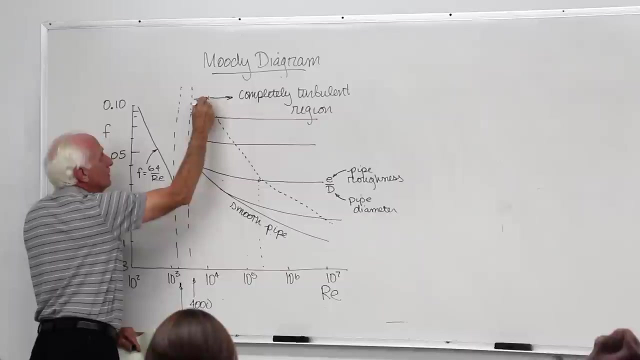 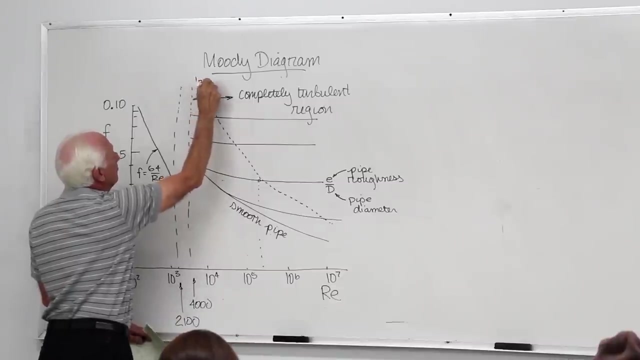 You can draw a dash line here. This is where it starts to be flat, Everything to the right of that dash line. these lines are horizontal, Horizontal. This region is labeled in our textbook completely turbulent. The region to that side line. The region from here to here is labeled transition: The transition region. 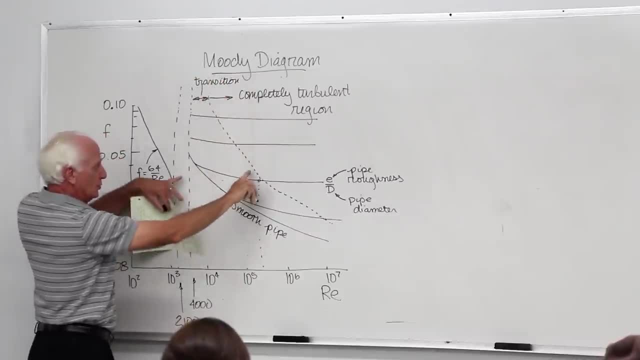 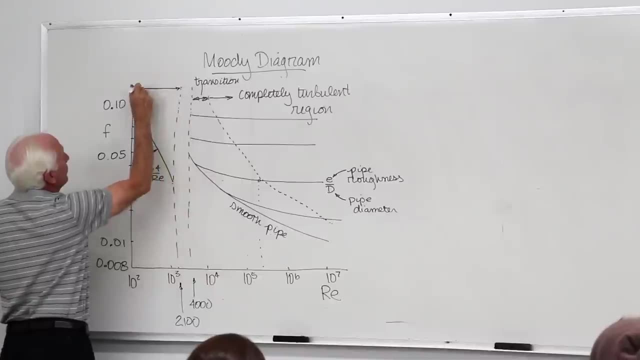 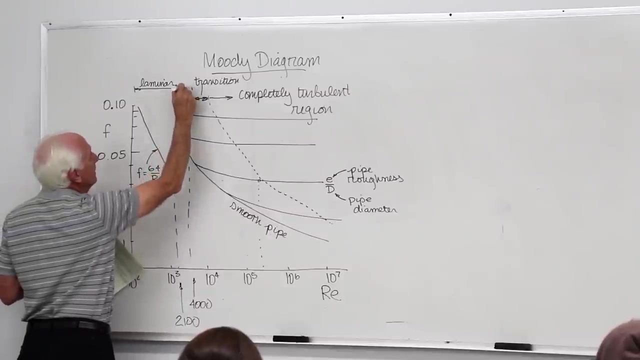 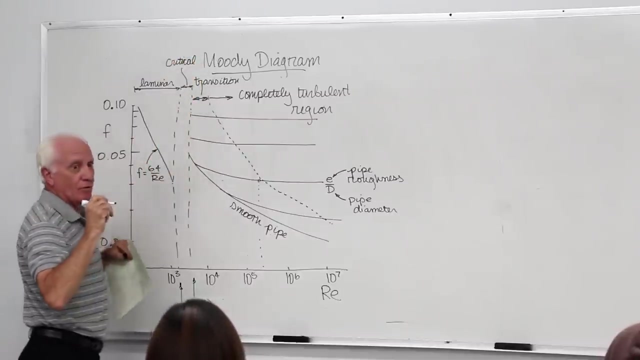 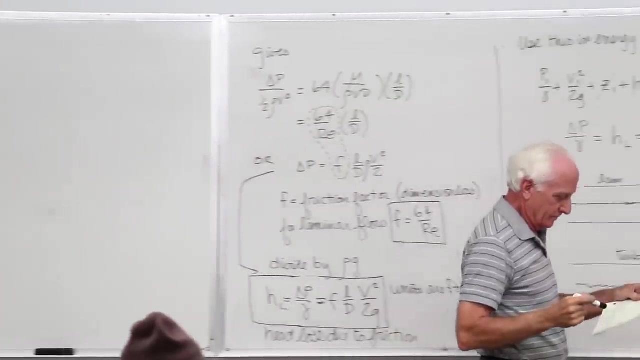 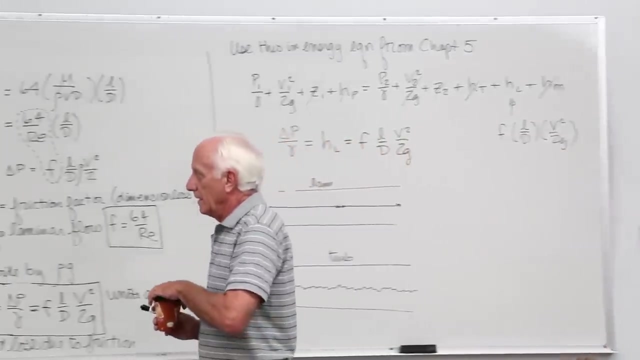 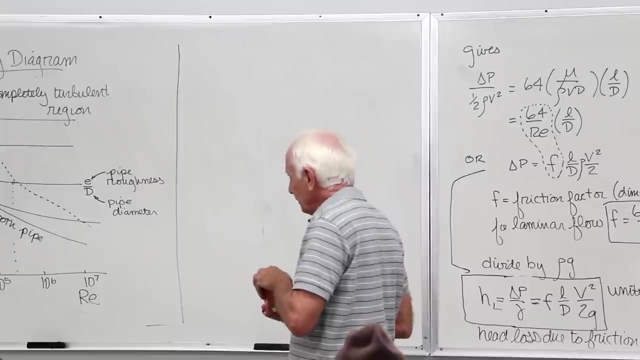 between these two dashed lines. transition region, the region from here to here. of course. laminar, the region between these two guys from here to here. critical. so there are four regions of the moody diagram, four regions of the moody diagram. you wouldn't need the moody diagram for laminar flow because it's don't ever use. 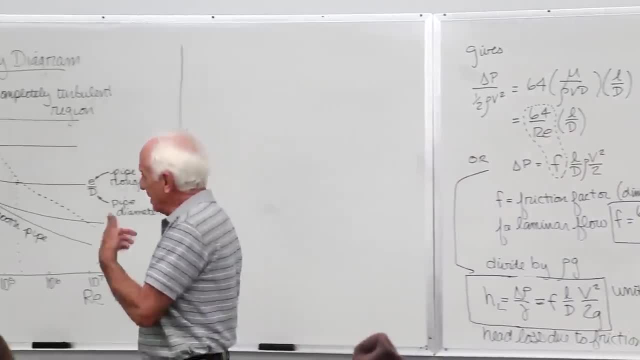 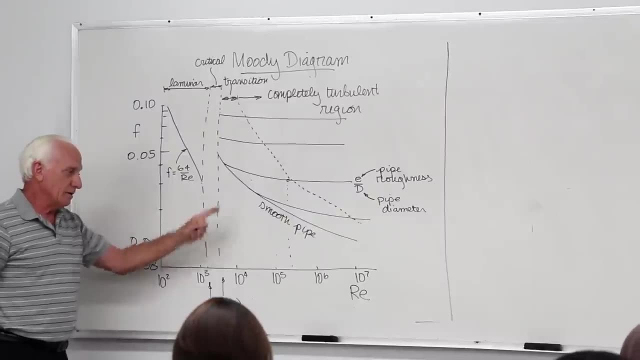 the moody diagram for laminar flow. do it mathematically: 64 divided by roughly 64.. number- oh, he's reading that log log chart. but where you need it is over here of course, or you can find some curve fit equation that might work to get F as a. 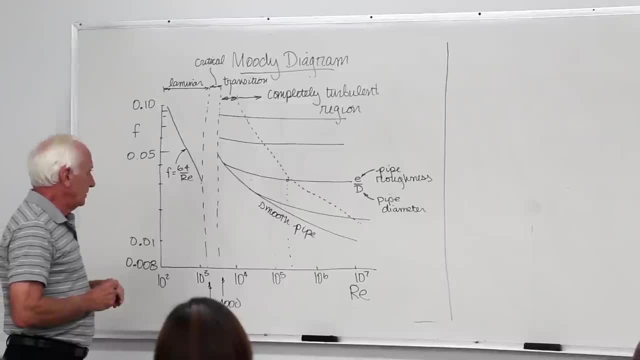 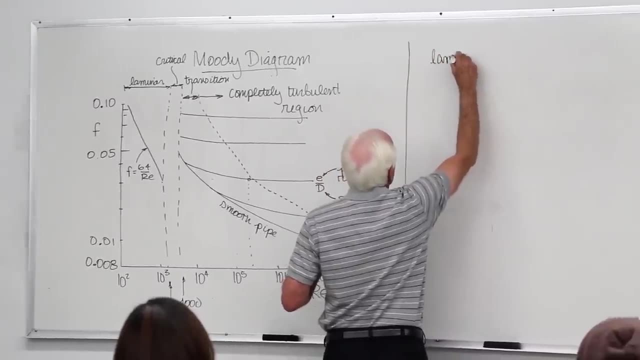 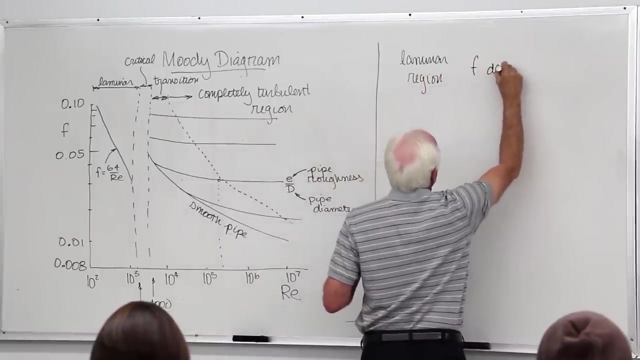 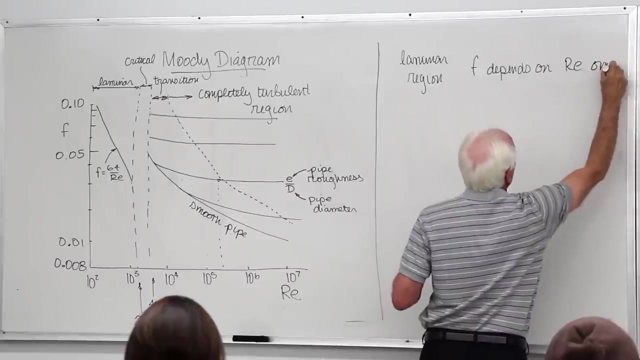 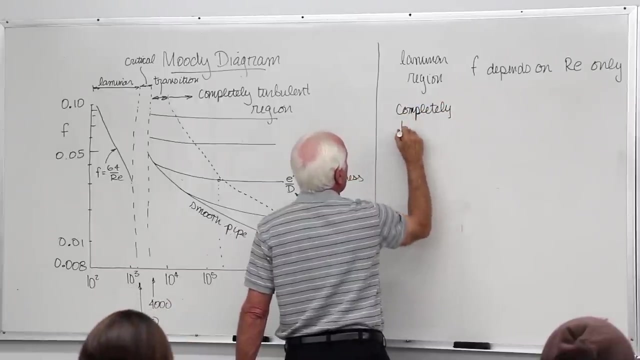 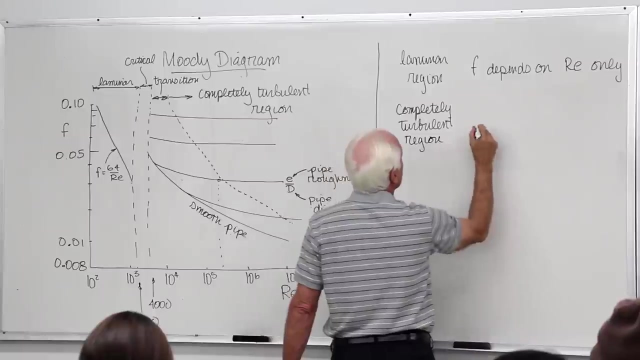 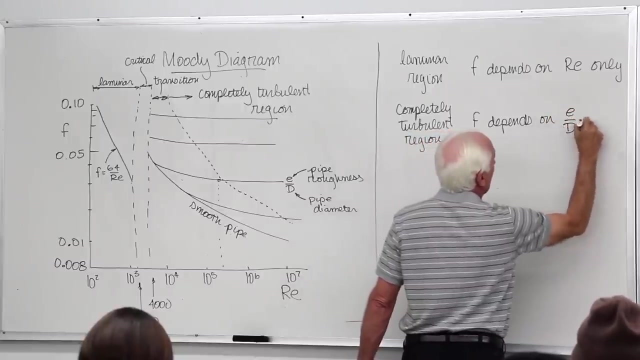 function of different things. okay, so let's say you're in the laminar region, F depends on the Reynolds number only. let's say you're in a completely turbulent region. F depends on E over D only F depends on E over D only we covered very well. I'll come back to that in a second. 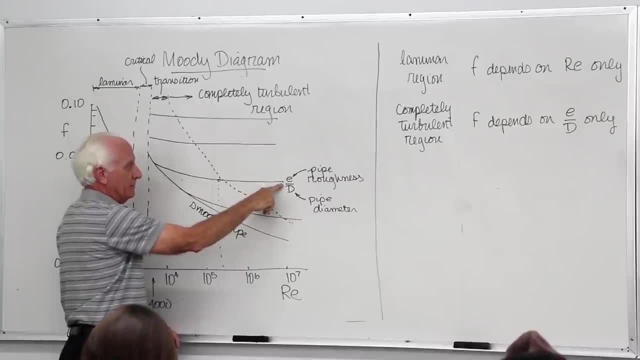 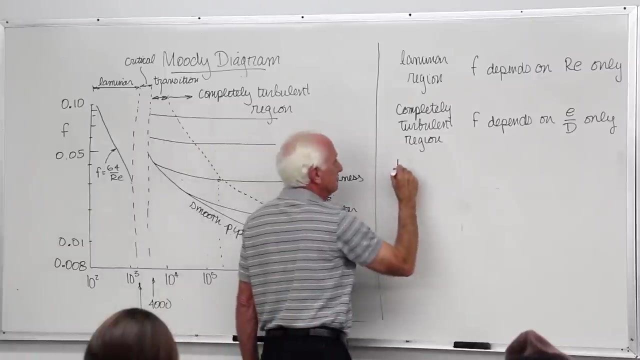 on the other side, off with some weight on the T and R. okay, now you get all the punishments. you learn more about time valve Viking one, like right here. that belly of F won't change along here where it's horizontal. and what's that region called words horizontal, a completely turbulent. 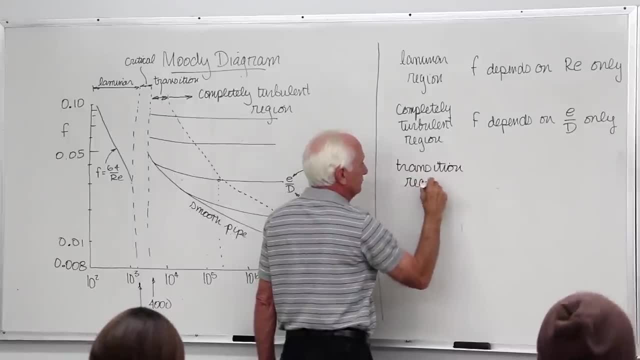 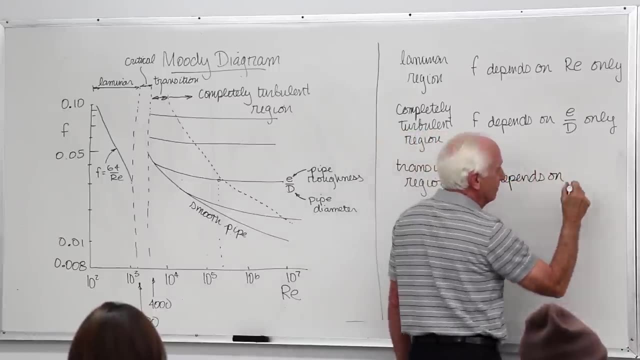 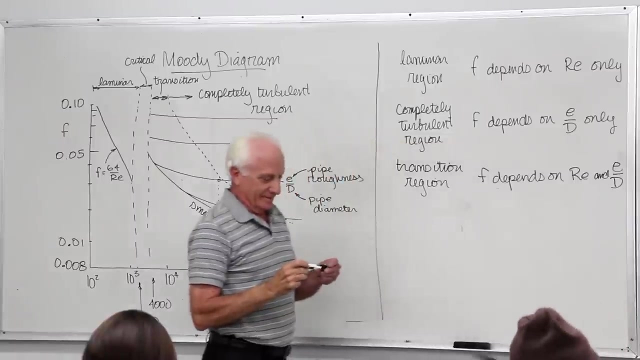 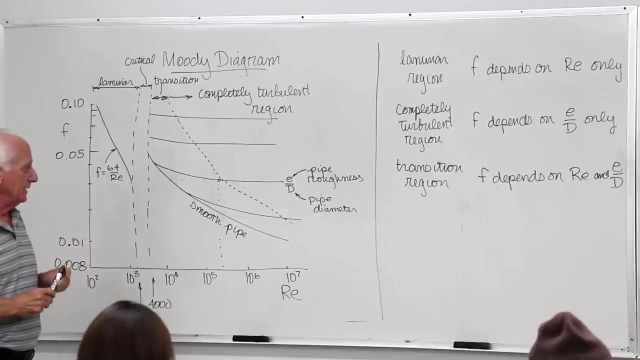 region. now tape the transition. F depends on: okay, now it depends on Reynolds and E over D. Okay, It depends on both things: the Reynolds number and the relative roughness. E over D is called the relative roughness, It's dimensionless. F is dimensionless, The Reynolds. 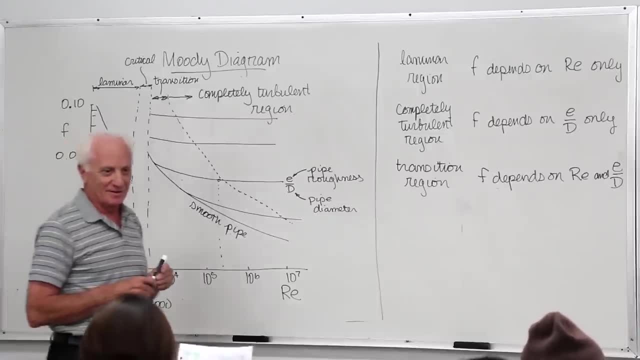 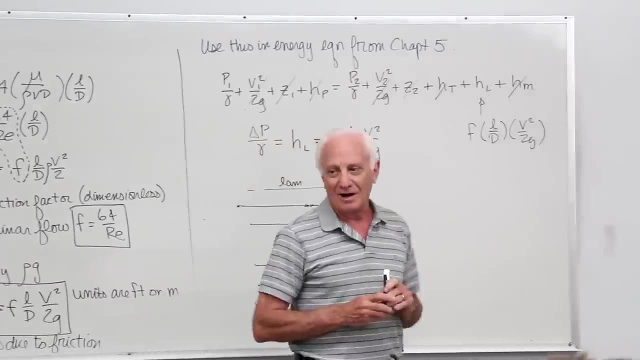 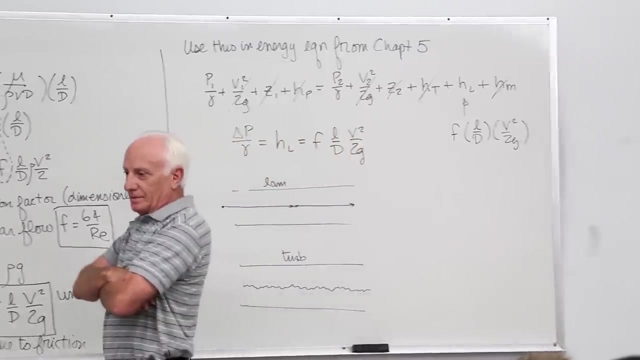 number is dimensionless. This is a dimensionless chart. We engineers love dimensionless charts In fluid mechanics and heat transfer. wow, there must be 25 or 30 dimensionless parameters: The Nusselt number, the Stanton number, the. 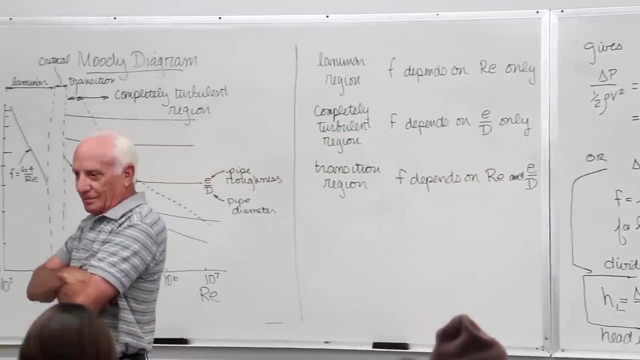 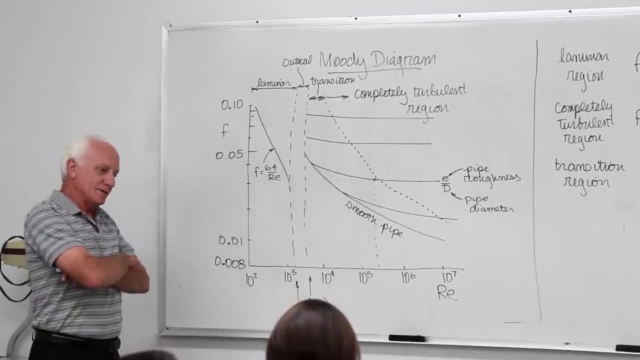 Weber number, the Poisson number, the Reynolds number, blah, blah, blah. the friction factor, the relative roughness, Those are all dimensionless parameters. So this is a dimensionless number. This is a dimensionless chart plotted on log-log paper. Sometimes people have a 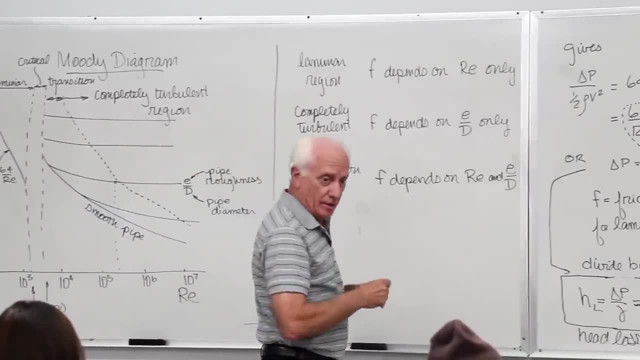 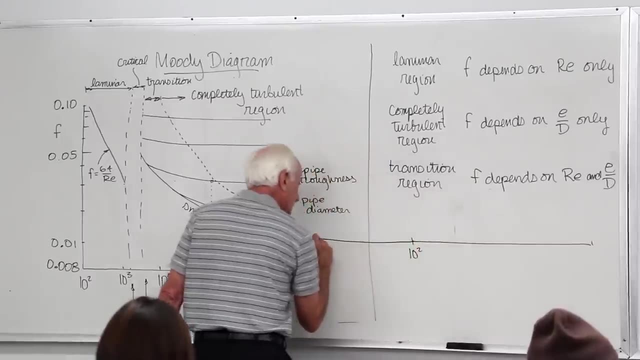 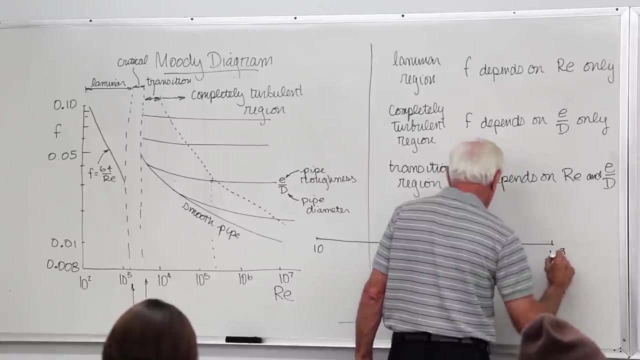 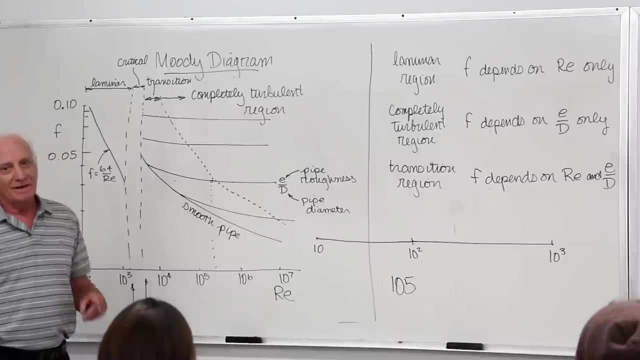 lot of difficulty reading a log-log axis. So if this is 10 squared and this is 10 and this is 10 cubed, okay, find 105.. Reynolds number 105.. Because if you can't read this axis, you're not going to get the F value right. 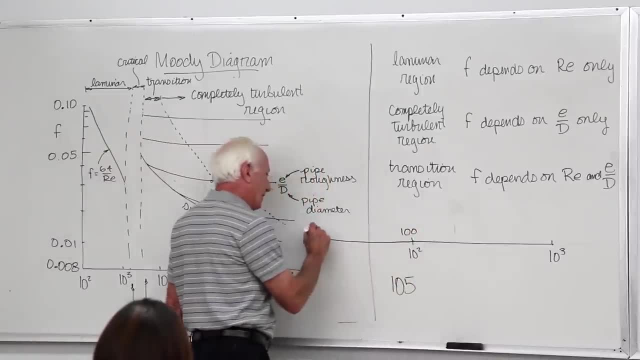 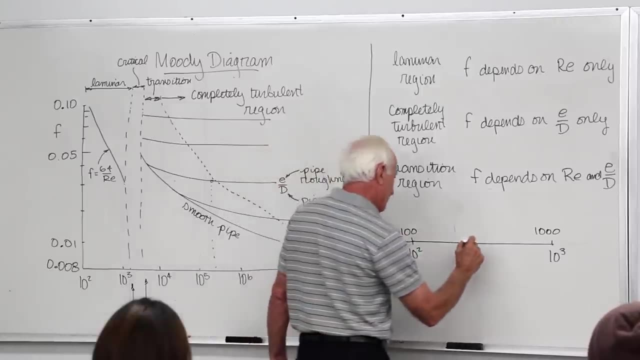 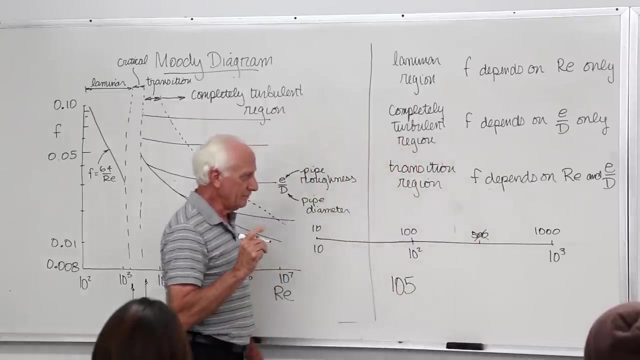 105.. What's this one 100.. What's that one 10.. What's that one 1,000.. Now, don't say this: I think 100 and I think that's 500.. No, no, Here's what it is. If you. 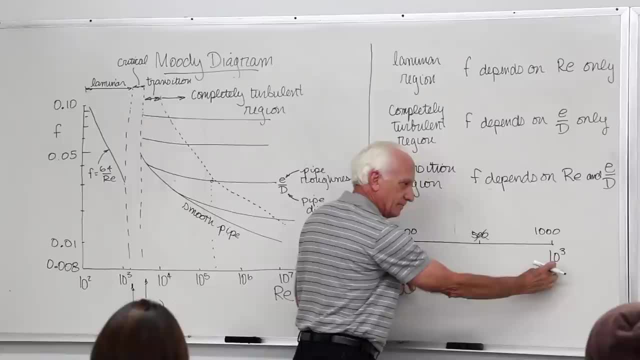 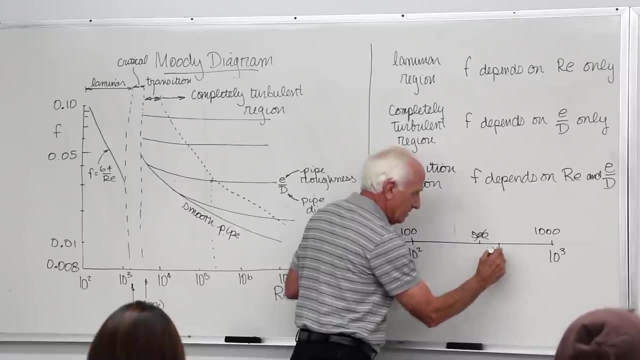 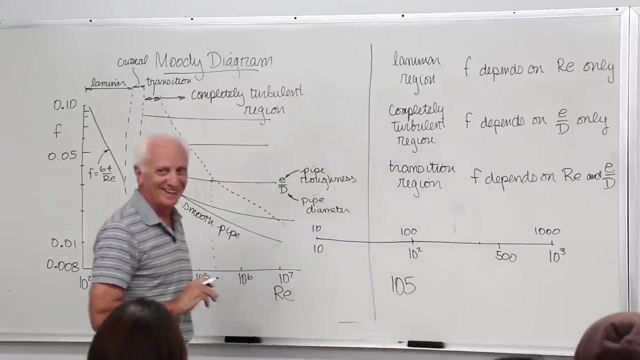 take the distance from here to here. take a ruler and measure this distance And take 70% of it. You got that 70% of it. That's what 500 is. Don't think linearly, Think logarithmically. That's how the scale's made. from log There's 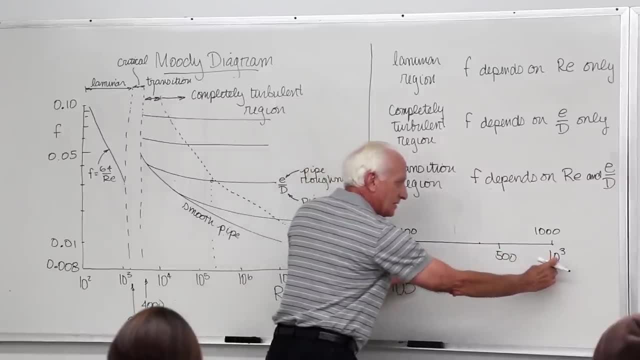 500.. It's not in the middle. No, it's 70% of the distance between my two fingers. That's where you put the 5 times 10 squared. That, by the way, is 500.. That's where you put the 5 times 10 squared. That, by the way, is 500.. That's where you. 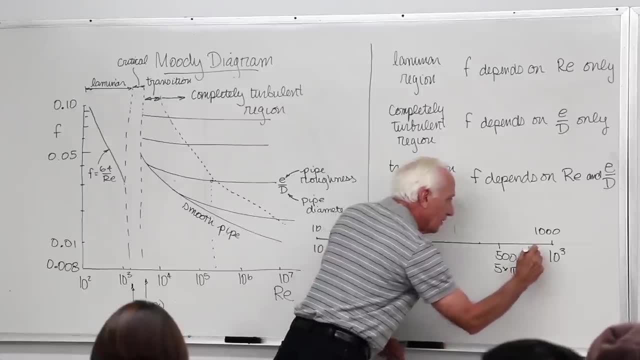 put the 5 times 10 squared. That, by the way, is 500. That, by the way, is 500. That, by the way, is 5 times 10 squared. Where is 9 times 10 squared? 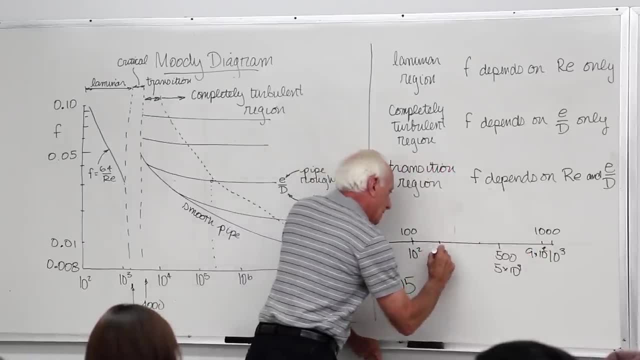 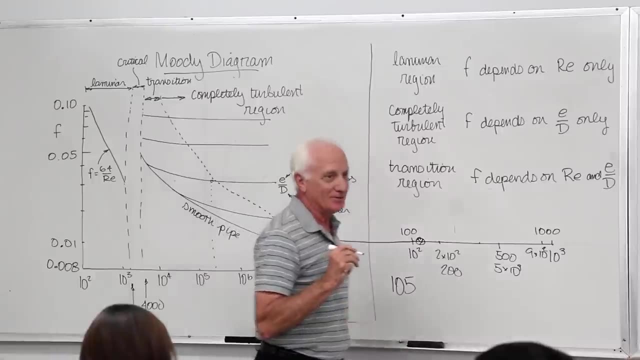 There. Where is 2 times 10 squared There? What's that 200.. Where's 105?? Right there, And boy, you better read those guys right. It's not rocket science, you know. It's not calculus, no. 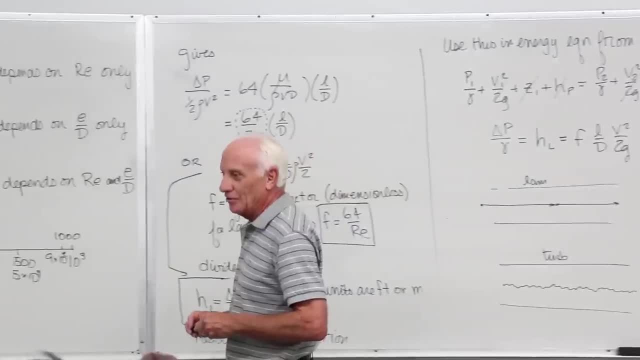 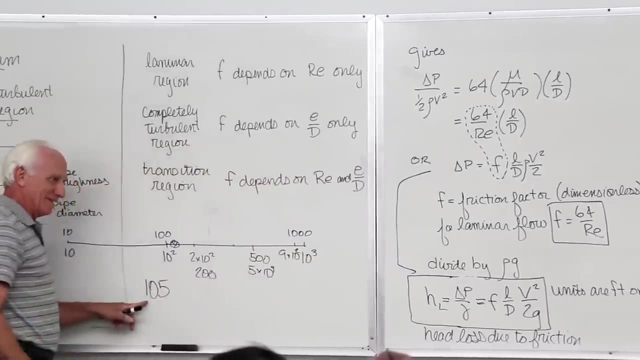 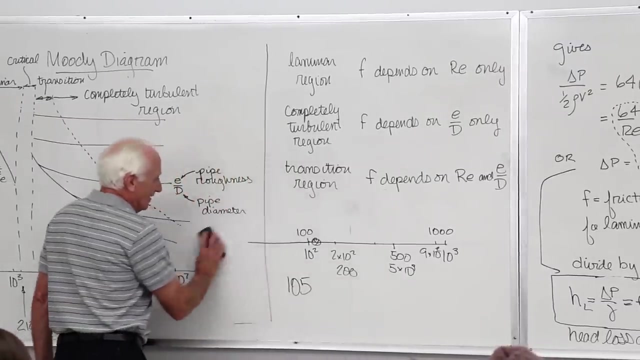 Not DPQ, no, It's. how do you read a log scale reasonably, reasonably accurate? So be careful. Some people, when they get numbers like this, they really have a problem reading those scales in your hand. Okay, Let's go back to here now. 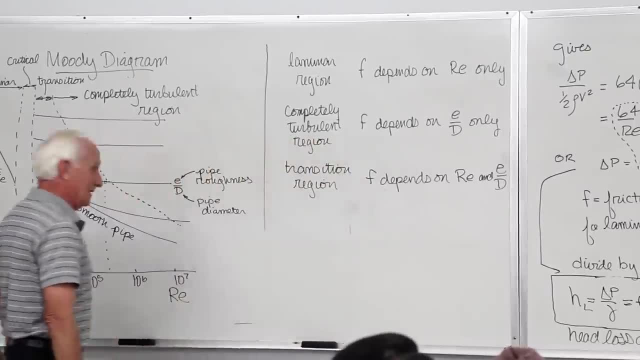 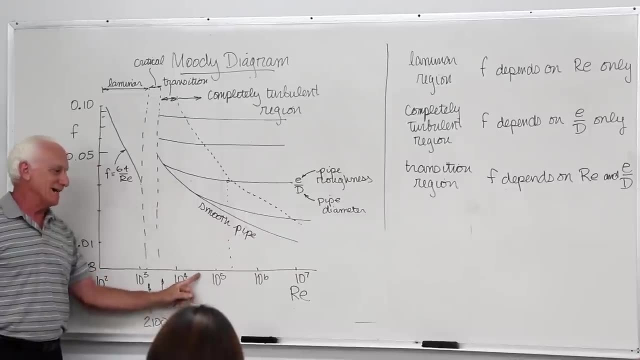 Is it serious? Oh, it's big time serious on a smooth bike: Very steep curve, Very steep curve. If you're offering this guy down, some people think, okay, this guy's going to go down. Okay, 110,000, 1.1 times 10 to the 5th. 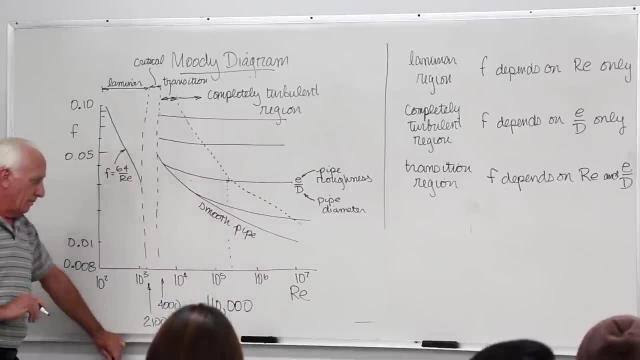 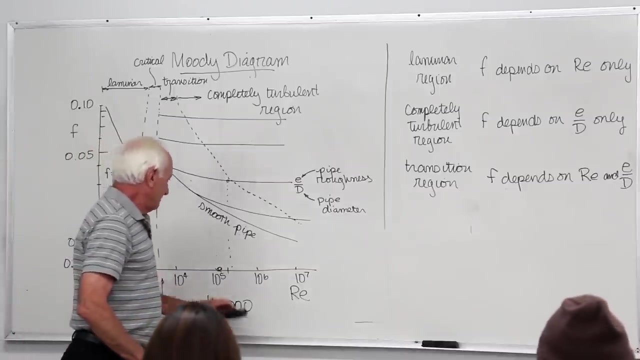 There's 2 times 2 to the 5th. Okay, Right there. There, it is Right there. So be careful. It can really get you if you're not careful. All right, I didn't do the critical region yet. 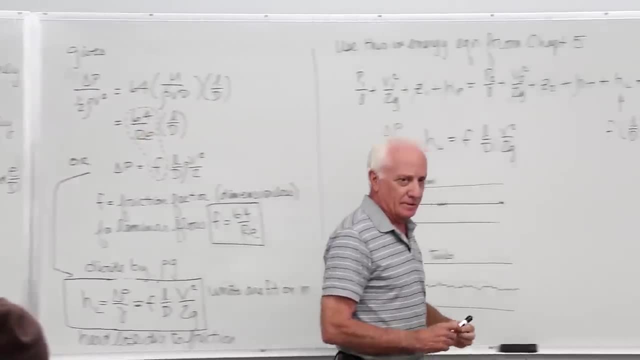 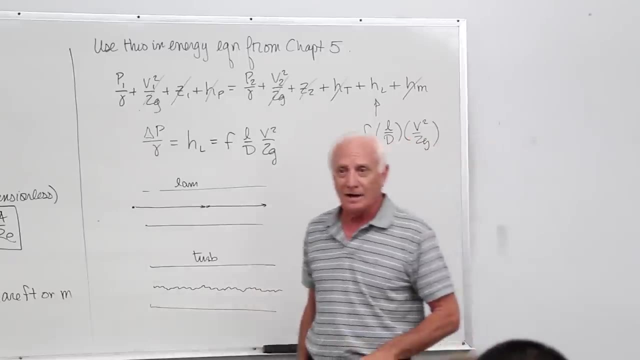 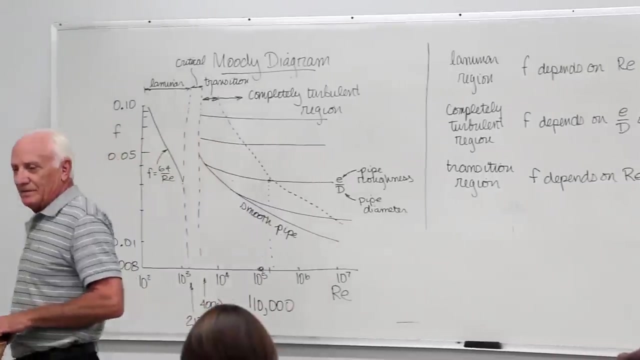 I didn't do critical region. No, I didn't do it and I'm not going to do it. look at the moody chart. what do you see there? i see a blank region. there's nothing there. the lines end, that's right, the lines end. well, what does that mean? that means: don't even attempt to get. 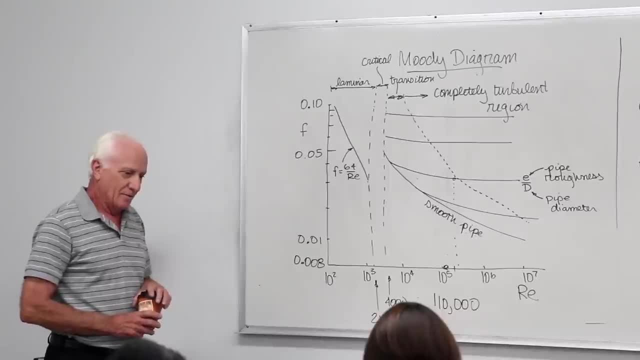 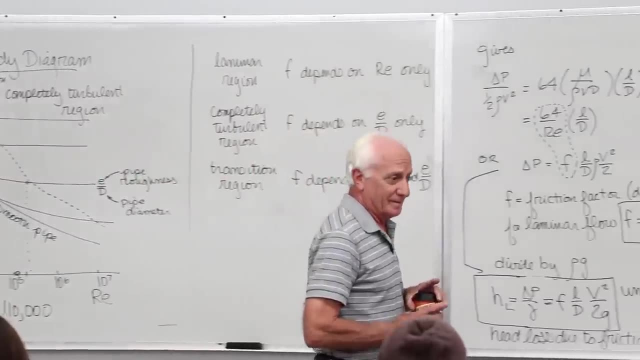 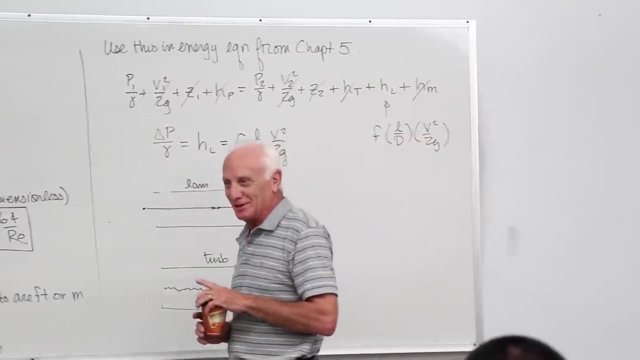 a friction factor in the critical region. well, what if i design something that's in the critical region? i say, well, you should have been an accountant, then maybe a graphic artist, i don't know. but you're not an engineer. no engineer designed something to operate in the critical region. 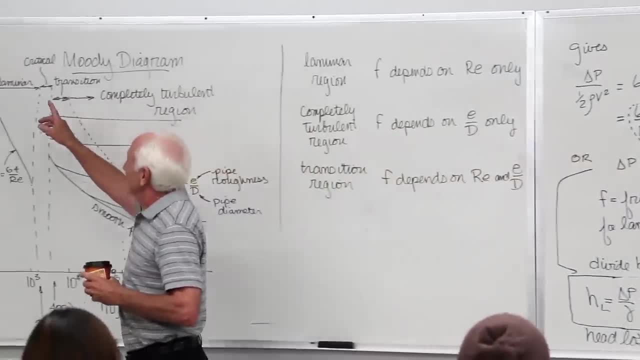 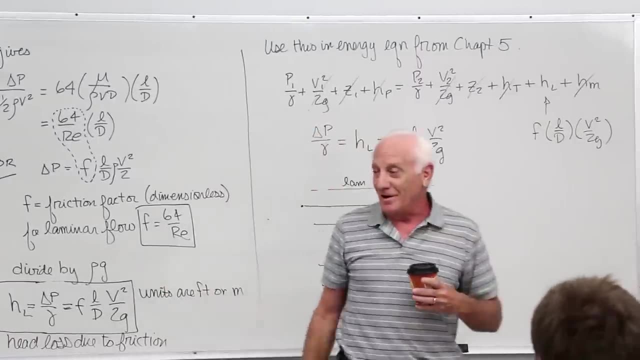 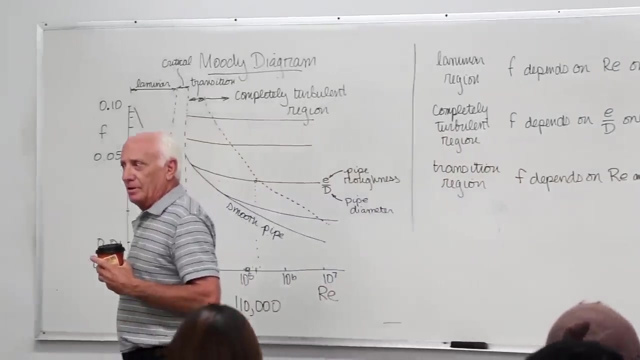 and guess why? because to the left is laminar flow and to the right is turbulent flow, and since we don't know where we are- your neck is on the chopping block- don't say, well, i think it might be laminar, or, you know, i'm pretty sure it's turbulent, but it's pretty sure, i mean, i think me. 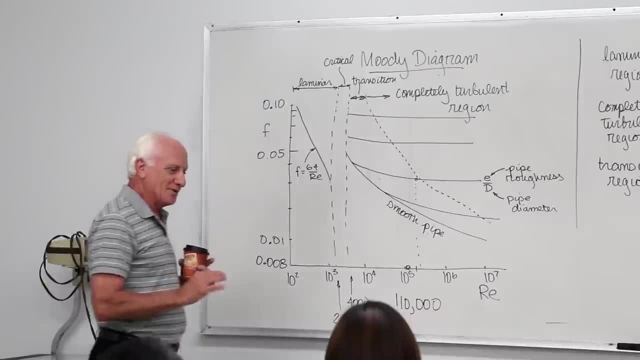 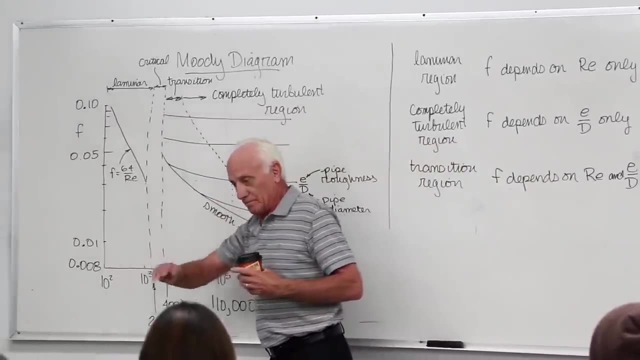 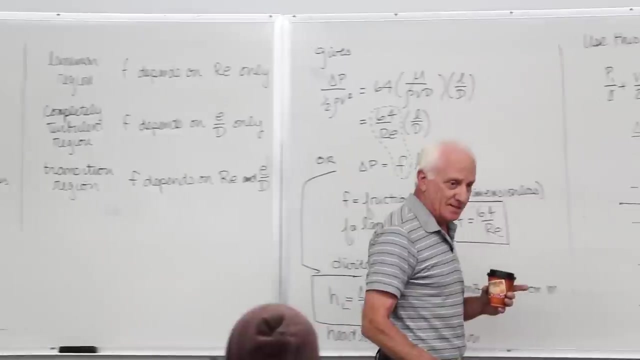 that means you're in trouble. no, it just means we engineers don't design anything to operate in that region. now we know we've got to go past it to get from no flow. when you turn the pump on no flow you're going to return them. we go past it, but we don't sit there on it. we don't design something to sit there. 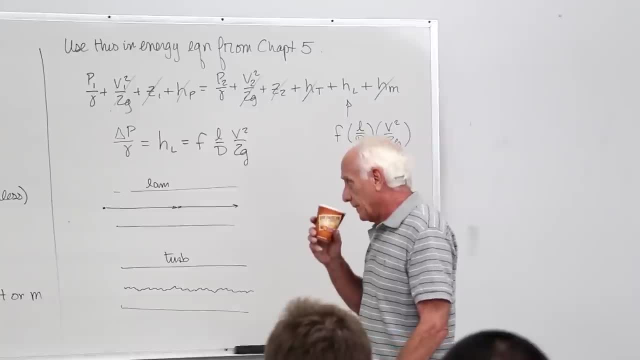 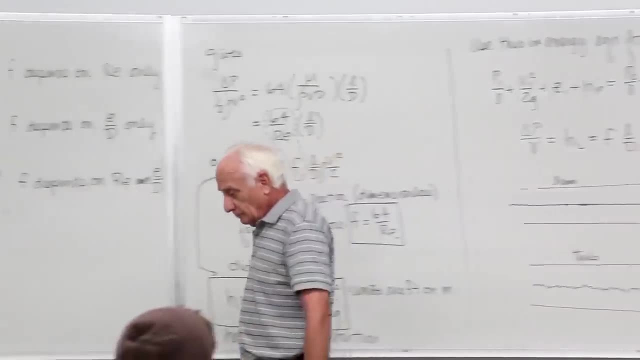 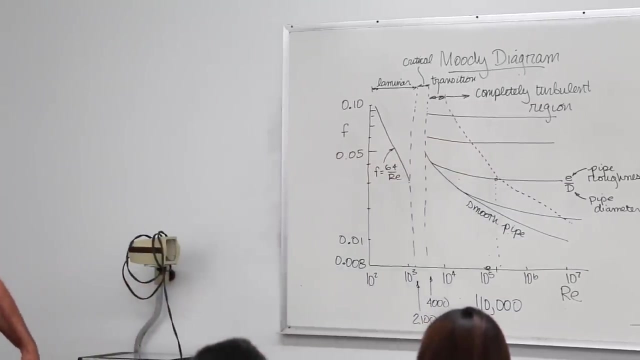 because we don't know what's happening. as a, for instance, the flow could be laminar in a pipe, in a factory, in a plant, in a pipe, and then the pipe protects the four bolts. and over there, 20 feet away, is a big compressor, big compressor. 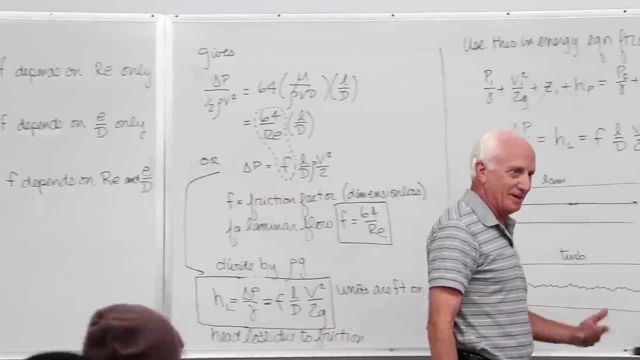 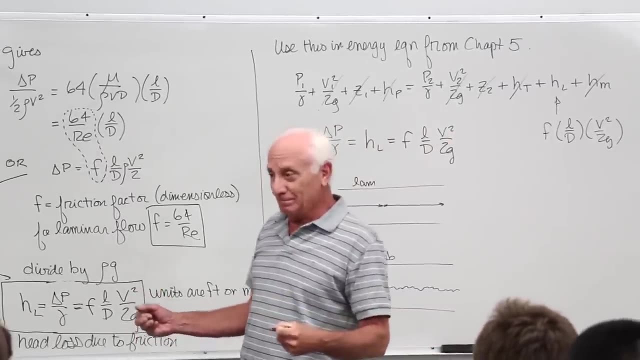 the compressor doesn't operate continuously. it goes on. when the pressure of the air goes down in the line, the compressor kicks on, the floor starts to vibrate. guess what happens? you're running the risk of tripping that laminar flow in the terminal flow just because the compressor went. 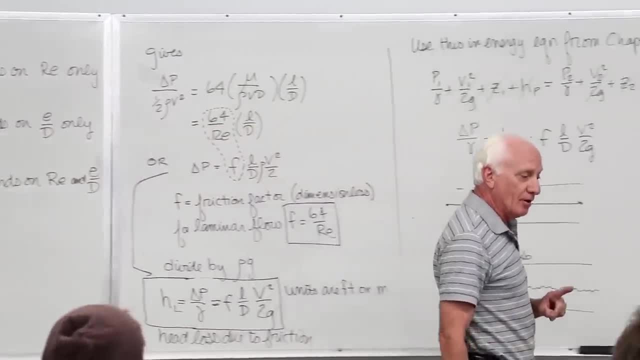 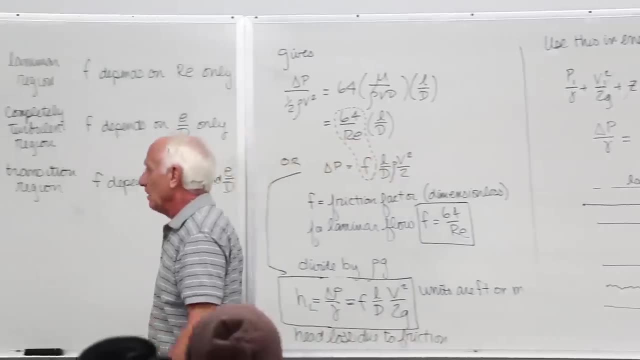 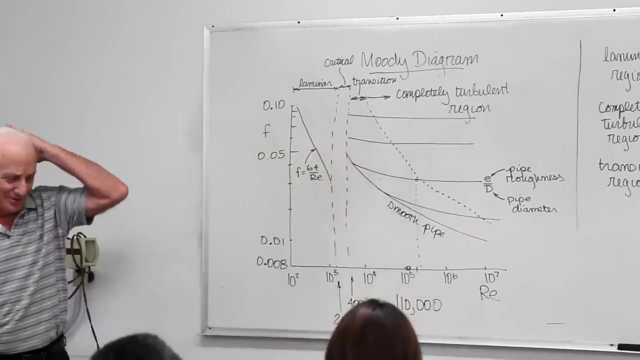 on, which means you, the engineer, don't know what's going to happen. so the lesson is: don't design anything near that region, stay away. say i'm going to make it exactly 2 100.. oh man, you're really, you, really, that's don't. don't do that. that's not a magic. 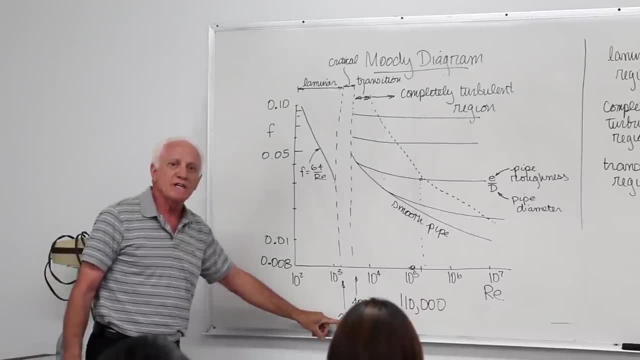 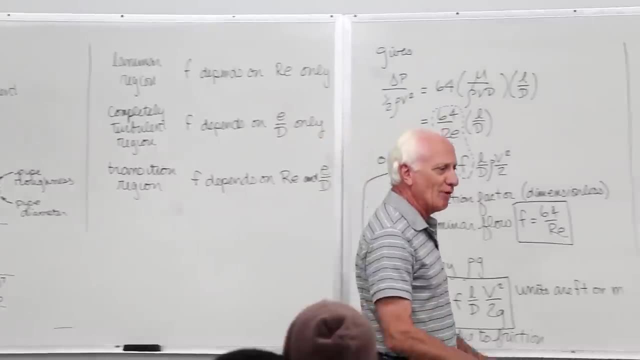 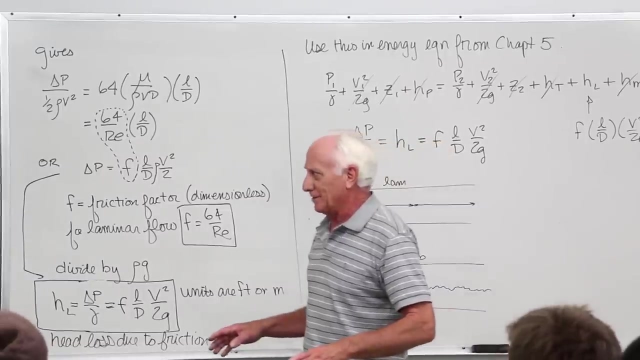 number four textbooks. our heat transfer book says 2300, some textbooks say 2000, some textbooks say 2100.. there's no magic number. it's around 2 100 plus or minus a couple hundred. don't don't think it magically at 2100 it's gonna. it's gonna kick off to. 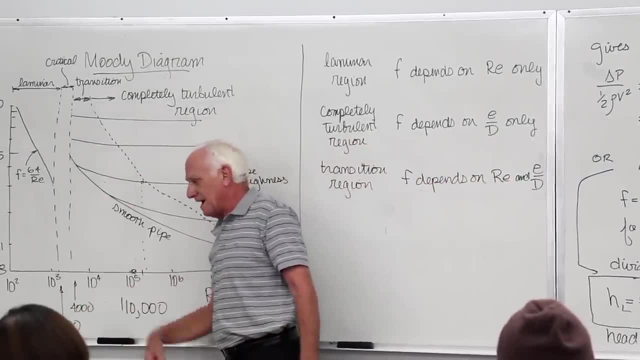 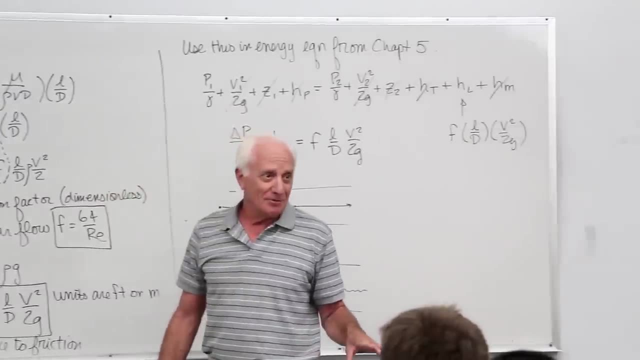 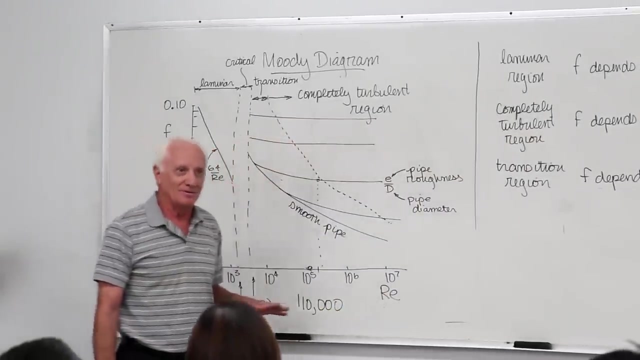 critical: no, no, no, no. all right, four thousand magic- no, it's not magic. now here's the rule book in our class: yes, magic number, if you get it on an exam, twenty, two thousand and fifty, okay, it's lambda flow. you get four thousand and one, it's turbulent flow. so in our class, the other magic numbers in the real. 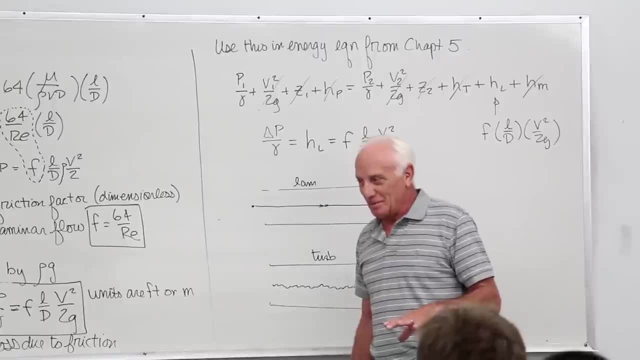 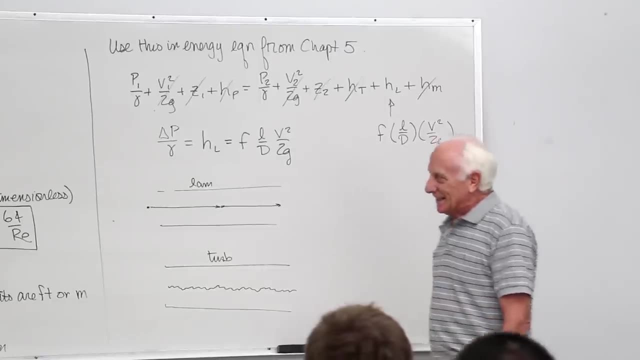 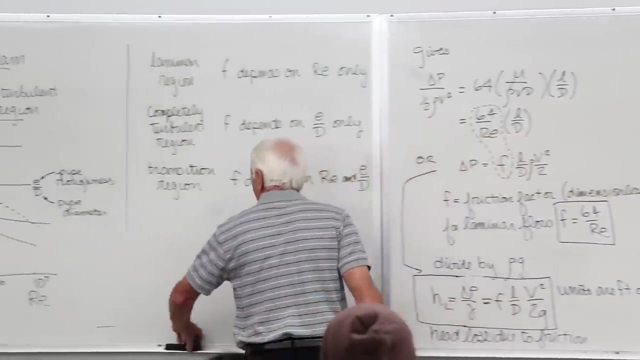 world. no, they're not magic, they're negotiable. where's your pipe? inside the plant? outside the plant, how close is it to it? to a diesel engine? blah, blah, blah, things like that. okay, now let's see, that's so. that's our turbulent here's. if it depends on now, there are various fit equations to fit. 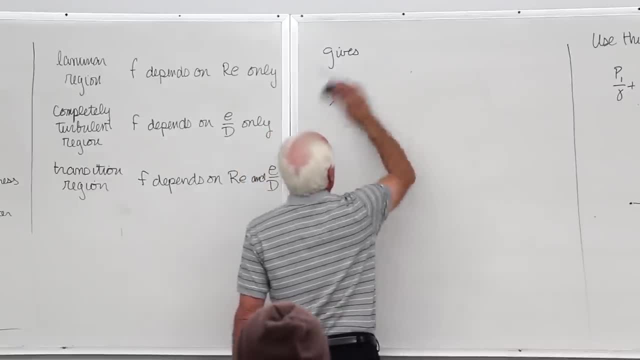 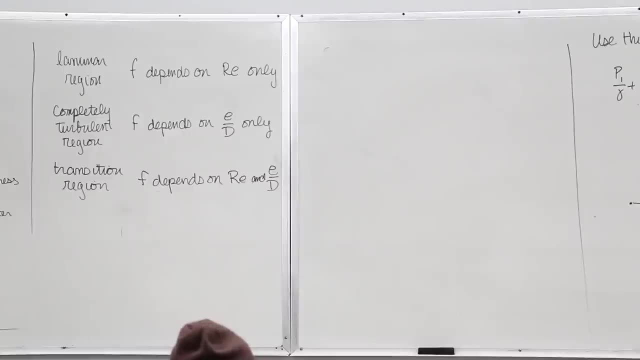 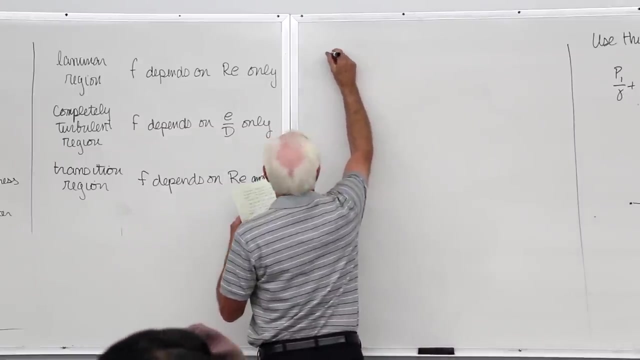 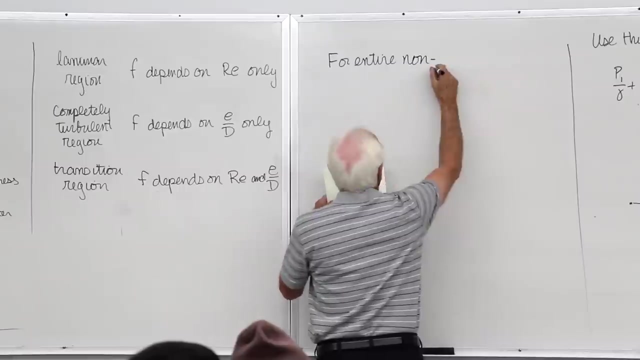 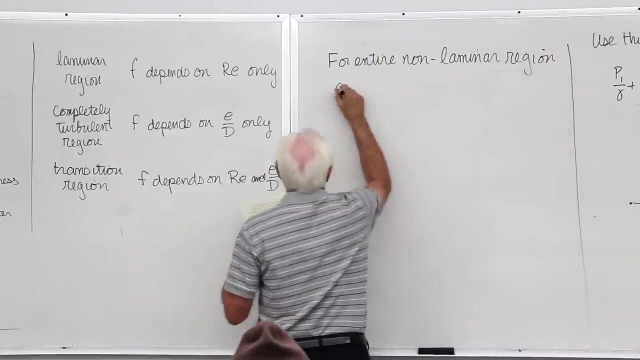 that data. some are more accurate than others. we're going to use one. you can use one equation that fits that data and it's called a modified Colburn equation. so this is for our entire nonlinear and non-laminar. you can use the Colbert formula. it's called a modified Colbert. 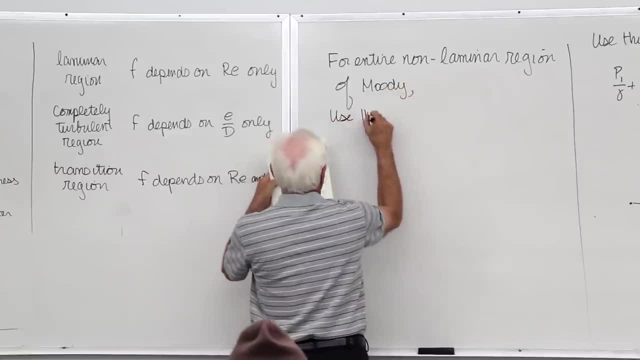 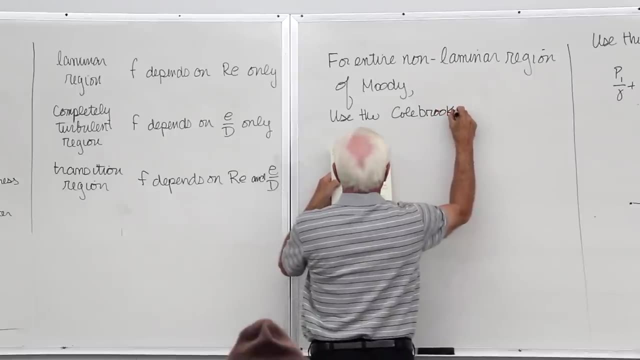 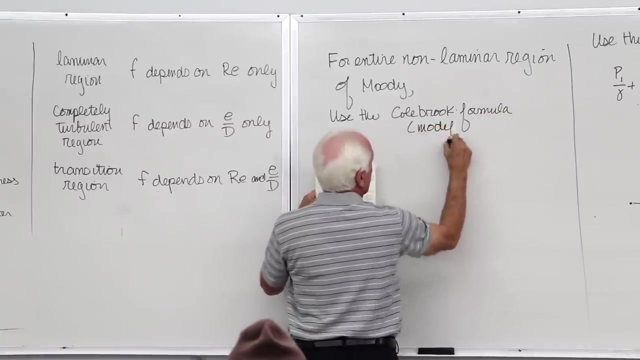 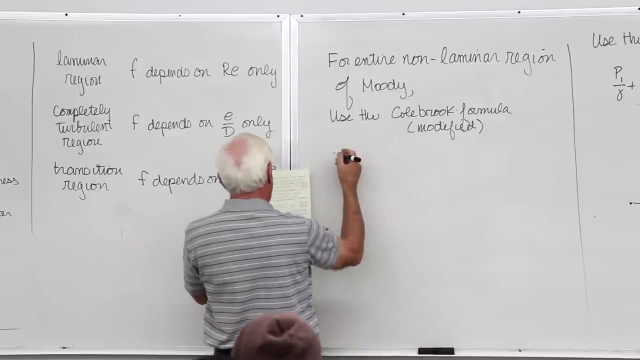 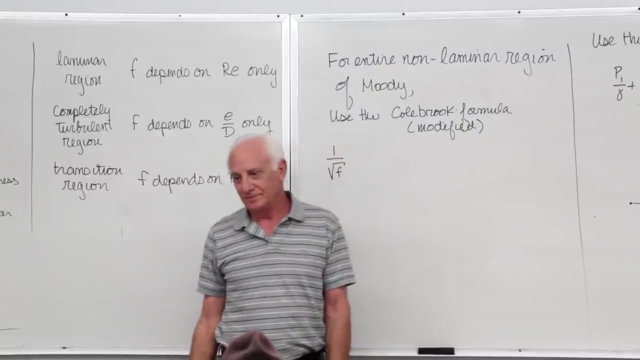 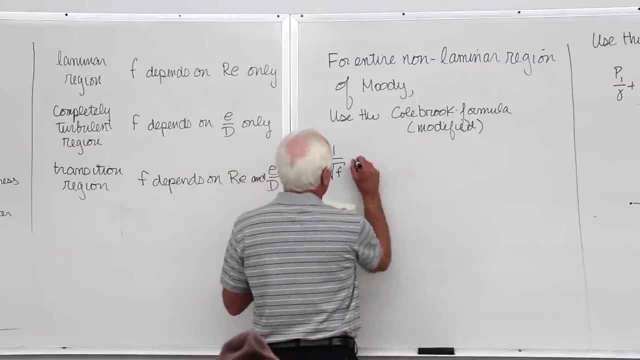 you can use the Colbert formula. it's called a modified Colbert, you sometimes call a halen equation but we'll call the modified Colbert 1 over square root F, because you can't put the moody chart on some kind of a computer code. obviously you got a pretty equation minus 1.8 log to the base 10 d over d 3.7. 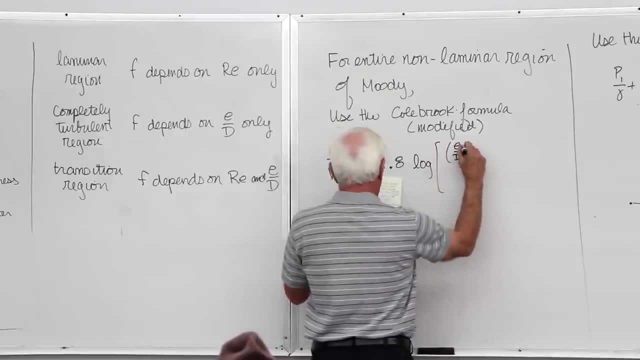 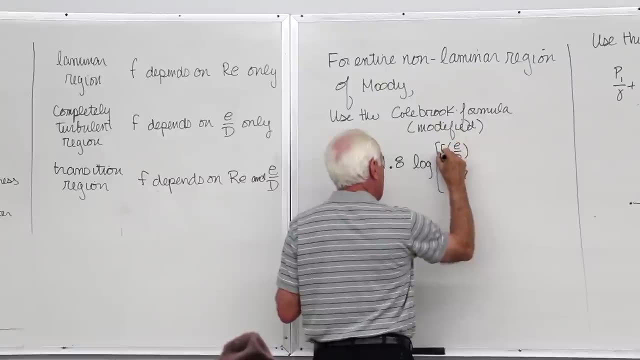 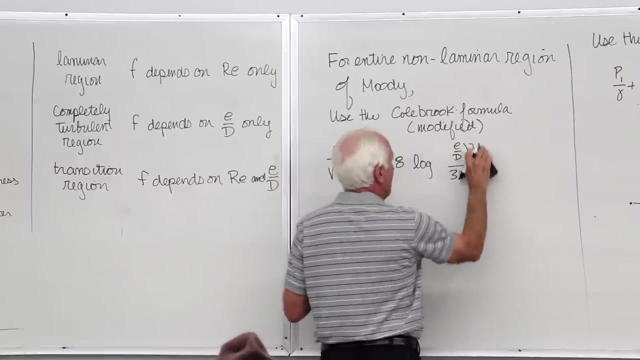 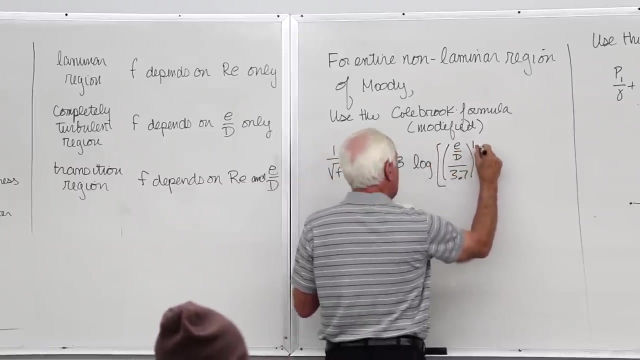 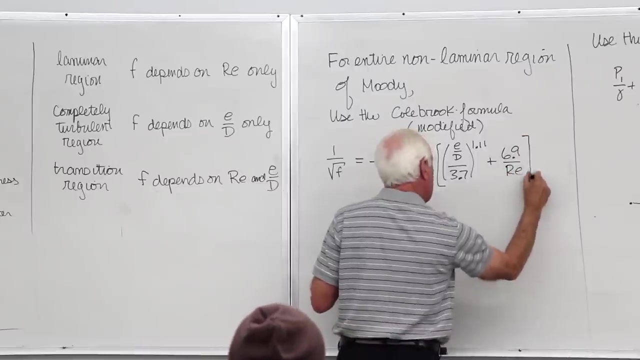 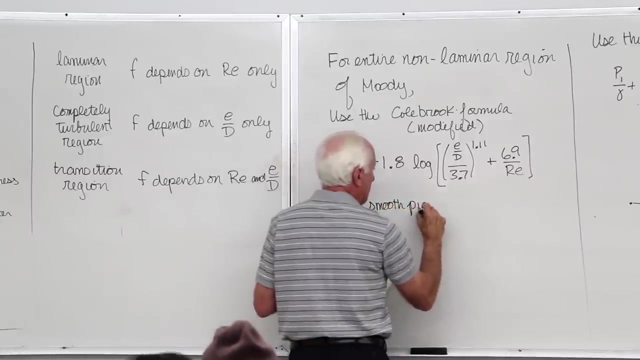 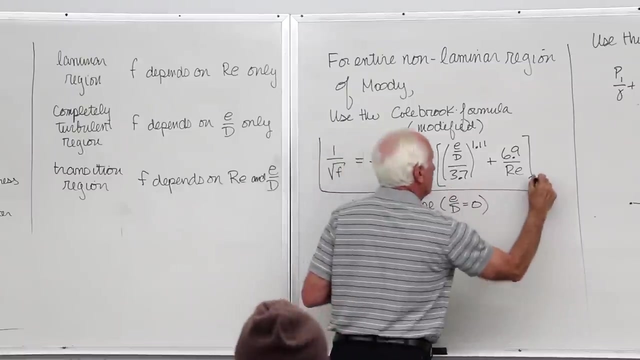 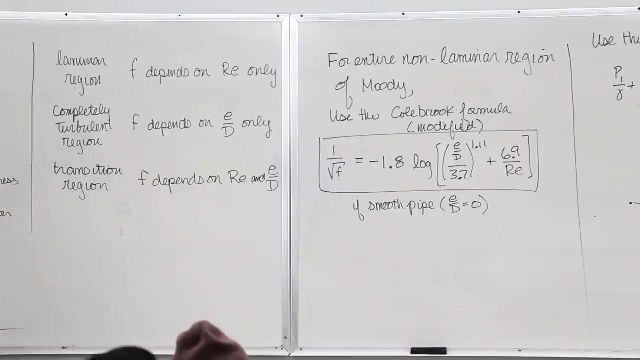 minus 1.8 log to the base 10 d over d 3.7. minus 1.8 log to the base 10 d over d 3.7. Let's just make it similar, So you can't use this to calculate F. 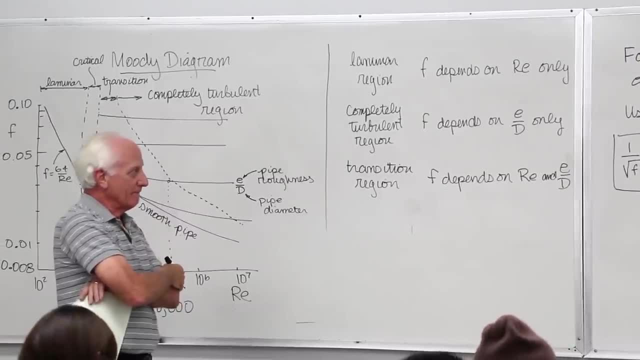 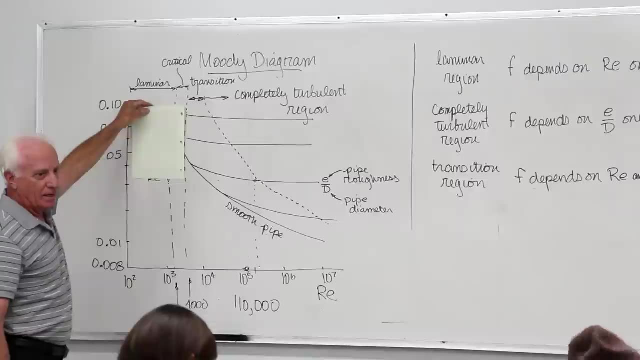 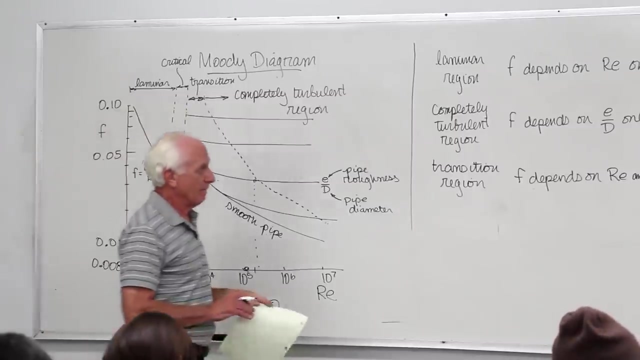 It's going to take some calculation, obviously, And that works anywhere to the point of the right of my piece of paper, Anywhere to the right of my piece of paper. If E over D is a smooth pipe, then of course the roughness is zero in there. 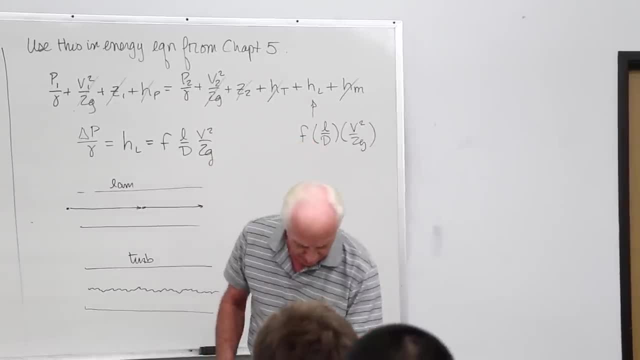 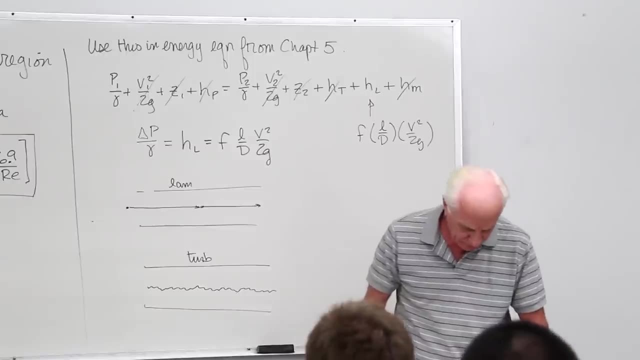 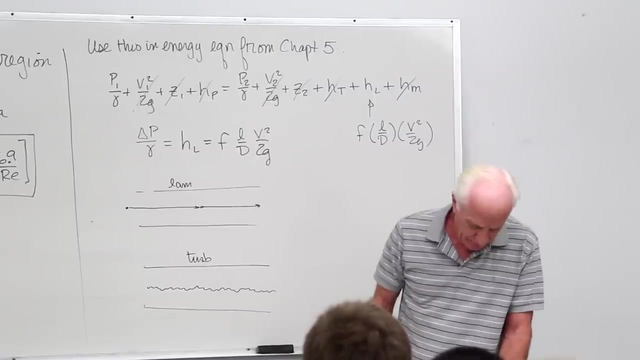 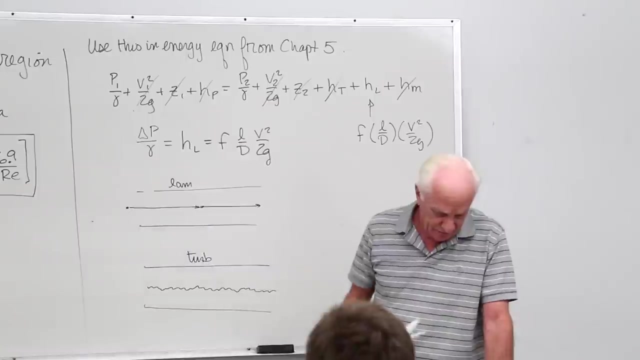 Okay, Oh, and our textbook tells you about. well, I'll read it here. Okay, A word of caution is in order concerning the use of the Moody chart or the equivalent formulas, Because of various inherent inaccuracies involved: Uncertainty in relative roughness. 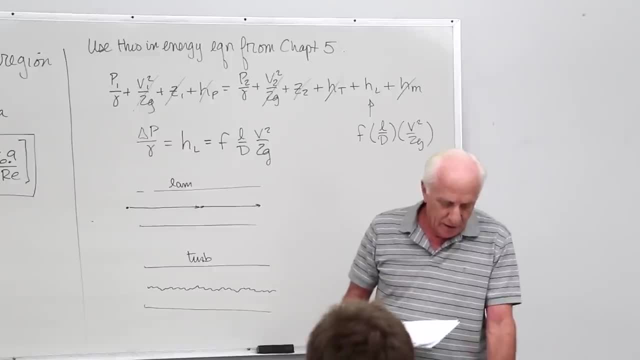 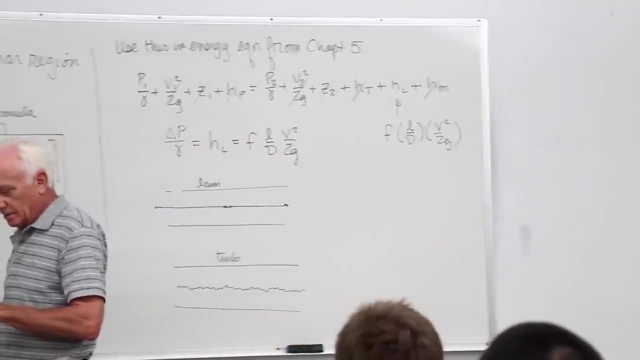 Uncertainty in experimental data to produce a new pipe. The use of several place accuracy in pipe flow problems is usually not justified. As a rule of thumb, a 10% accuracy is the best expected. That's the best. So it goes downhill from there. 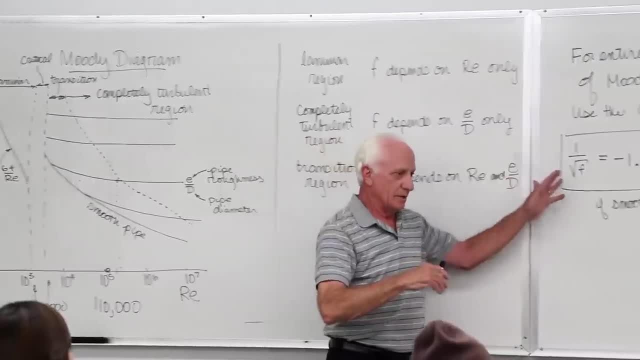 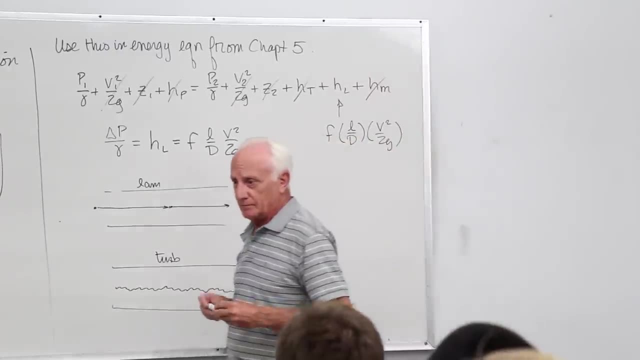 So the best you can get by reading the Moody chart or using the equation is within 10% of the actual one, And of course that's only for a brand new pipe If the pipe's been in the line for five years. 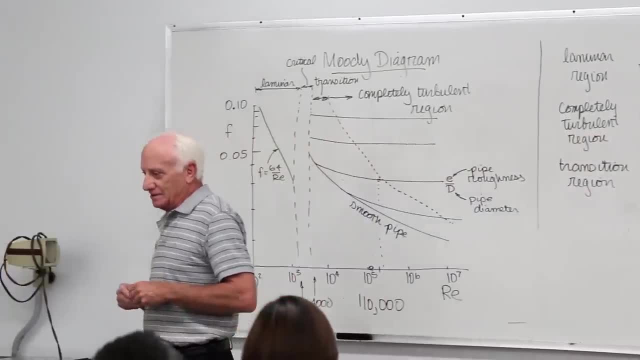 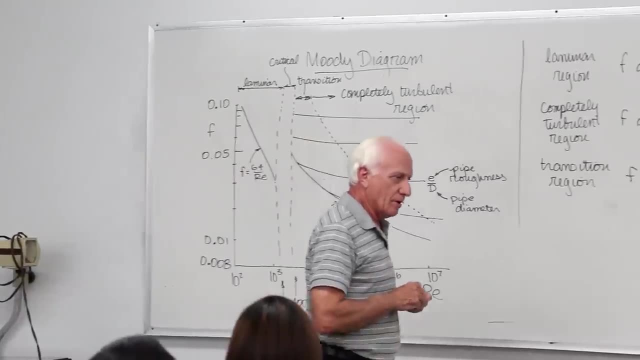 all bets are off. The roughness has increased dramatically because of hard water deposits on the inside of the pipe, For instance, your pipes in your home. Hard water in the western region of the US, Oh yeah, And what does that do? 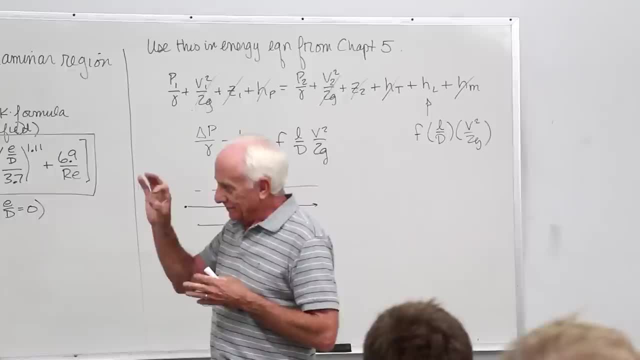 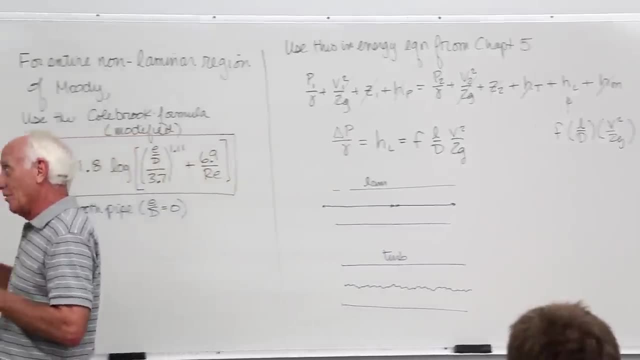 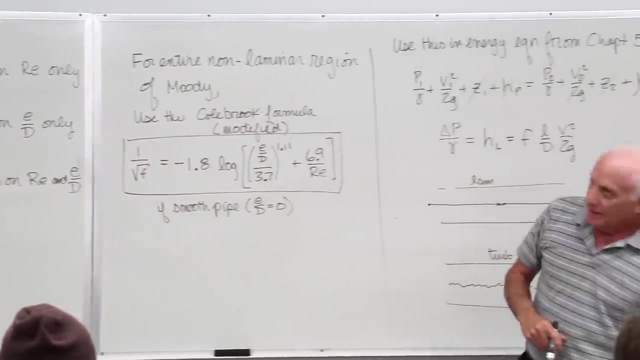 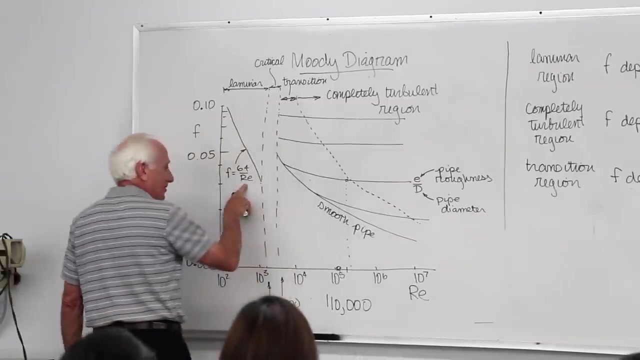 Deposits. calcium makes the surface really rough and it makes the opening smaller and smaller with time as you get more and more calcium. So yeah, that's a big, big problem. This is only for designing new pipes. Okay, Now look at the friction factor for laminar load. 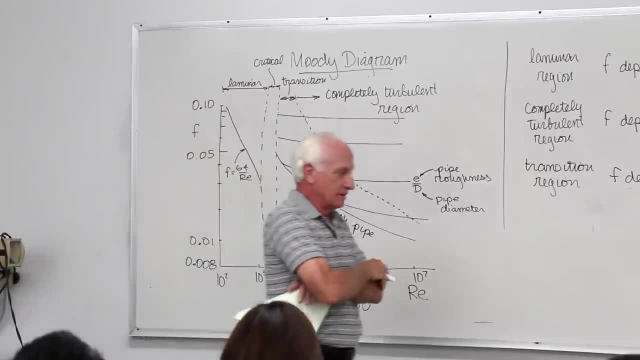 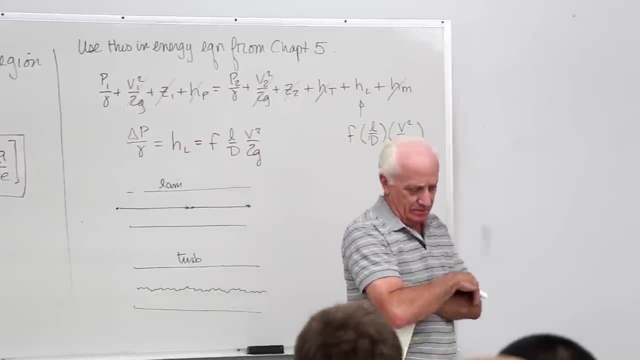 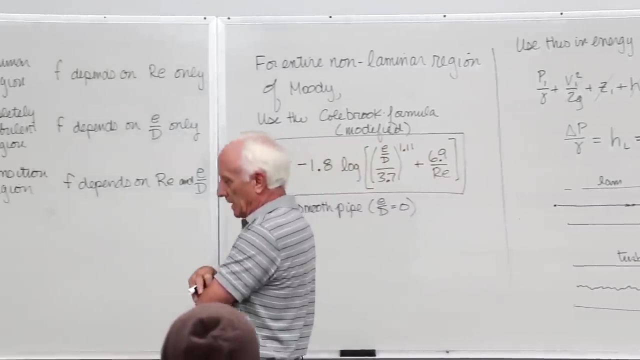 Is that equation valid for oil? Of course it is. Water, Yeah. Air. Mm-hmm. Carbon dioxide- Yeah. A one-inch pipe, Yeah. Six-inch pipe, Yeah. Rectangular duct, HVAC duct, Uh-huh. 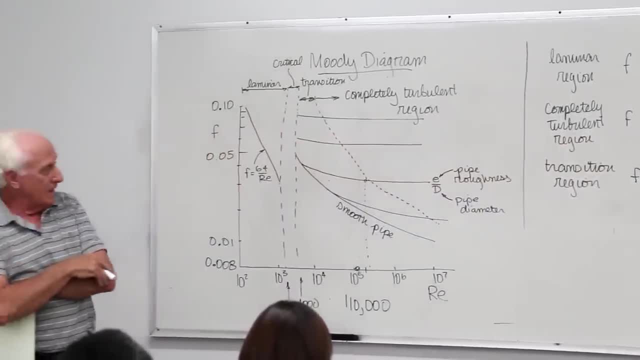 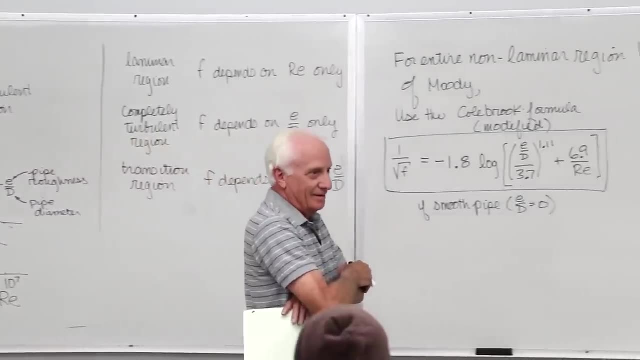 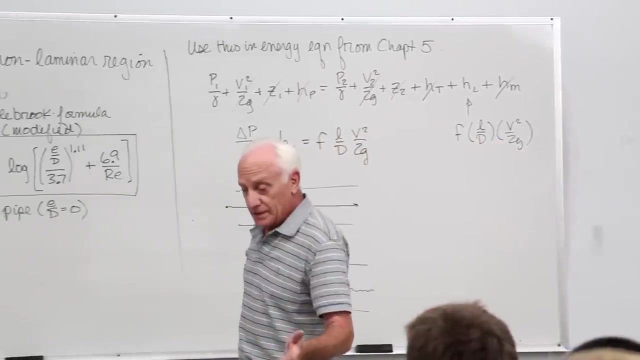 30-foot water pipe? Yeah, Okay, Is it valid for PVC? Yeah, Is it valid for cast iron? Uh-huh Concrete? Yeah, You get the point. There's not a special equation for different diameters or different flow rates. 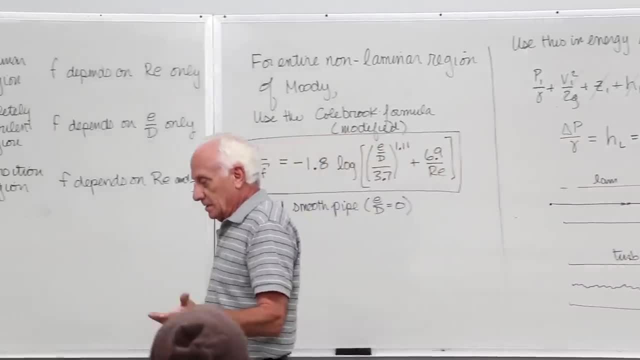 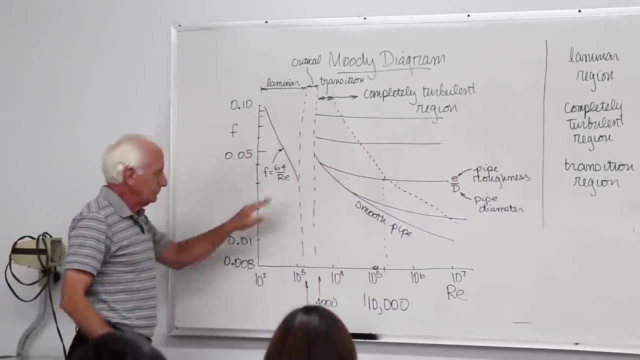 Flow rate: two gallons per minute, 10 gallons per minute, 30 gallons per minute. Does it work for all that? Yeah, it works for all that, No matter what the pipe's made out of. Well, you know, here's the Reynolds number. 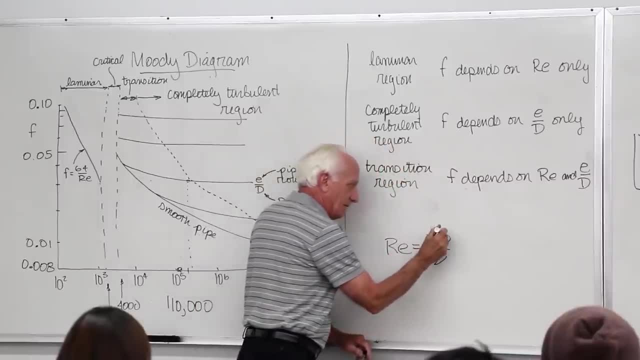 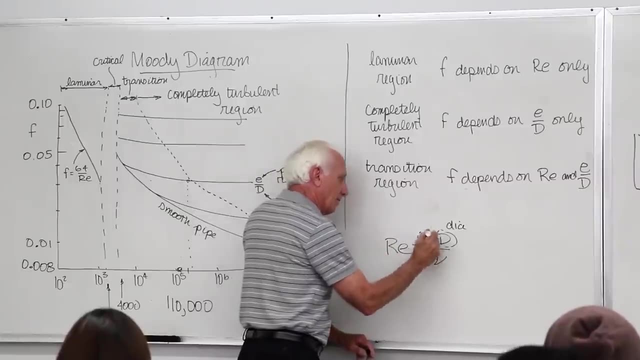 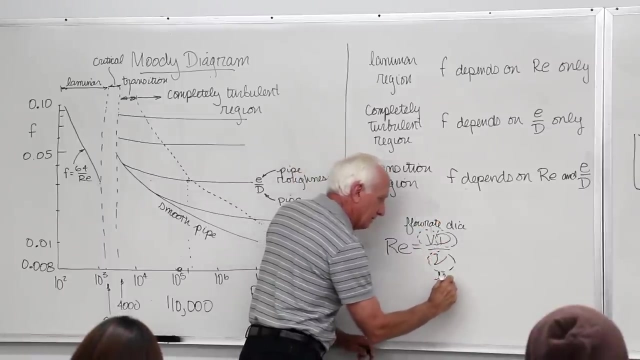 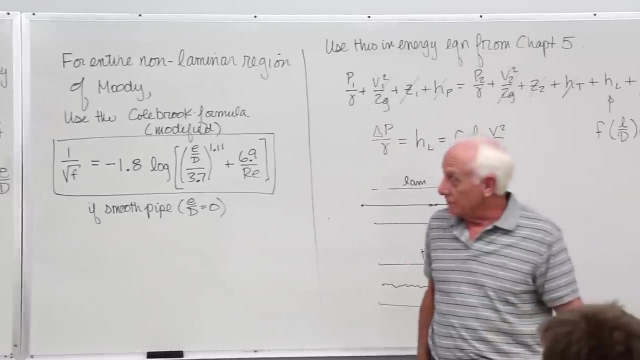 Here's what the Reynolds number is. First of all, it's a function of the pipe diameter. Second of all, it's a function of the flow rate. Third of all, it's a function of what the fluid is. Those are the three things that the friction factor. 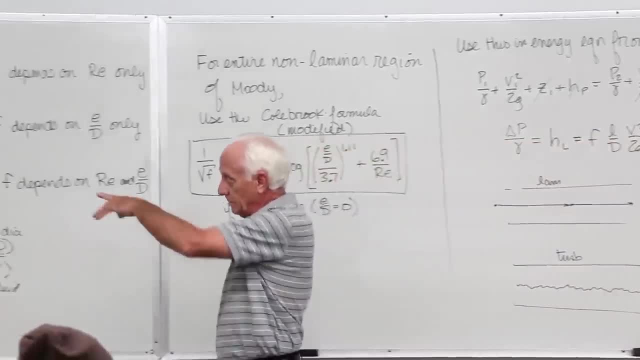 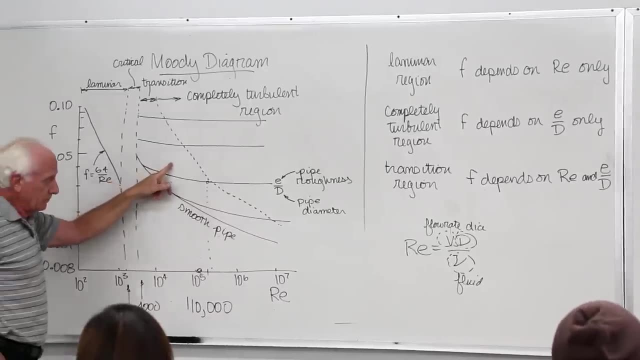 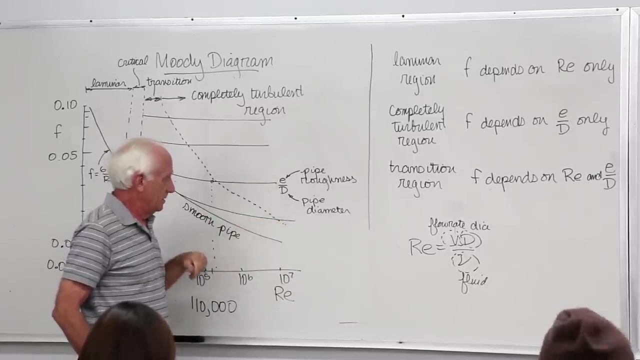 the Reynolds number depends on. So there's only one equation for everything. Now you go to turbulent flow. Now I add one more parameter, this dimensionless thing, E over D, to that one. So now you tell me what kind of pipe it is. 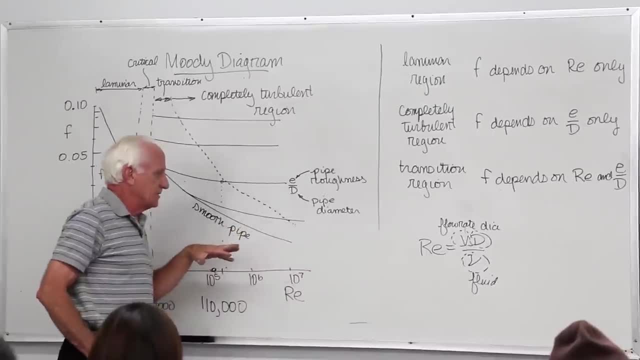 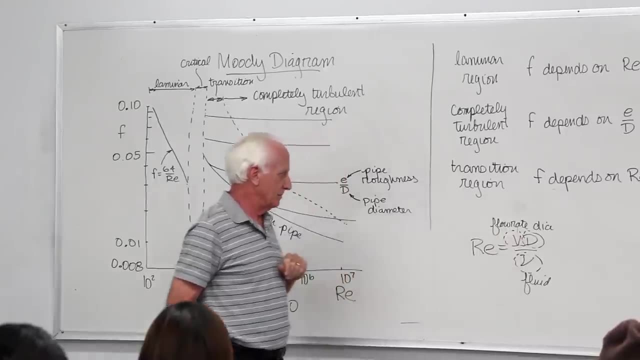 Stainless steel. Okay, I get E over D. Tell me its flow rate: 100 gallons per minute. Okay, I got V. now Two-inch pipe, Got it. What's it carrying Water? Got it. So I know everything I need. 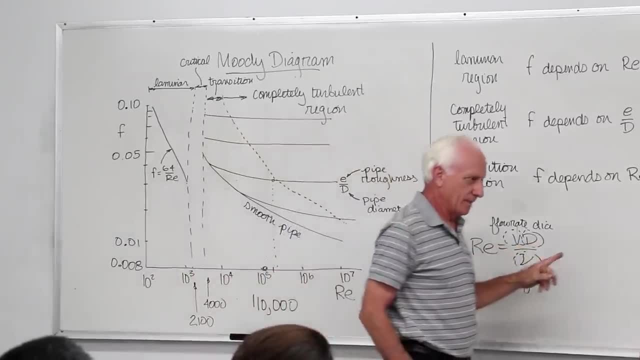 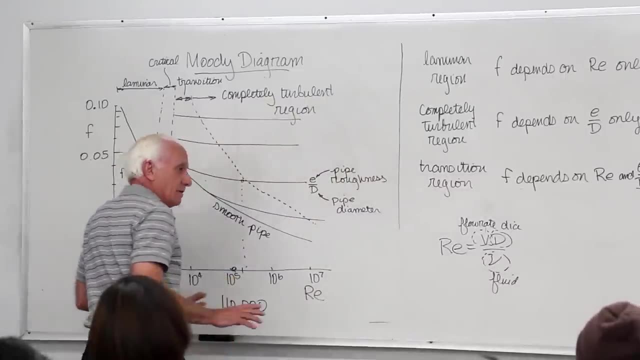 What kind of pipe it is, What's its diameter, What's the flow rate, What's the fluid. Based on that, I can go over here and I can find the friction factor. Now you know what's the flow rate. 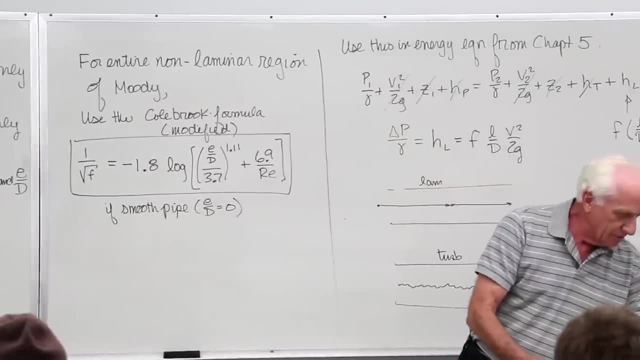 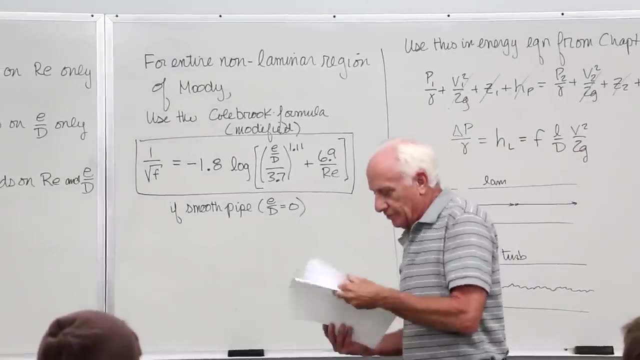 Is there 10,000 sheets of paper? Let's see, I'm trying to find stainless steel. Oh, here it is. Now I'm trying to find stainless steel two-inch diameter. Oh, there's a movie chart for that too. 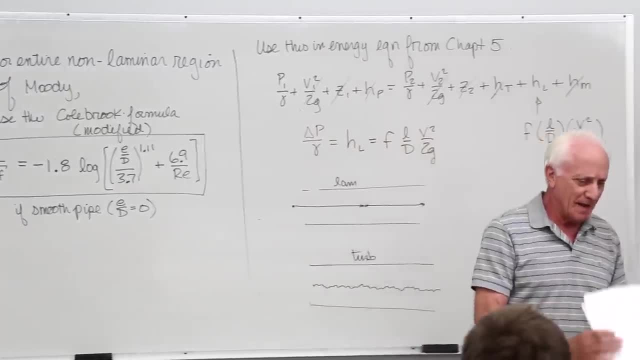 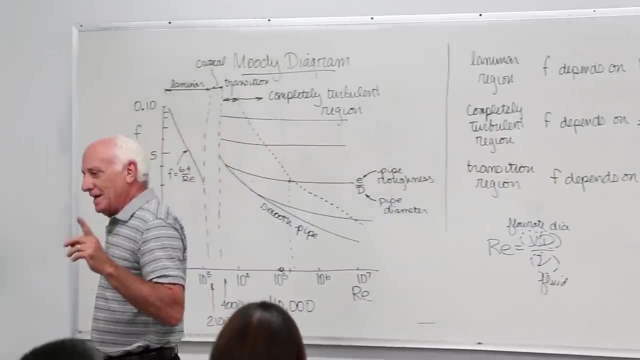 There, right there. No, there's not 10,000 sheets of paper, one for each fluid, one for each diameter, one for each flow rate. No, no, no, no. Guess how many sheets of paper I need to give you the friction factor. 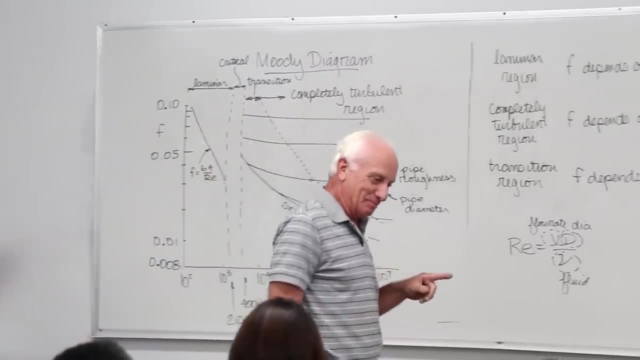 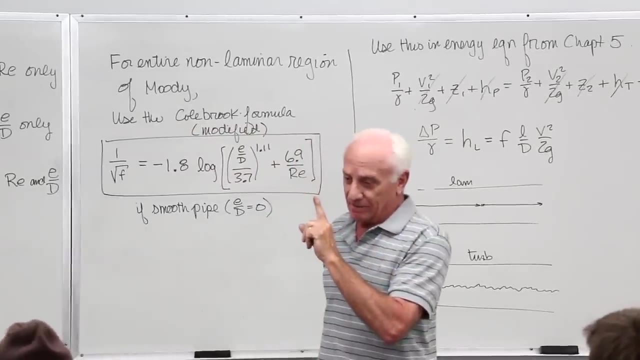 For any pipe material, any pipe flow rate, any fluid in the pipe. I'll tell you One: I wish I'd invented the little diagram. I love the sound of that. No, I'm sorry I didn't do it. 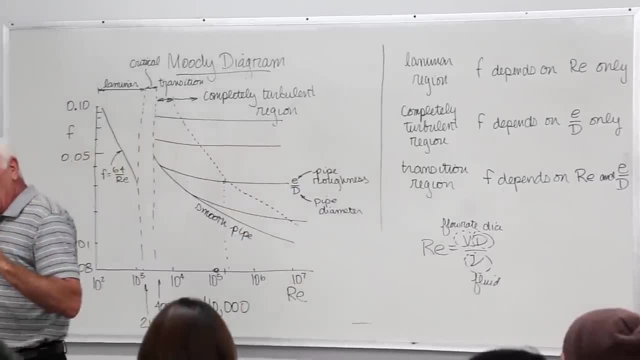 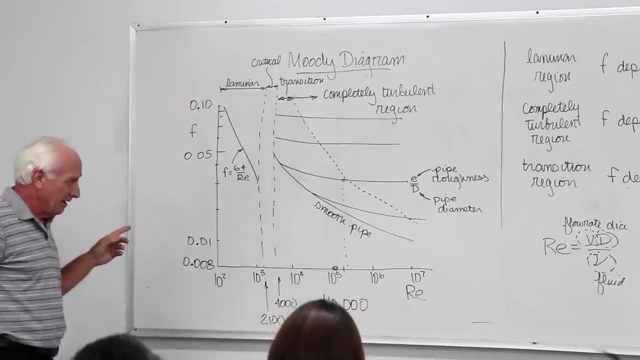 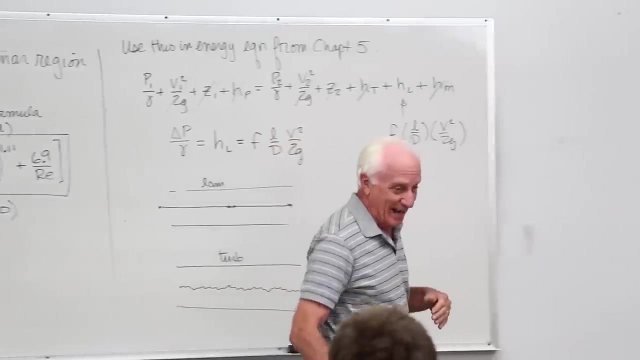 Professor Moody did that back then. So yeah, Now people don't realize that. Are you kidding me? One sheet of paper, The friction factor for everything that engineers can imagine. That's why everybody graduating from a fluid class better know the Moody diagram. 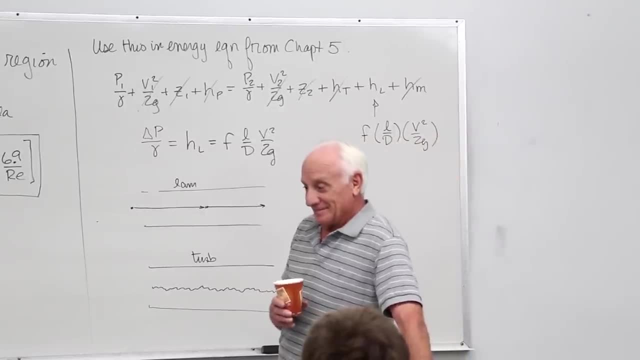 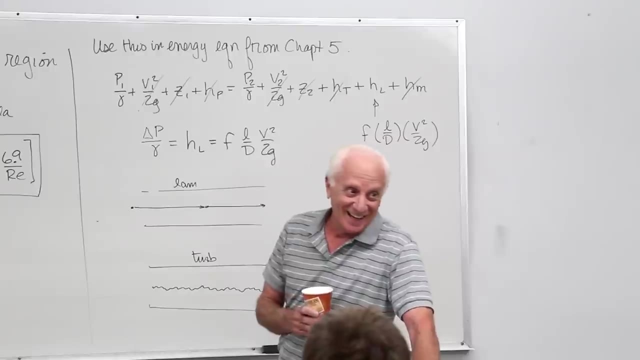 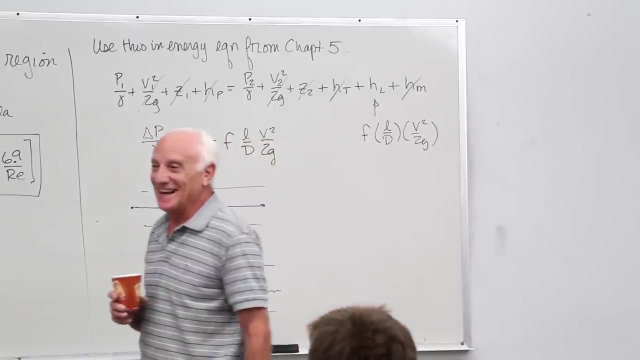 Everybody graduating from an ME 218, street materials. what should they know about a certain diagram, The what? What's the one with the circle? You got it. You got it. Are there equations to do that? Are there equations to do that? 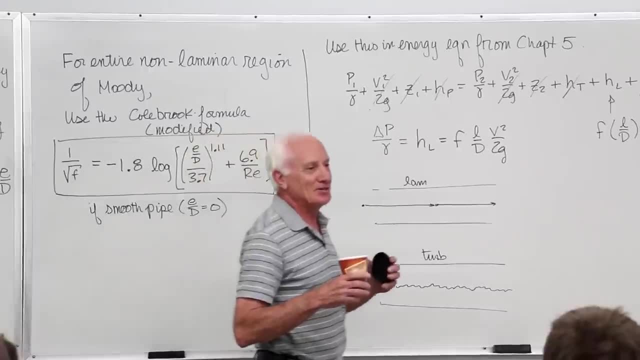 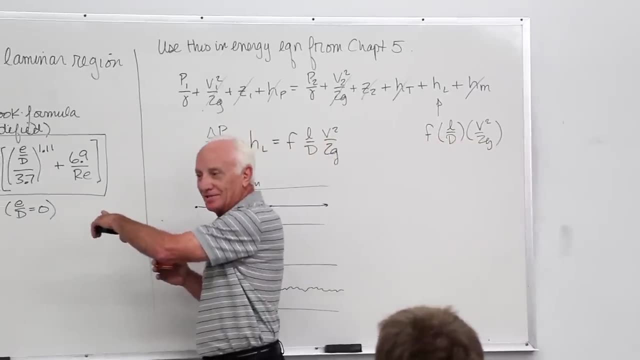 Yes, there are. Why do we still teach them over a circle, then? Because we engineers love the visual impact of a diagram like that, And why don't we just use the equations? Because the equation came from that. So, number one, you should learn how to read this. 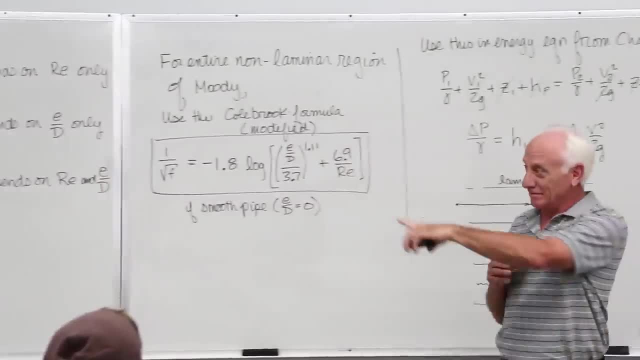 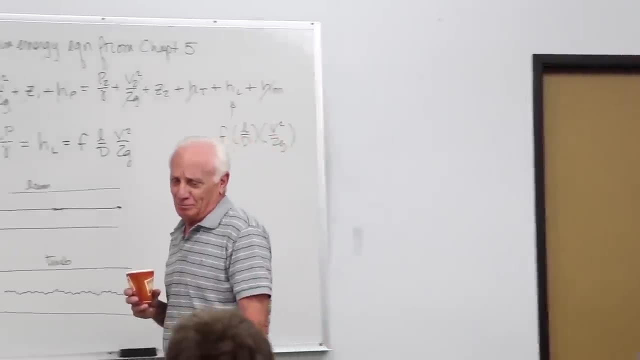 And this is just then what you put on your computer program to solve for that diagram. Oh, isn't that beautiful. I just love that diagram. You know, Here we are. We're that kind of people. Now, the math people say: 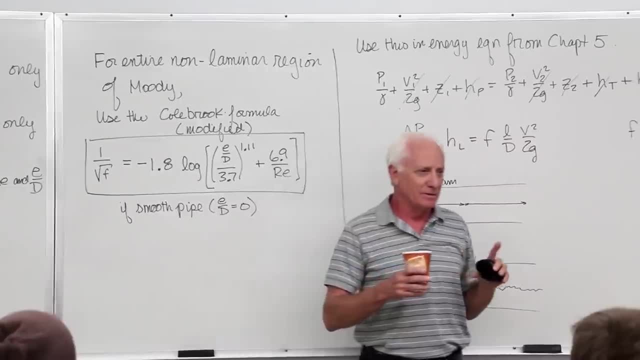 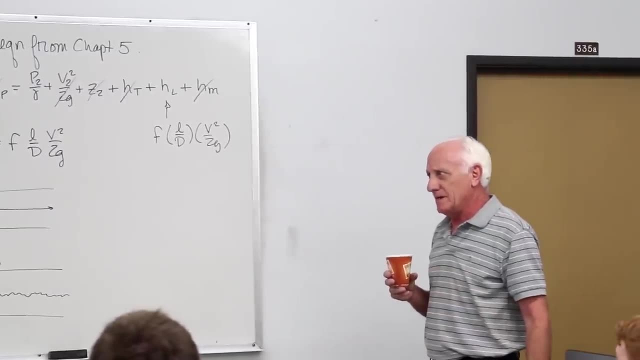 oh, look at that equation. I love that equation. I know I love them too. They're good people, But they're not engineers. okay, We love other things later. That's why I love that Moody diagram. Everything is on that thing. 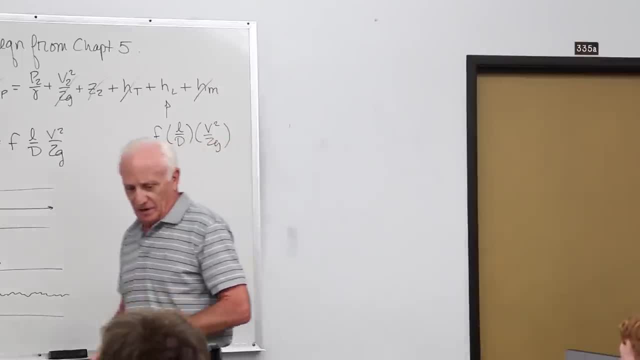 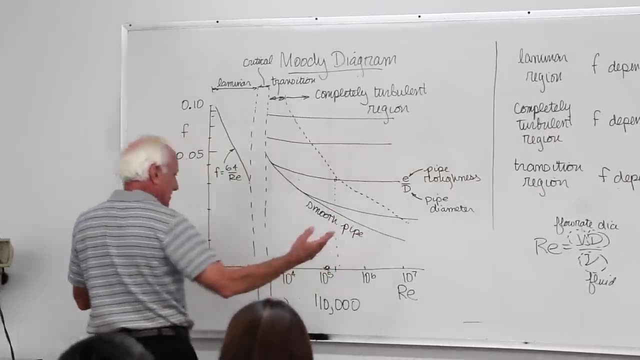 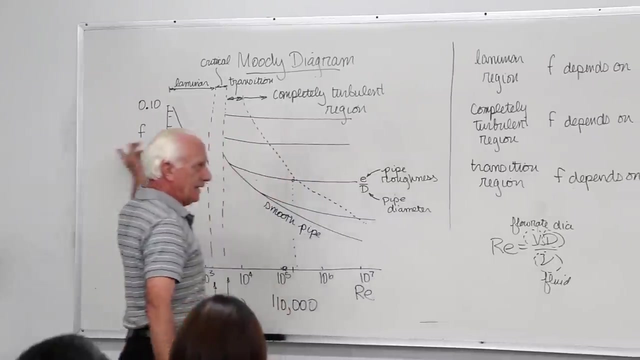 And what kind of diagram is that? That's called a dimensionless diagram. We engineers love dimensionless numbers. You don't plot the flow right here, the velocity. You don't plot the timer. It's all divided by different things here and here. 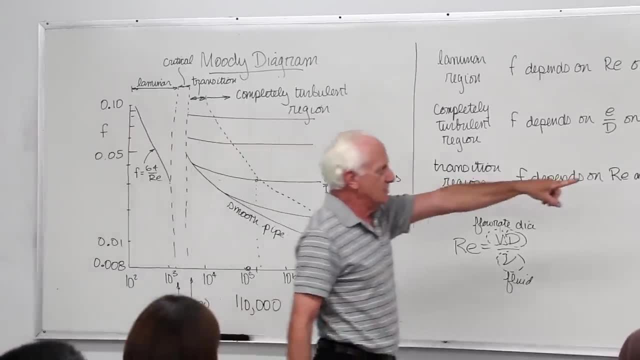 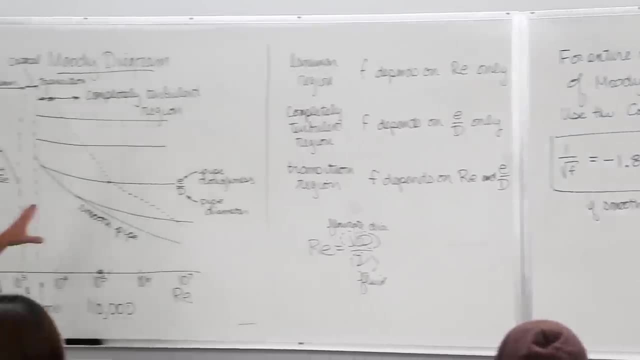 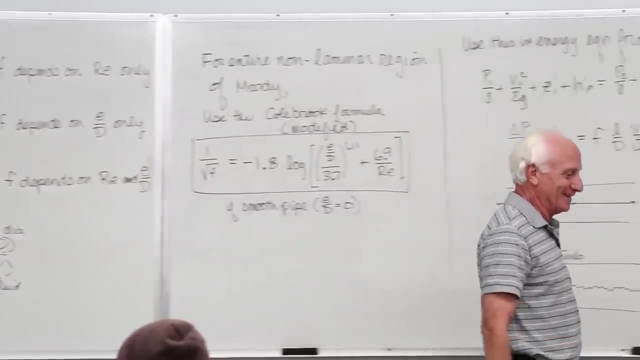 And F dimensionless. That equation right, there is a dimensionless equation. Nothing has dimensions. Okay, So that's the diagram that you want to use to get the friction factors for homework and other problems. You'll have one on the final exam. 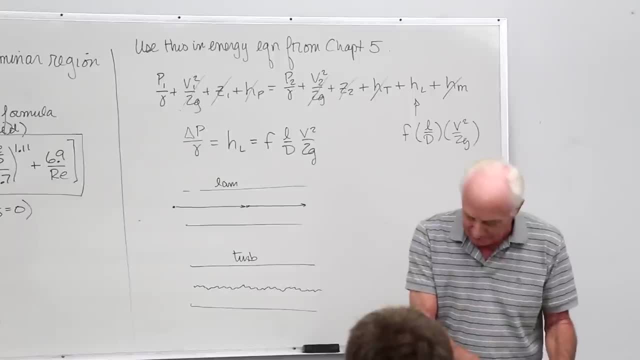 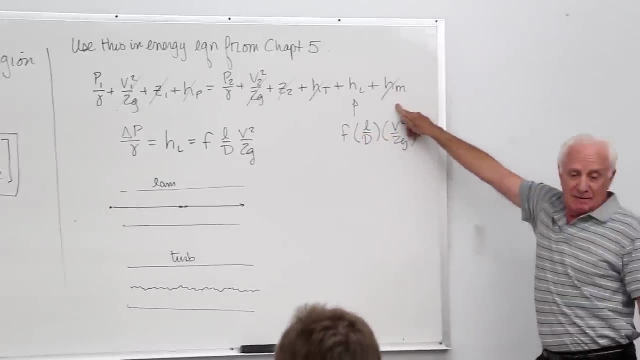 So you'll have that in your hands for that. Okay, Good stopping point. Now. next time we're going to bring in Here it is We're going to bring in the guide. Next time we're going to discuss the minor losses.